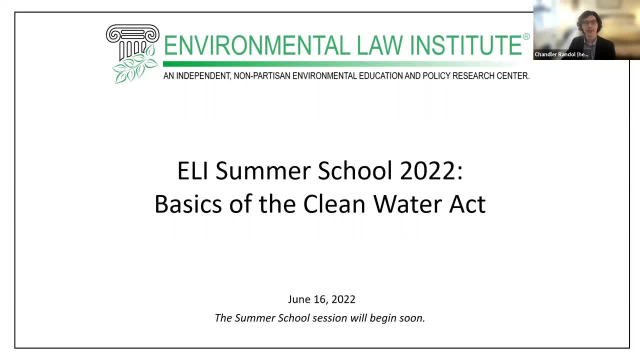 At the end of today's webinar, we will have time for a Q&A session, so please submit your questions through GoTo's question box and please do not wait until the end. Please send us your questions as soon as you think of them. I would like to thank our outstanding panelists for joining us. 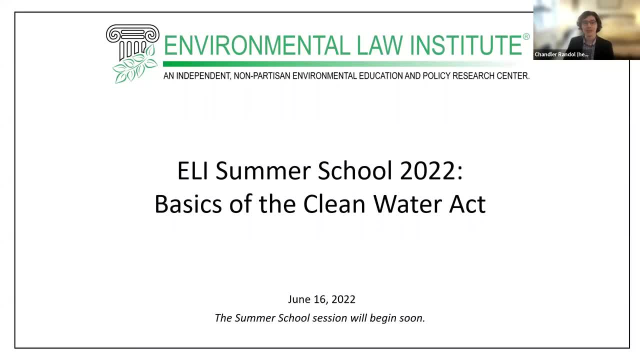 today to lend their expertise to this webinar and, while they will be introduced briefly, the full speaker bios are posted on our website, eliorg, and I strongly encourage you to check out their expertise and experience In more detail there. as we begin, I would like to very briefly introduce today's moderator, Adam. 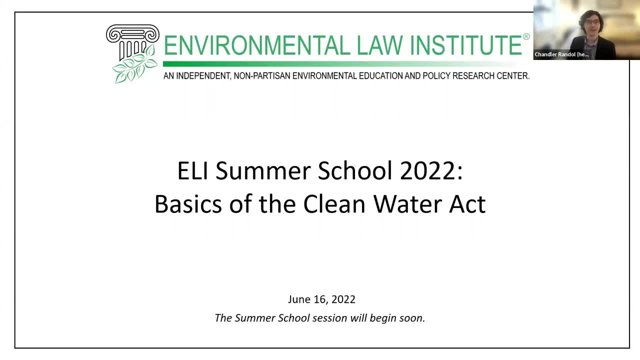 Shipp Adam is a Senior Attorney and Director of the Western Water Program at the Environmental Law Institute. Much of his research focuses on water resource management, specifically identifying opportunities to meet conservation and sustainability objectives through existing laws and potential legal developments. He leads ELI's work on water allocation and use in the US. 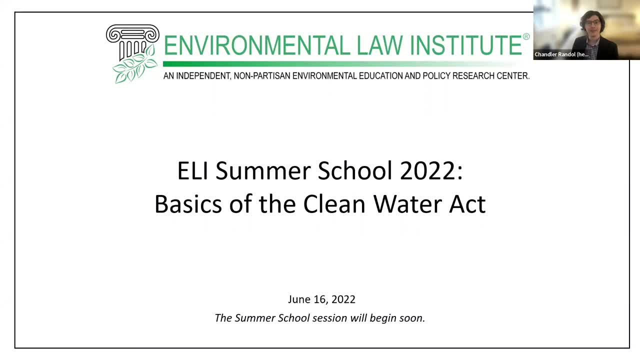 Adam also has worked extensively on other topics, such as water management and water management. He has worked extensively on other topics, including TMDLs and the Clean Water Act. 303D listing marine spatial planning and ecosystem based management of marine resources and routine program challenges under the Coastal Zone Management Act. Adam, we are so thrilled to have you here with. 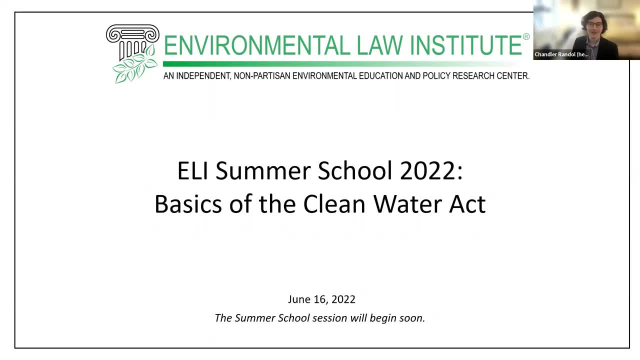 us today. With that, I will turn things over to our amazing moderator, Adam Shipp. Thank you all so much. Great the introduction, Chandler. Thank you very much. Hello, welcome everyone to this week's summer school course. We are very privileged to have 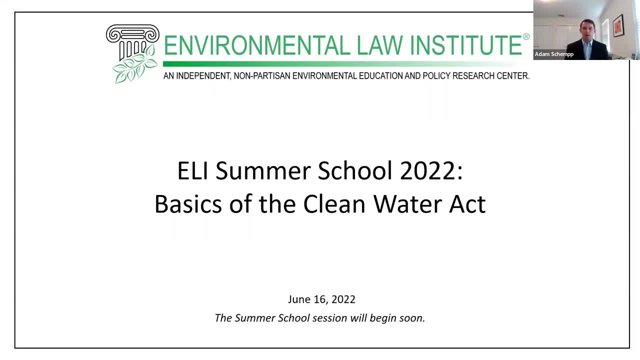 three distinguished attorneys walking us through various aspects of the Clean Water Act, starting with a broad overview before detailing some of the more hot button issues of late. Specifically, Robin Rotman will recount the history of the water quality regulation in the US, provide a quick summary of the various aspects of the Clean Water Act and then briefly touch on some. 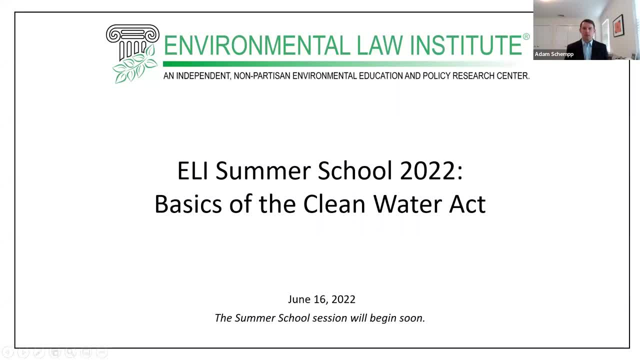 current issues. Jonathan Genzier will then explain the history of the current state of affairs. history and current state of affairs regarding waters of the US, which is effectively the applicable jurisdiction of the Clean Water Act. He will then explain the history of the current state of affairs regarding waters of the US, which is effectively the applicable jurisdiction of the Clean Water Act. 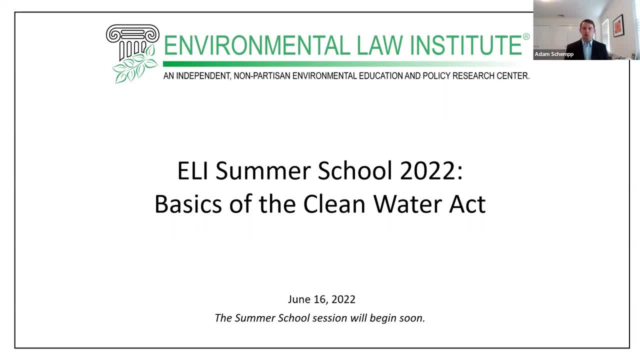 He will then explain the history of the current state of affairs regarding waters of the US, which is effectively the applicable jurisdiction of the Clean Water Act, And then talk about the new section 401 rule, which concerns the review authorities of states and tribes relative to certain federal actions. 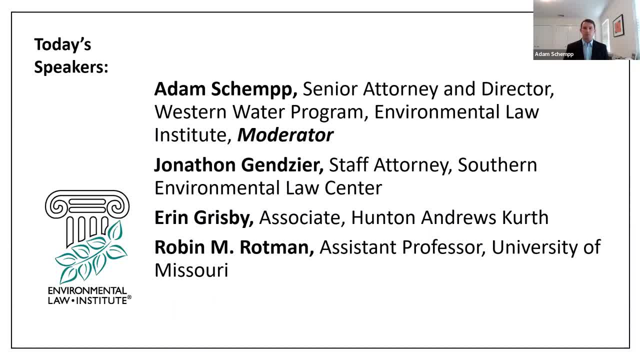 And last but not least, Aaron Grisby will cover aspects of point and nonpoint source pollution, including the Maui decision, before explaining some of the basics of total maximum daily loads, or TMDLs. The session is going to conclude with a Q&A period and hopefully we will have plenty of time to address any questions that you may have. 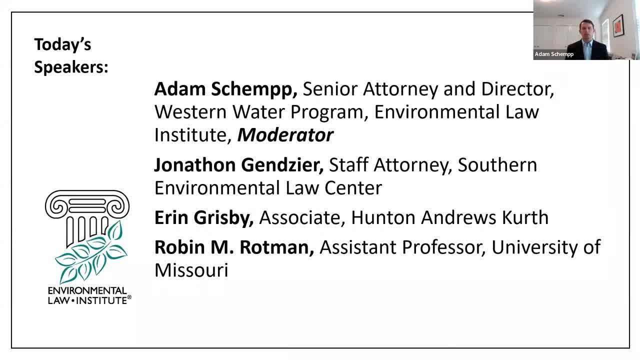 To reiterate what Chandler just mentioned about the questions, please submit them as they arise to you and do so through the questions box. This will ensure a much more efficient transition to the Q&A period, but also, if there's anything, that's sort of a quick clarification for any of the presentation materials. 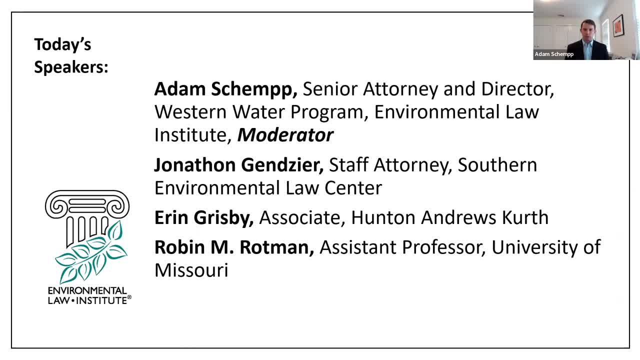 I'll ask that in between the two, the three presenters, to try to make sure that that information gets addressed pretty quickly. So again, please submit your questions as they arise And for anything that's quick, we will address it before we move on to the next presenter. Things that are going to be a little bit more substantively involved, we'll save to the end. 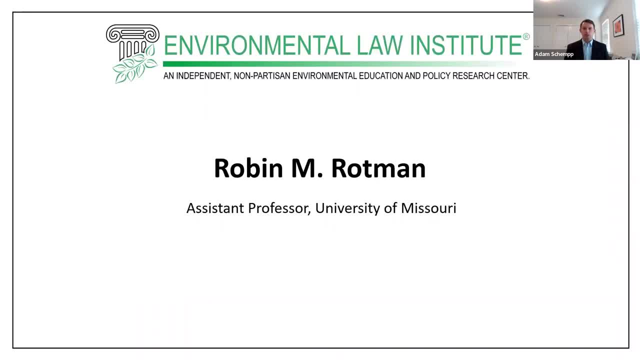 So with that I would like to introduce Robin Rotman. She is an assistant professor at the University of Missouri, having moved to academia after a decade of practicing environmental law at the Missouri Department of Natural Resources and at Bendis-Feldman LLP in Washington DC, where she continues to serve as counsel. 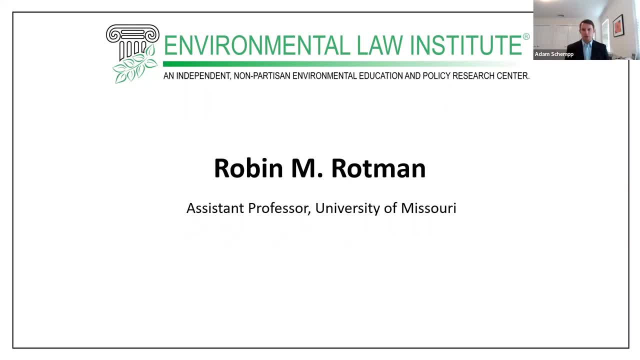 Robin's primary interests are water resources and water quality, land use and environmental justice. She earned her bachelor's degree in geology from Sewanee, the University of the South, her master's in water science from the University of Oxford, where she was a Rhodes Scholar, and her JD from Yale Law School. So with that, Robin, the floor is yours. 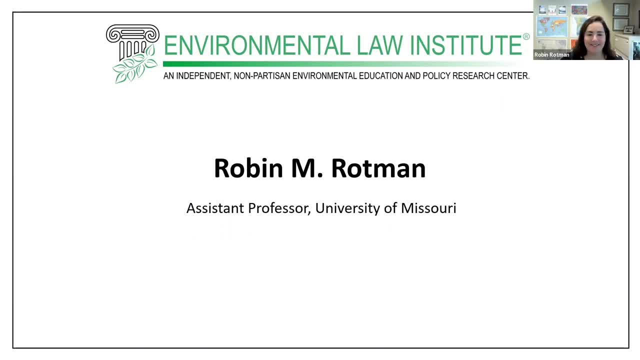 Thanks so much, Adam And Chandler. thank you for the opportunity to participate today. It's great to see we have, I think, right now 261 participants, probably including undergrad students, law students, summer law clerks associates, So it's great to see such a good turnout today for our discussion of the Clean Water Act. 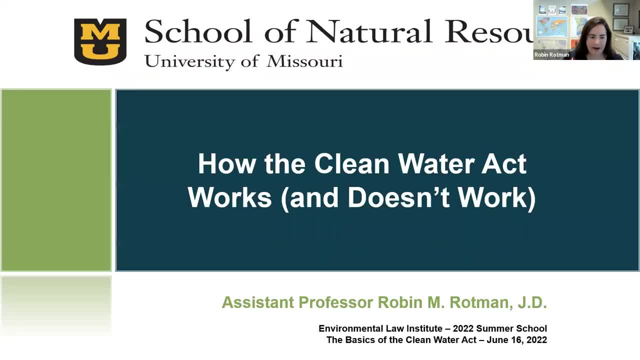 And let's see if I, if I can be there, we are Okay. so it looks like they've given me control of the slides. As Adam said, I'm Robin Rotman, I'm an assistant professor at the University of Missouri and I'm going to be starting things off with a broad overview of the Clean Water Act. 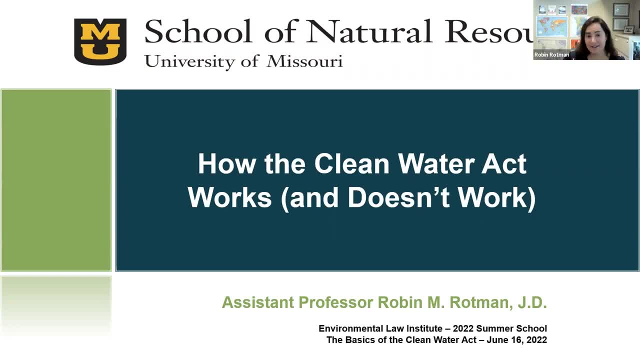 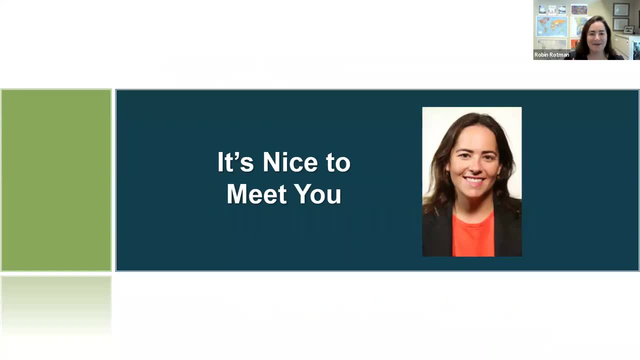 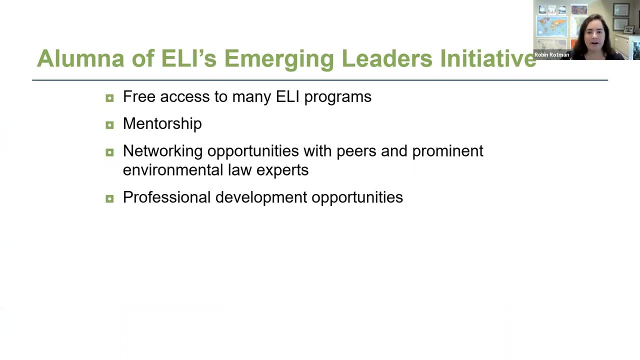 Basically how it works and also some commentary on how it doesn't work. Again, it's nice to meet you. I hope one day we'll be able to gather again in person. And I wanted to put in a plug for a program that ELI offers called the Emerging Leaders Initiative. So this is a program that I was previously a part of and it is a cohort program for junior practitioners in environmental law. 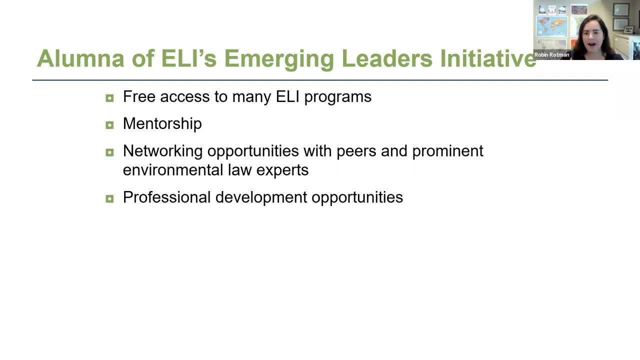 And so it offers access to ELI programming, mentorship, fantastic networking opportunities. When I went through it was during the COVID era, so entirely virtual, but it was still a great way for me to meet other peers and more senior practitioners. 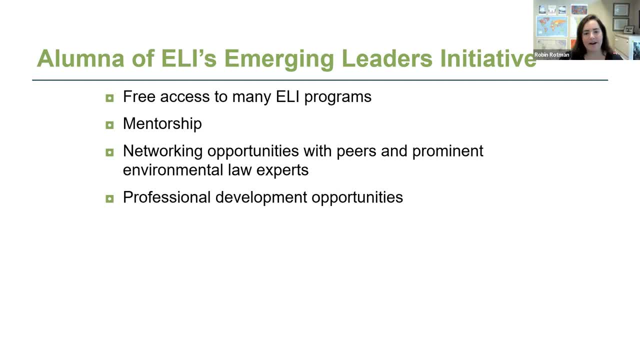 And also offers some professional development opportunities like writing an article or even giving a presentation such as this one. So if you would like more information, I'm sure that the Chandler or Adam can provide more information, But I just wanted to note that that was a program I had participated in and found quite valuable. 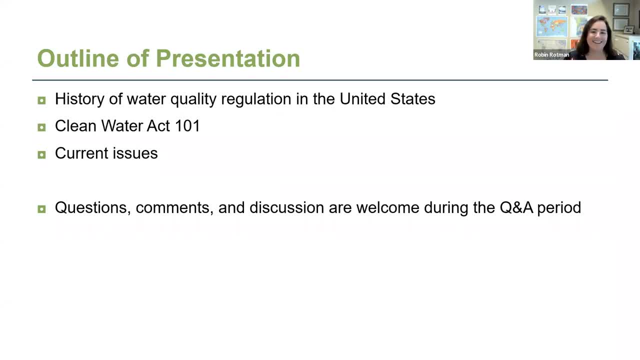 So, in terms of my presentation, we're going to do three things. First, I'm going to give a quick history of water quality regulation in the United States. So we're going to go all the way back to the Constitution and some very early case law. that then leads us up to the Clean Water Act. 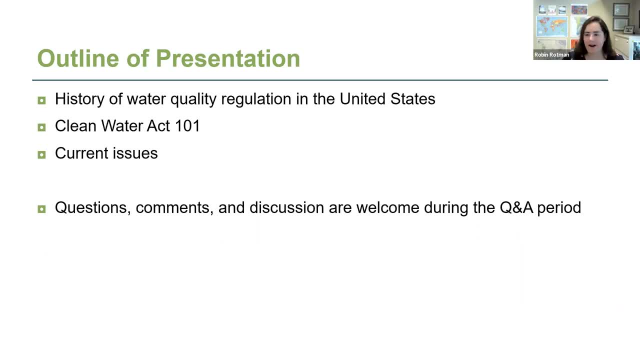 So I'll discuss the main components of the Clean Water Act And how they work, And then I'm just going to tee up a couple of those current issues, like the waters of the United States definition, or the county of Maui case, which then Jonathan and Aaron will discuss in detail. 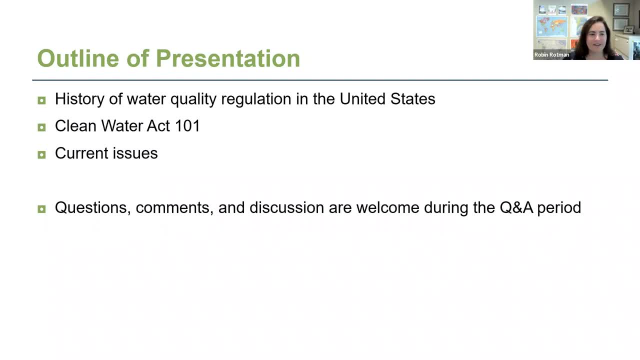 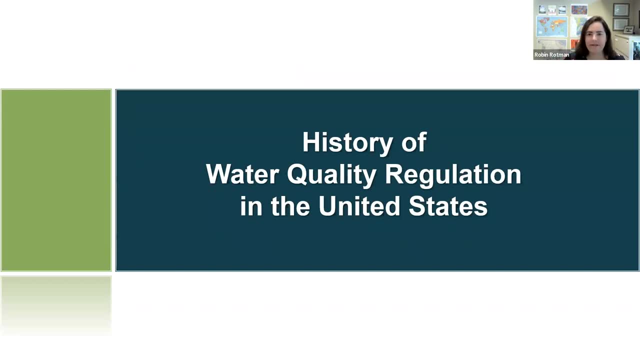 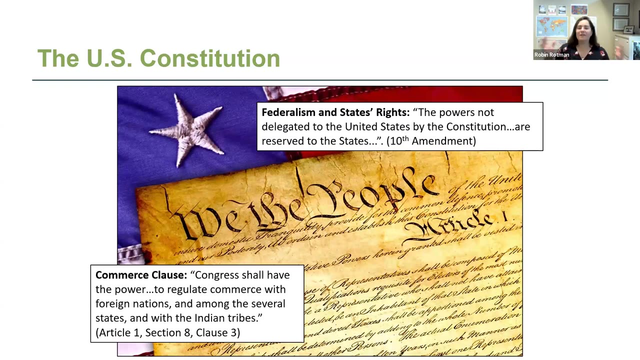 And, again, I look forward to your questions or your commentary during the Q&A period. Okay, so, diving into the history, It all starts with the Constitution And I just I know that we've all studied the Constitution, whether that be in elementary school or high school, or those of us who are attorneys. certainly we've taken constitutional law. 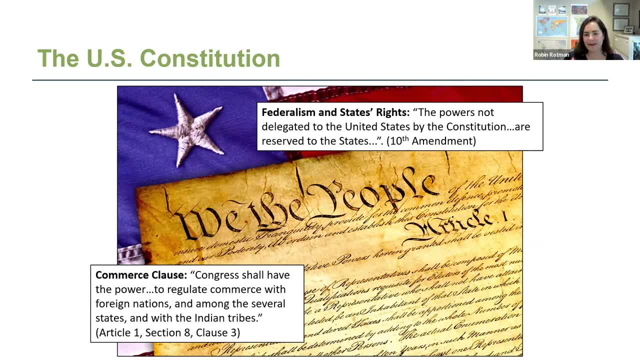 But just a couple of principles to ground ourselves in as we look at the Clean Water Act and other environmental laws. Which is so? we are a nation of states that came together and ceded certain rights to the federal government, So not every country is like that. 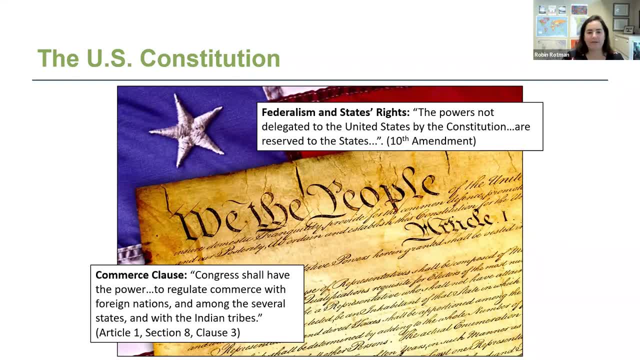 But so we had states with states rights Came together, delegated some of those rights to the federal government in the Tenth Amendment of the Constitution. But this amendment says that those powers that the states did not expressly give to the federal government are retained by the states. 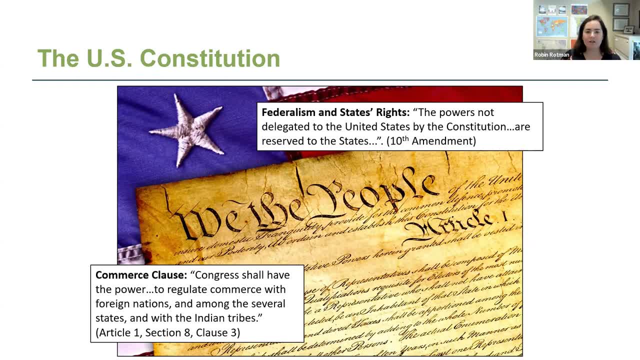 And so, over and over in environmental law we see these questions of well, what is within the proper purview of the federal government, like the EPA, and what is in the purview of the states, And that's a theme that comes up in particular in the Clean Water Act. 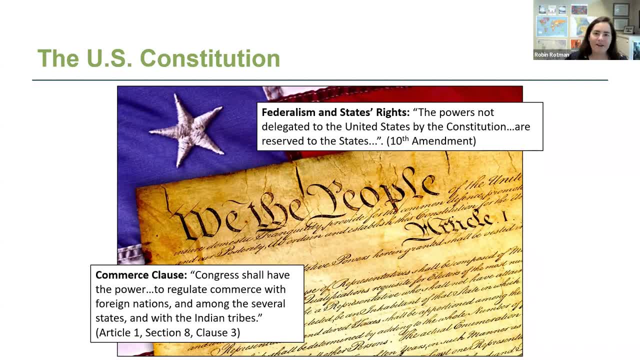 The other key provision I want us to keep in mind is the Commerce Clause, which says that Congress, so the federal government, has power to regulate commerce with the foreign nations, among the states and with the Indian tribes, And so this Interstate Commerce Clause has been used as a basis for federal jurisdiction over many different types of issues. 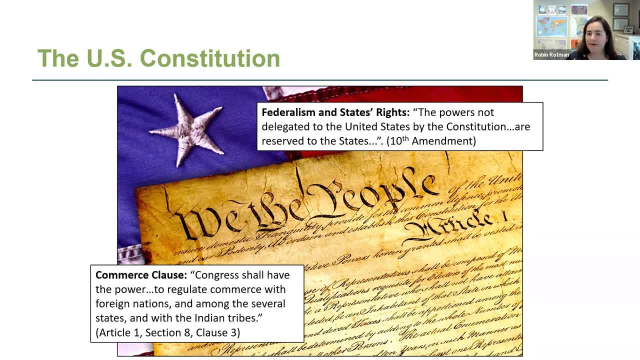 We'll speak about it in the environmental context today, But I think more, Perhaps more significantly, was an anti-segregation provisions. So when we hear back about, you know, restaurants that would not admit people of a certain color, or facilities that segregated people by color, it was the federal government's power through the Commerce Clause that had those state laws to be overturned. 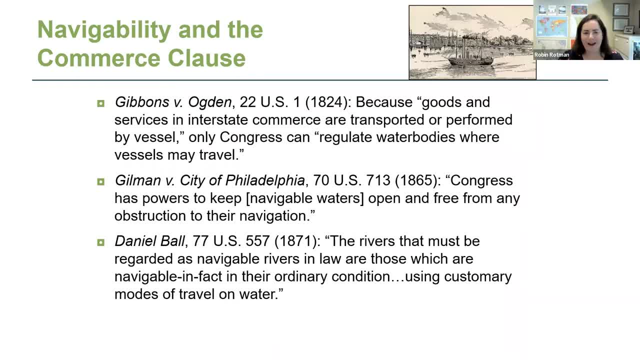 So let's dig into this question of: well, what does the Commerce Clause have to do with water quality? Well, it actually goes way back to some very early case law From the 1800s. So the first case I want to summarize is called Gibbons versus Ogden. 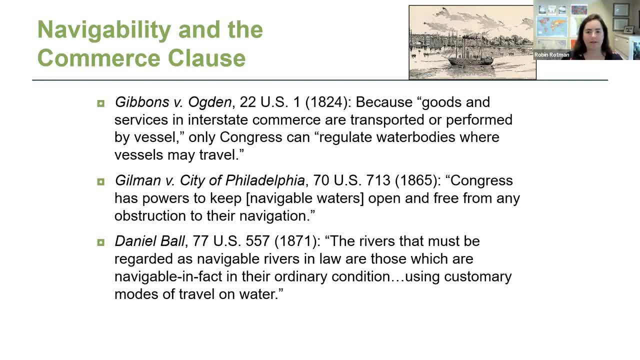 And this involved some passenger steamship routes between New York and New Jersey and the efforts by those states to regulate those steamship route rates. So the Supreme Court shut down those state standards on the basis that goods and services in interstate commerce that are transported by vessel. 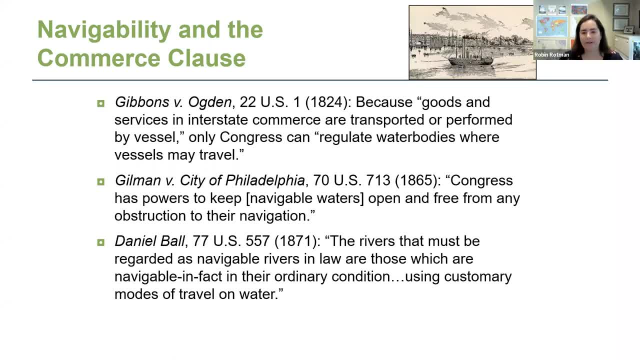 It's a matter of interstate commerce and therefore only Congress can regulate those water bodies. And then, about 40 years later, a case involving a bridge in the city of Philadelphia. some boat operators complained that the bridge was going to be an impediment to navigation, but the city wanted to construct it and the state 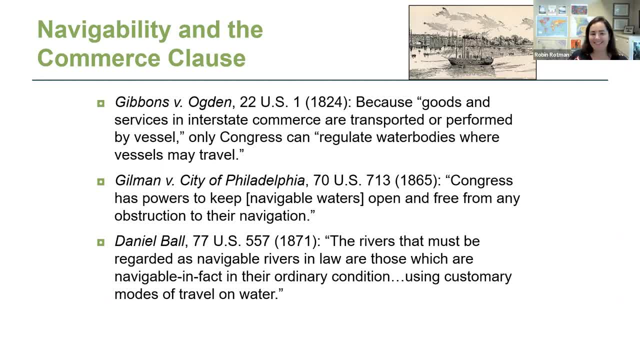 The Supreme Court refined its position saying that Congress- so not the states, but Congress- has the power to keep navigable waters open and free from any obstruction to navigation, and this was due to its Commerce Clause authority. So the first case that actually then defined navigable waters is the case called the Daniel Ball, and this had to do with a regulation of a steamship licensing in the state of Michigan. 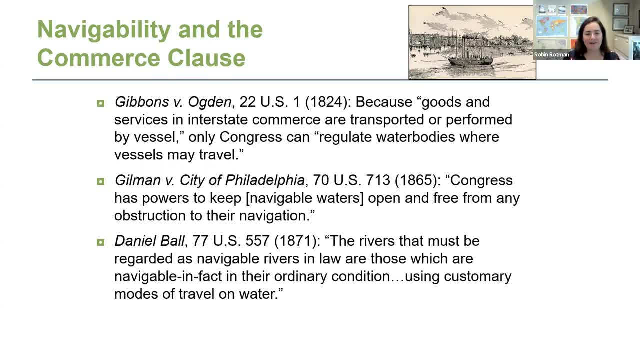 And the Supreme Court held that, basically, when we talk about navigable rivers for legal purposes, those are those which are navigable, in fact, in their ordinary condition, using customary modes of travel. So basically, this says: you know, if you could float a boat on it, if you could actually conduct commerce in this water body, it's navigable, in fact, and therefore also navigable in the eyes of the law. 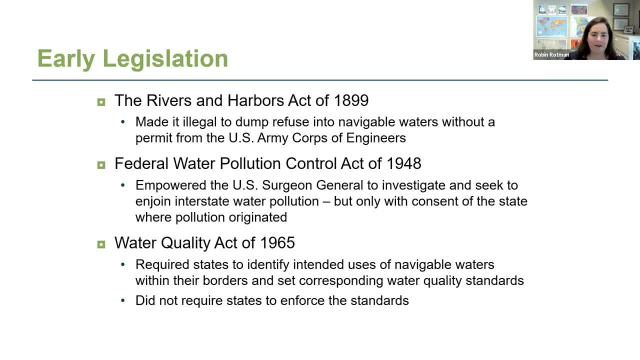 So some of the legislation that led up to the passage of the Clean Water Act also focused in on this navigable waters definition. The Rivers and Harbors Act of 1899 is often called the first American environmental law, and it made it illegal to dump refuse or debris into navigable waters without a permit from the Corps of Engineers. 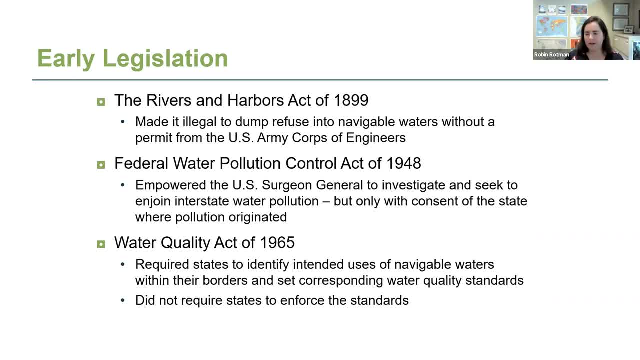 And so the basis here was, you might think well, the Corps. we'll talk in a moment about the role of the Corps. The motive: we call this the first environmental law, but the motivation at the time was not necessarily environmental. 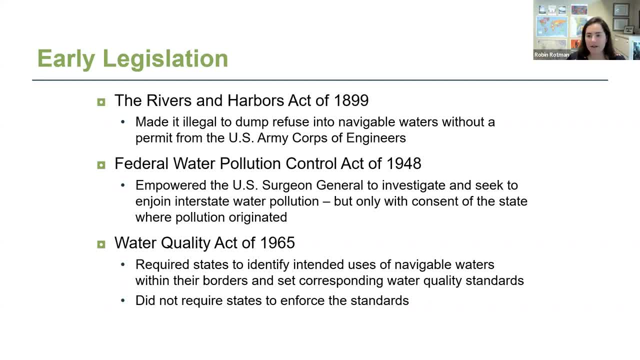 It was to promote navigation, And, as people were dumping trash into rivers and more urban areas, this was an impediment to boat travel, And so this act made it illegal to dump that refuse without a permit. That's really all we had on the books until the mid-1900s, when the Federal Water Pollution Control Act- now this was the first act that- 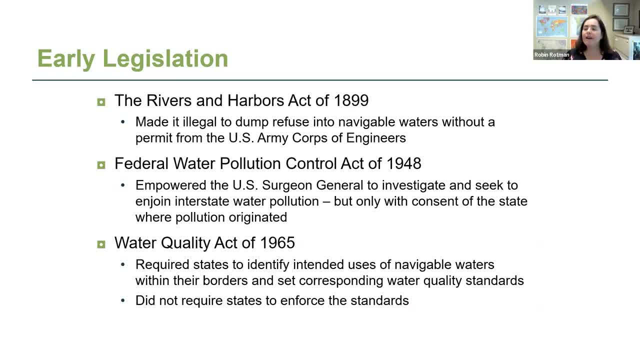 sought to do something about water pollution in the way that we think of it today, So not just debris that had been deposited and interfering with navigation, but actually pollutants that affected water quality. And so this act empowered the US Surgeon General to investigate and seek to enjoin, so seek to get an order from a court to stop water pollution that was originating in one state and affecting another. 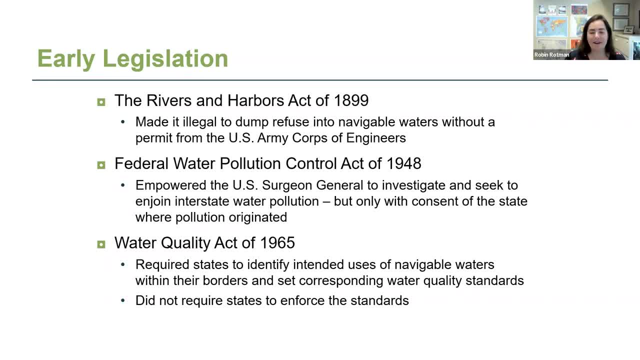 However, this authority was more limited than it sounds, because the Surgeon General could only do this with the consent of the state where the pollution originated. And probably not surprisingly, a lot of states didn't give this consent because they saw that it might negatively impact their industry and they might not have really cared if this water pollution was ending up somewhere else. 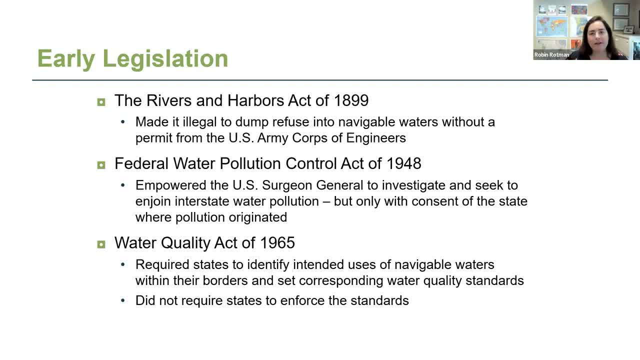 The Water Quality Act of 1965 is really the precursor to the modern Clean Water Act and contains a similar structure. So it required states to identify the quality of water in the state. So it required states to identify the quality of water in the state. 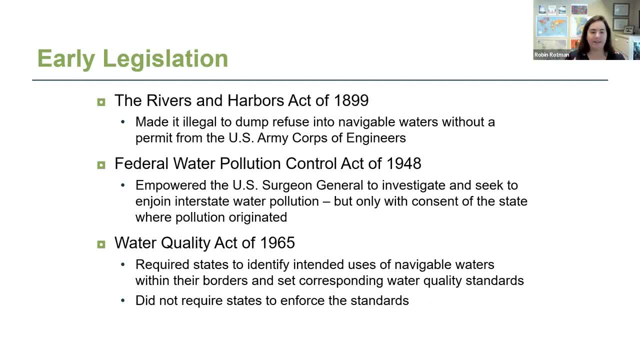 So it required states to identify the quality of water in the state, identify the intended uses of navigable waters within their borders and set water quality standards that would support those intended uses. So this was more of a planning exercise. so it required that identification, the setting of standards, but it didn't actually require states. 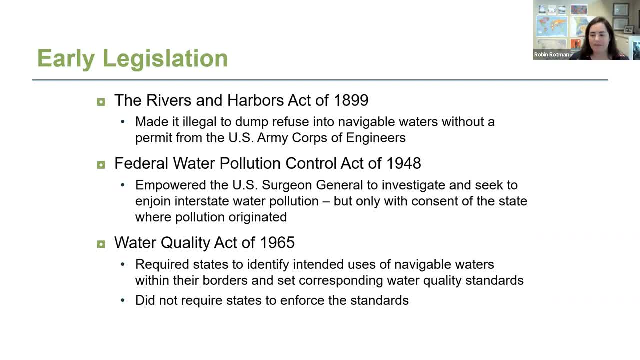 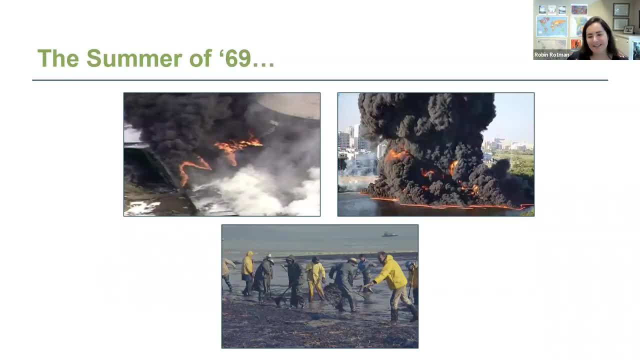 to enforce those standards, And so, without an enforcement mechanism, it wasn't a particularly effective law. And that brings us, if you might know the song- the summer of 69, to a number of events that occurred in 1969 that really captured the public attention. So here I've had a picture. 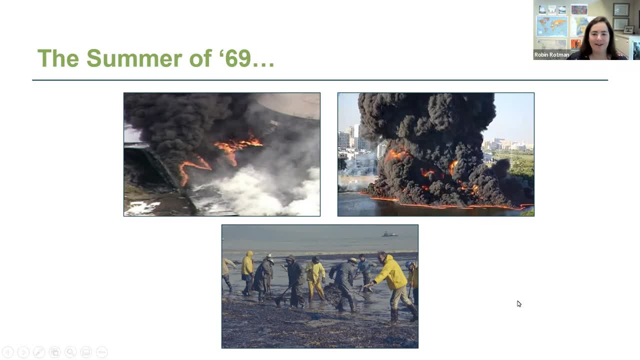 of the Cuyahoga River in Ohio catching fire, Also one of the Rouge River in Detroit. I could have also put one of Lake Erie that also caught fire that same year. And then, also, looking at coastal issues, This is an oil spill off the coast of Santa Barbara, California. 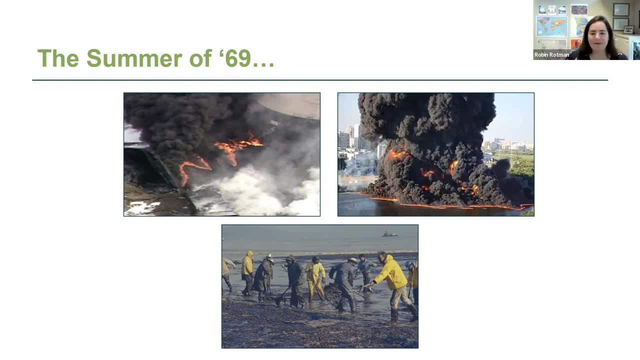 And so all these events happening in relatively close proximity brought the issue of water pollution more into the minds of the American public, And so more and more the electorate began demanding that the elected officials take some action to address this problem. Now, certainly this wasn't only Clean Water Act. The late 60s through the 70s was a time where 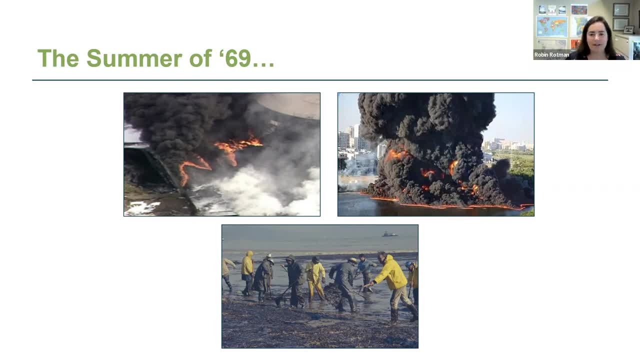 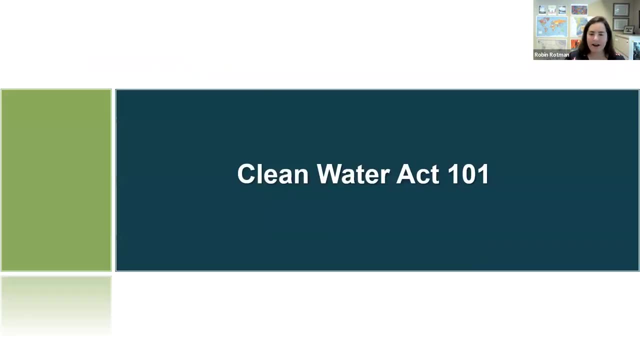 many of the modern environmental laws were passed. So, as we all have probably heard from many people, as public attention just grew generally regarding environmental protection, So that kind of takes us through the history. And now I want to go through the nuts and bolts of how the Clean Water Act works. 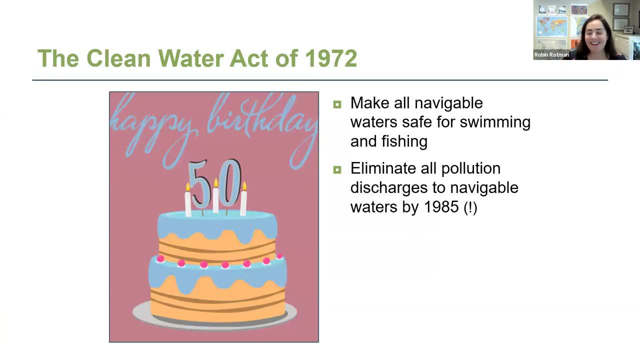 Well, I would note that it's the Clean Water Act's 50th birthday this year, And so this is done to address water pollution in the United States. So at the time it was passed, in 1972, the Clean Water Act contained two main goals. First, to make all navigable waters safe for 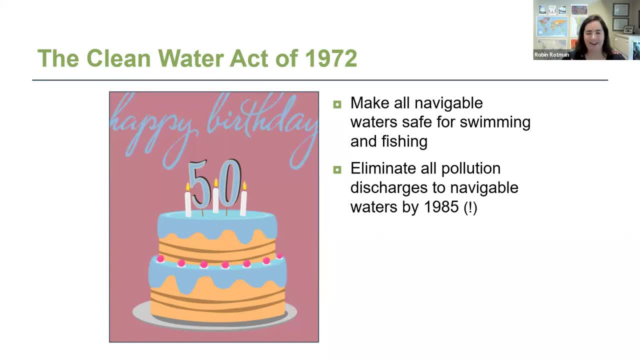 swimming and fishing, which remains a goal today. The second was pretty ambitious: eliminate all pollution discharges to navigable waters by 1985. Certainly didn't meet that target. We still haven't met it today But, as I'll describe, we have made some progress in controlling pollution. 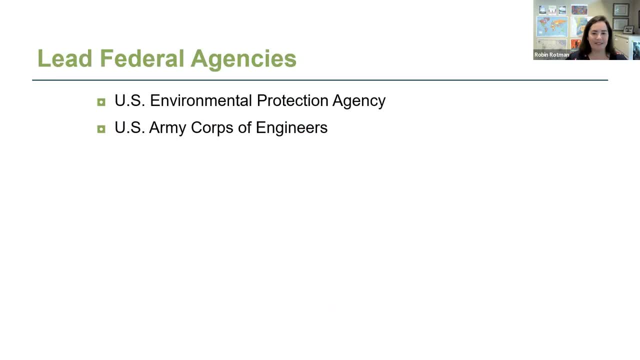 discharges. So two main agencies Overall. the US Environmental Protection Agency is the agency charged with implementing most provisions of the Clean Water Act, And so when I talk about permitting with the non-point source and point source, it's the EPA that's really driving the train on that. 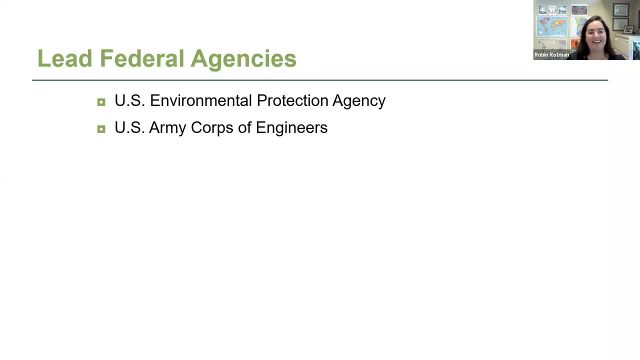 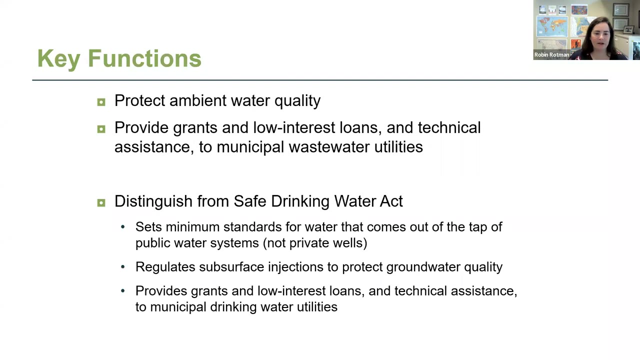 However, as I mentioned, historically there was an emphasis on navigation and navigability of waters for defense purposes, And that's why, even today, the Army Corps of Engineers still plays a role in permitting. So the two big functions of the Clean Water Act are to protect ambient water quality. So this is 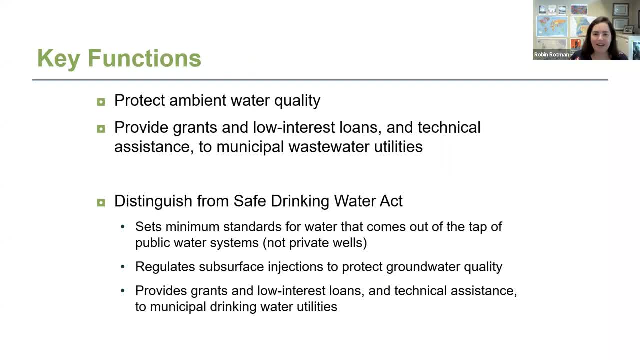 the quality of water in the environment, like our lakes, our rivers, our streams, And this is what we'll focus on today. I did want to mention briefly, though, that there's a second key function, which is for the EPA, under the Clean Water Act, to provide grants and low interest loans. 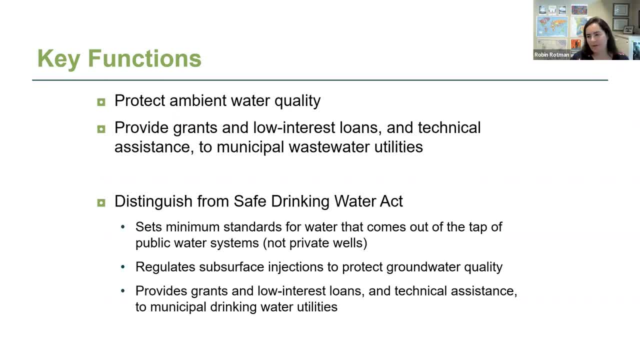 and also technical assistance to municipal wastewater utilities. So you might have heard of the State Revolving Funds Program. This is a way that municipal wastewater treatment plant or sewerage districts can get access to loans and capital to make improvements to their infrastructure Again. 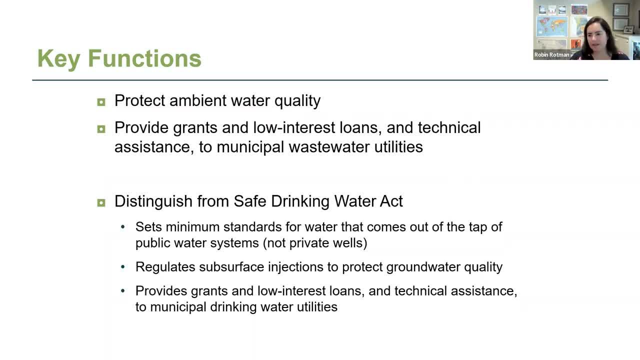 we'll focus more on the water quality protection, But these are. this is hundreds of millions of dollars every year, So these, these grants are not insignificant. Now I want to take just one moment to distinguish the Clean Water Act from the Safe Drinking Water Act. 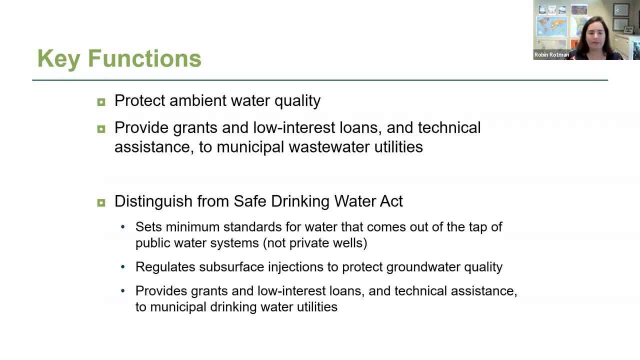 So the Clean Water Act, like we said, protecting ambient water quality. The Safe Drinking Water Act, on the other hand, sets minimum standards for the water that comes out of our tap of public water. So these are the standards for the water that comes out of our tap. 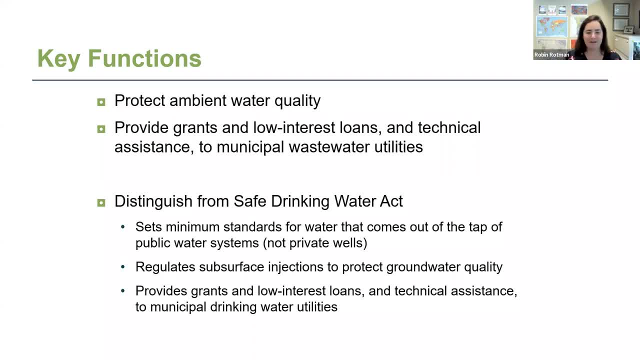 of public water systems. So here I. you can see, I got my water bottle. I filled it up this morning. I filled this up at my home public water system, And so this water would be regulated by the Safe Drinking Water Act. 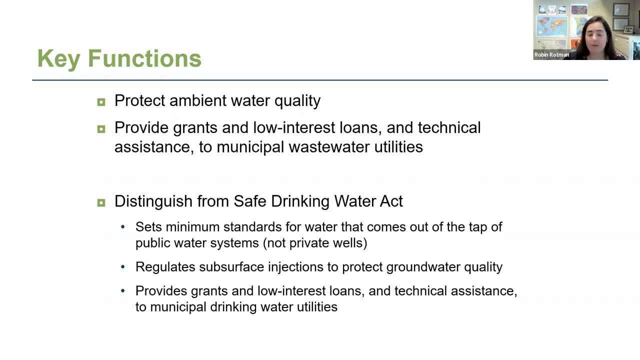 I would note that the Safe Drinking Water Act does not cover private wells, So perhaps if you're living in a more rural area you have a private well. If that is regulated at all, it's probably regulated at the county level. So the Safe Drinking Water Act doesn't oversee bottled water quality. 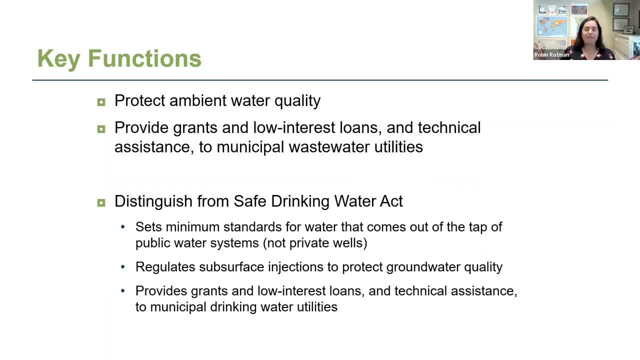 That is handled through the Food and Drug Administration. Okay so, but big picture, Safe Drinking Water Act, tap water quality. It also, though, regulates the injection of pollutants into the subsurface, And this is because there's a clear link between pollution injections into the subsurface and water quality that could be used for drinking water. 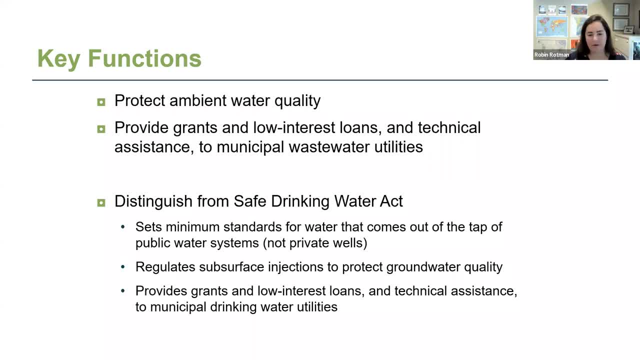 And, just like the Clean Water Act, it provides a financial assistance program, This time to drinking water utilities. The Safe Drinking Water Act was passed in 1974. And I would just take a moment to make an aside, which is that in that era, drinking water and ambient water were really seen as two separate resources. 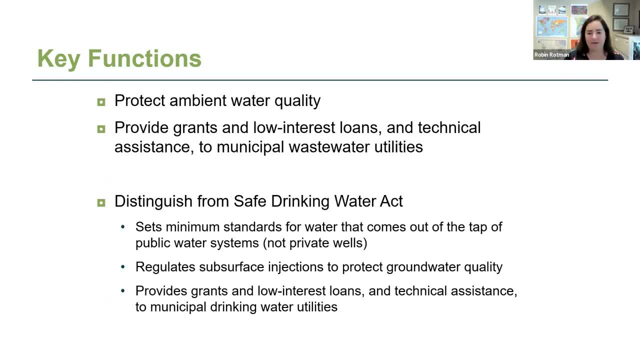 Likewise, surface water and groundwater were seen as two separate resources. Of course, now we have a better understanding of hydrogeology, the water cycle, We understand how water in the air is used And the ambient environment affects the quality of the water we drink. 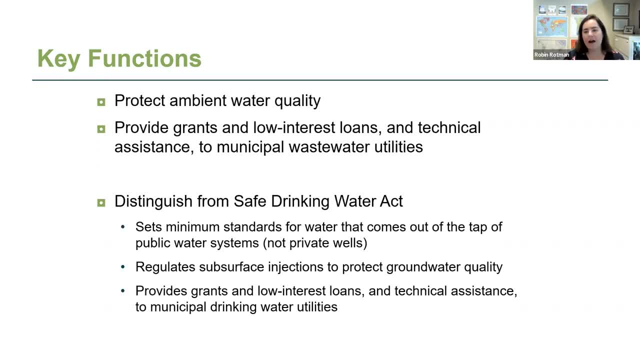 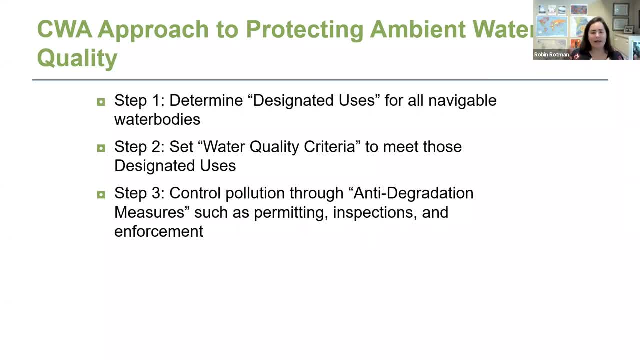 But they also sound a lot like the 1965 Act. Okay, just slightly different terminology. So the first is to determine the designated use. Okay, before it was called intended use, Now designated use for all navigable water bodies, So that could be as a drinking water source. 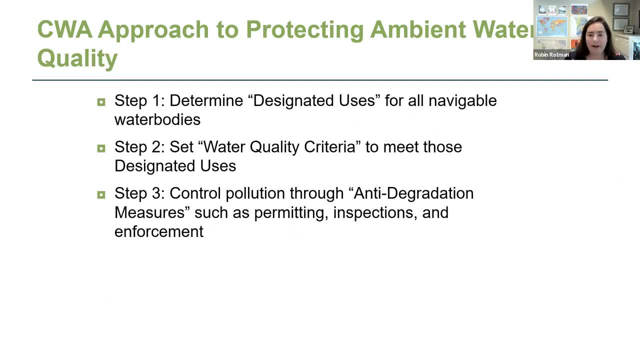 It could be for hydropower, It could be for irrigated agriculture, It could be for fishing and swimming, and so forth, And then setting water quality criteria area to meet those designated uses. The Clean Water Act, though, goes further by implementing 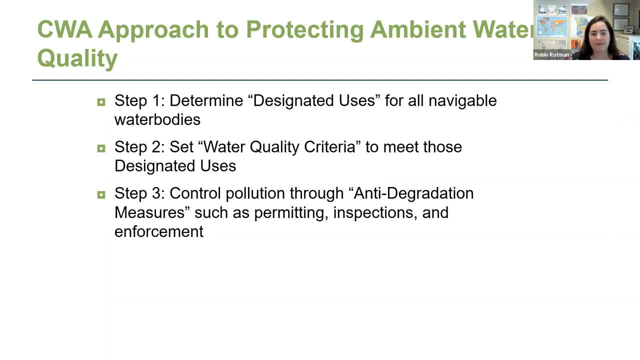 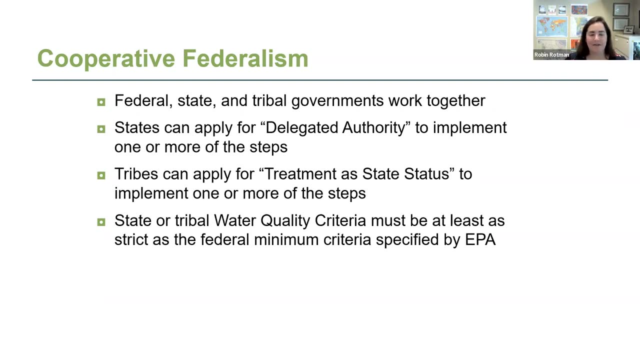 anti-degradation measures. So this is what gives the first two steps like the teeth through: permitting inspections and enforcement. Now you might have heard of the topic of cooperative federalism. We talked a little bit about federalism before, But this is the idea that the federal, state and tribal governments. 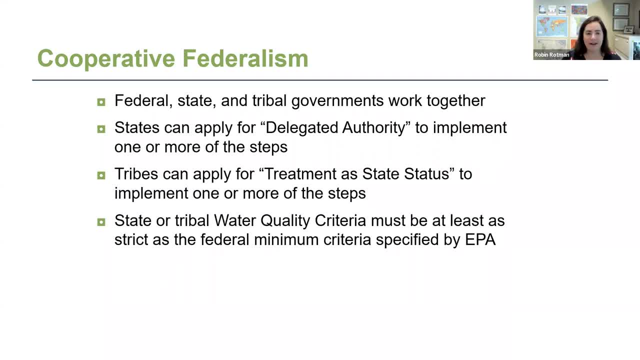 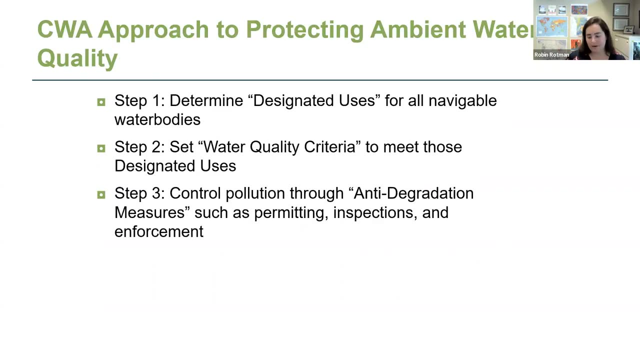 work together to implement the environmental laws, And in fact the Clean Water Act is often held up as kind of the poster child of cooperative federalism in the environmental context. And that's because states can apply for delegated authority to implement one or more of those three. 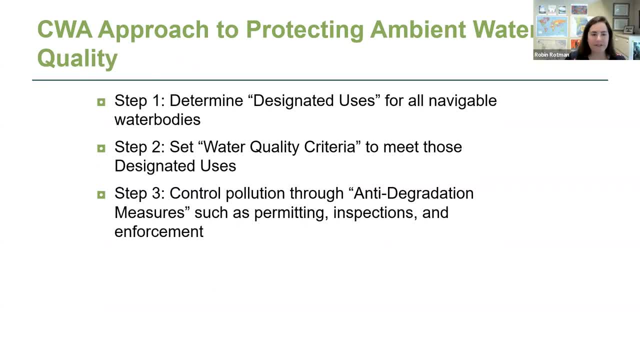 functions And, as it is today, actually all 50 states have some amount of federalism, There's some amount of delegated authority for designating uses and setting water quality criteria, And 47 states have authority to issue permits, conduct inspections and do enforcement. 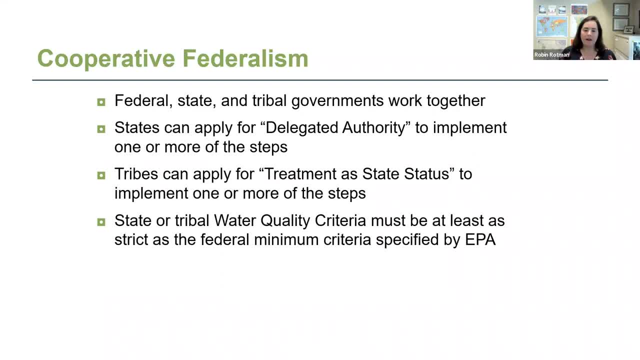 activities. That delegated authority was built into the Clean Water Act when it was passed in 1972. At that time, at the time of passage, the Clean Water Act didn't envision that Native American tribes would have a role to play. But through Clean Water Act amendments, tribes can now apply for treatment of state status. 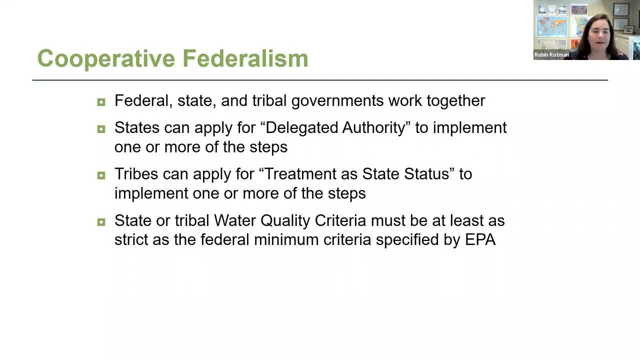 which basically means that they can apply, just as the states can, to implement one or more of the regulatory functions, And today 80 out of the approximately 560 federally recognized tribes have that authority. So I said it's cooperative, though The states and tribes can't just do. 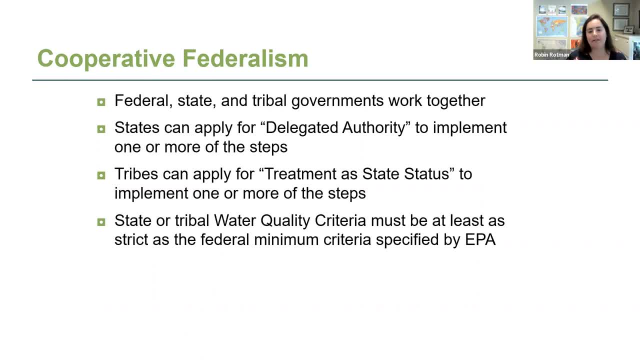 whatever they want, They have to comply. The state can't like do whatever they want, because they have to comply with certain minimum criteria that are specified by the EPA. So they have the ability to make stricter standards, to say that they want to have a higher quality of water in their jurisdiction, But they can't. 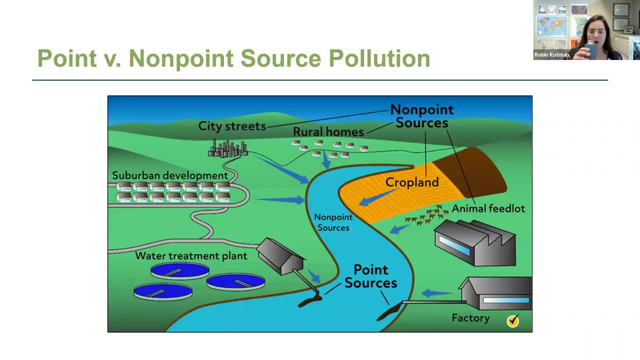 drop below those federal minimum standards. The Clean Water Act recognizes two different types of pollution sources- Point sources- so these are like, literally, ones we can derivatively advocate on for for specific purposes, But this is just a general example of this and it's not just one of many, And so it's a 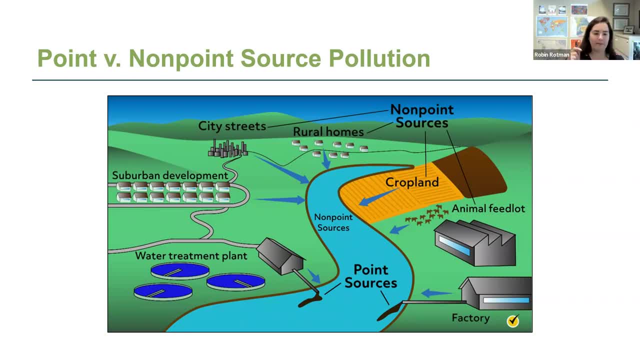 point to, like a pipe coming out of a factory or a pipe coming out of the wastewater treatment plant, as well as non-point sources, and these are more diffuse, like agricultural fields, highways, parking lot runoff, And I'll talk for a moment about how the Clean Water Act addresses. 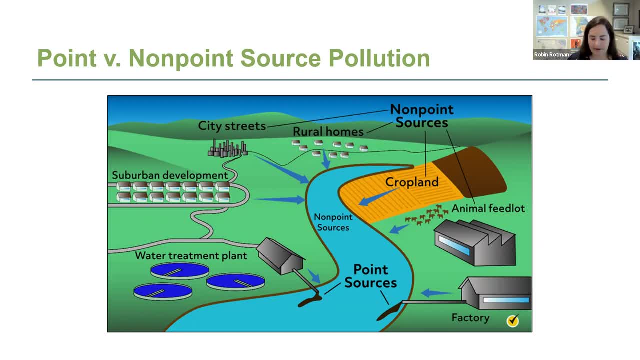 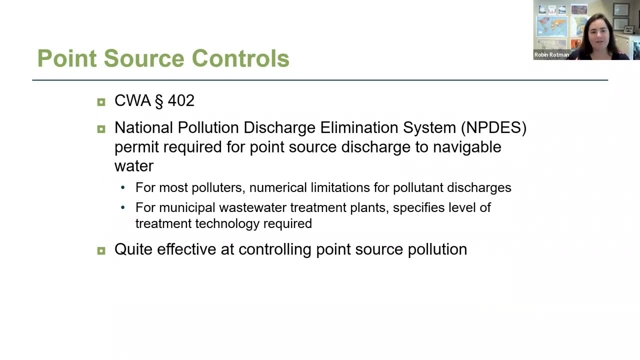 each of these sources, and then this is a topic that Erin will discuss in greater detail, Erin Neweyer MD. So the point- source control system- is fairly straightforward. This is set out under section 402.. And what this section says is that a permit from the EPA called the National Pollution, 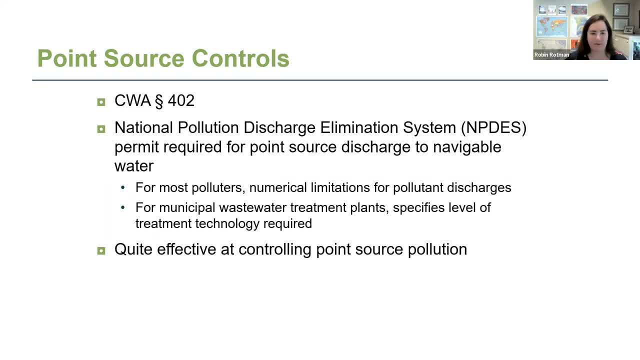 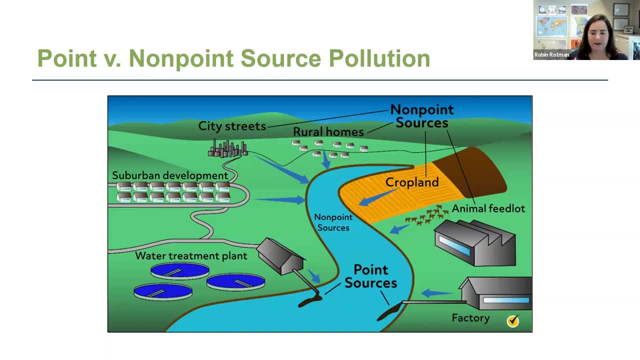 Discharge Elimination System Permit. NPDES permit is required for point source discharges, And so on the prior slide I have the factory here. So for most polluters such as a factory, the NPDES permit is required for point source discharges, And so on the prior slide I have the. 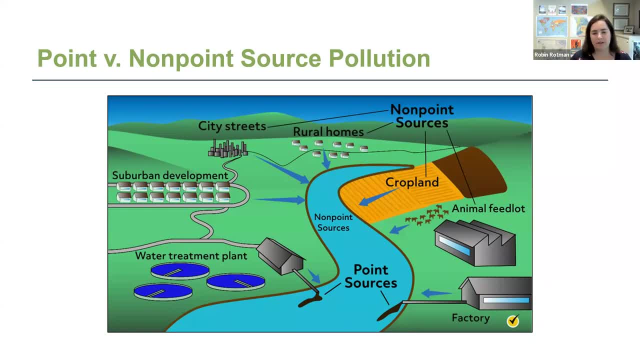 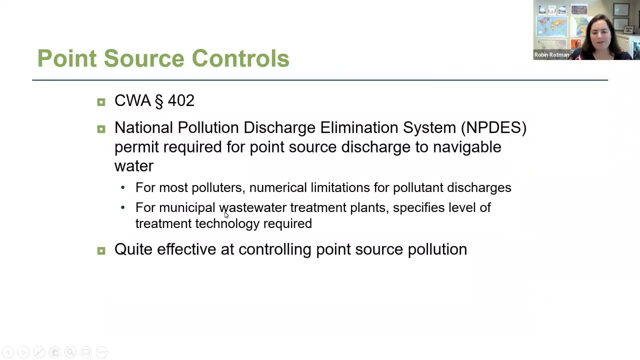 factory here. So for most polluters such as a factory, the NPDES permit is required. for point EDS permit will contain numerical limitations on how much of the various pollutants can be discharged. When it comes to the wastewater treatment plant, though, it's harder, because 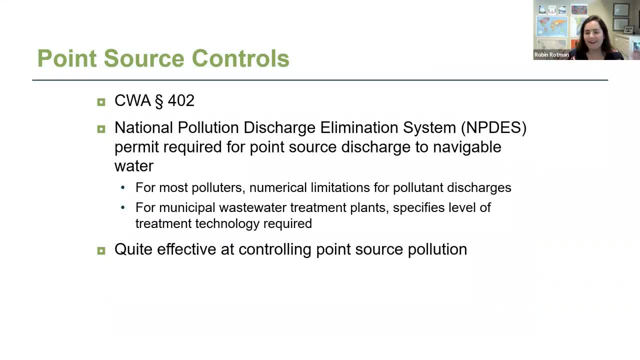 those plants have to receive whatever is coming into the sewer, And so, unlike a factory that has you know, like a well-established process for what they're producing, the wastewater plant is just receiving this water without even knowing what's in it, And so the permit, instead of specifying. 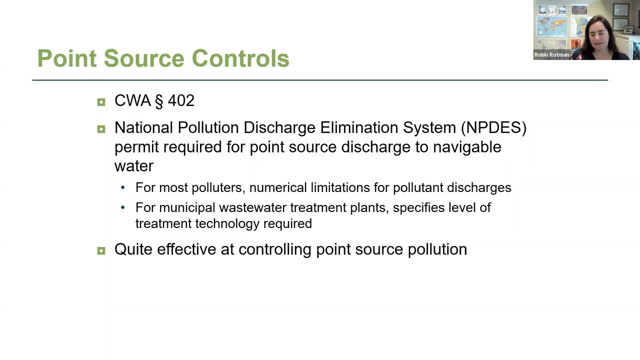 affluent limitations. it specifies the level of treatment technology required. So that would be whether primary, secondary or tertiary wastewater treatment And I'm happy to expand on that in the Q&A And overall Clean Water Act. Section 402 has been effective at controlling point source. 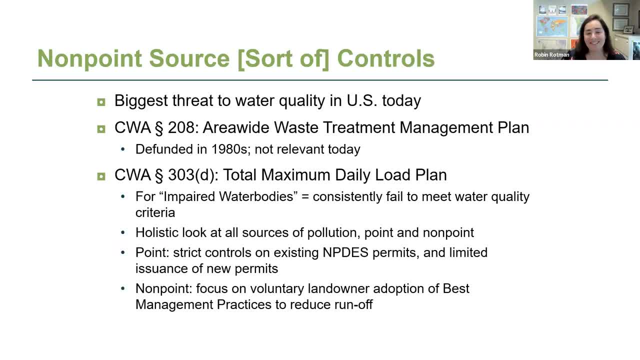 pollution, which might explain why today, the biggest threat to water quality in the US is actually non-point source pollution. Now, the awareness of non-point source pollution was built into the Clean Water Act. at the start, Section 208 required states to develop these area-wide waste treatment management plans. 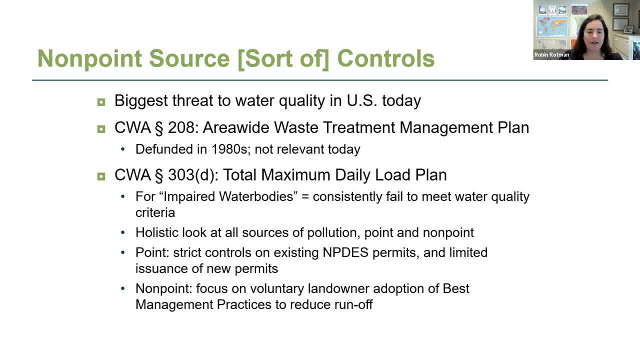 to address non-point source pollution. The idea, though, was that the federal government would give states a financial allocation in order to develop and implement these plans, But the program was defunded by Congress in the 1980s and is not relevant today. 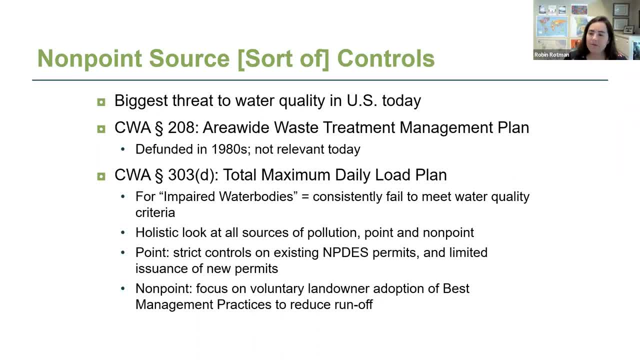 So there's two provisions that are relevant today. One is 303D, the total maximum daily load, and Erin will discuss this in detail, But just in brief I would say so. not all water bodies have a TMDL plan. It's only required for impaired waters, which are those that consistently fail to. 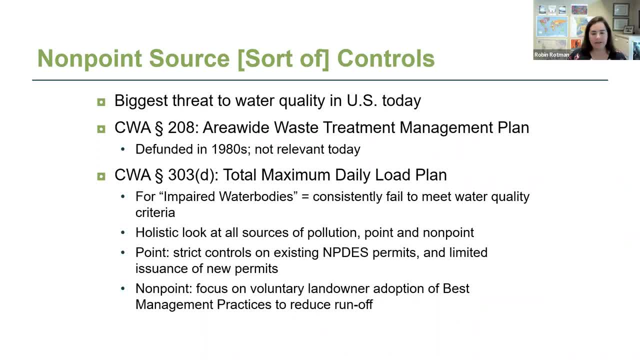 meet their water quality criteria, And so this is a very important part of the plan, And so the NPDES program looks at all the sources of pollution in the watershed point and non-point source. For those water bodies subject to a TMDL, the NPDES permits that exist can be tightened to become 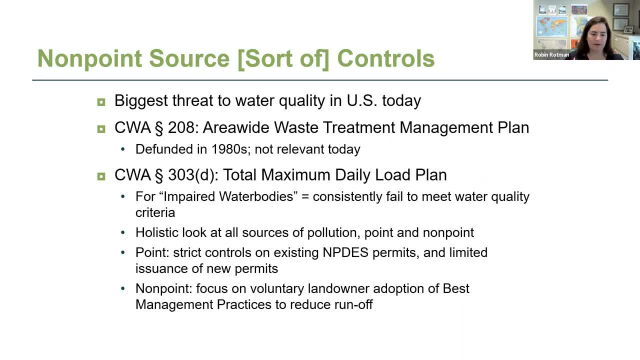 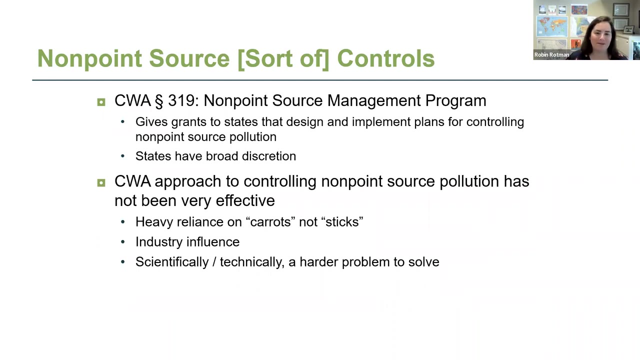 more stringent and there can be a limited issuance of new permits. On the non-point side, the main focus is encouraging states to encourage landowners to voluntarily adopt best management practices to reduce runoff off, like installing riparian buffers. Section 319 also tackles nonpoint source pollution and this takes the financial. 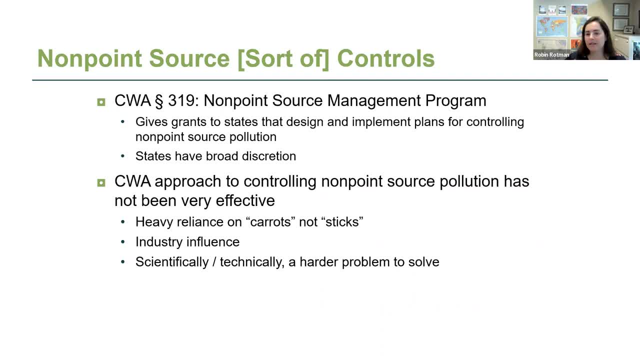 incentive approach by offering grants to states that design and implement PANs for controlling nonpoint source pollution. Oh, I see that, Jayla. I see your question. I'd be happy to take that afterwards. So again, this is focused on voluntary measures, but states have broad discretion as 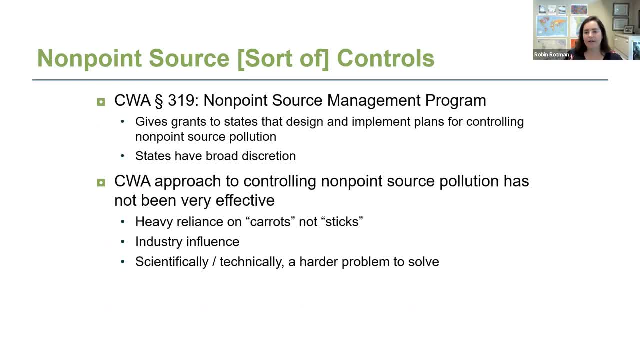 to how they're going to implement their programs And as long as they're showing some some progress in controlling nonpoint source pollution, these federal funds keep coming in But in the big picture the Clean Water Act has not been very effective to controlling. 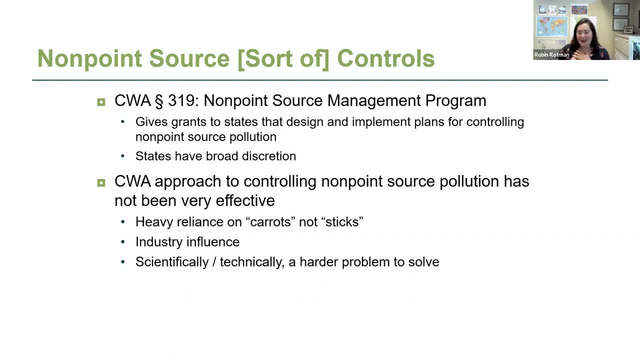 nonpoint source pollution In my. now I'm giving my opinion. OK, this is just opinion, you can disagree or disagree. In my opinion, it overly relies on the carrots, like these voluntary financial incentives, and not sticks like binding regulations. 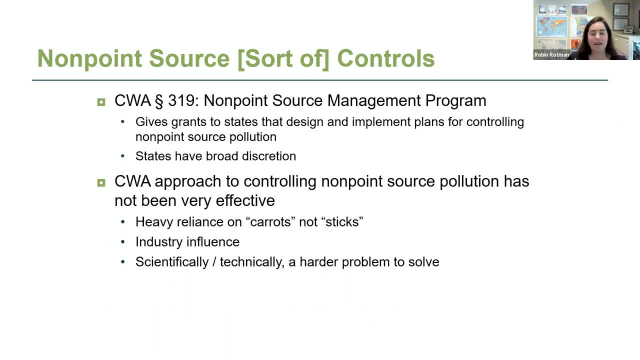 And, in my opinion, the reason for this is that the industries that are the primary sources of nonpoint source pollution have a strong lobbying presence. So these could be agriculture, this could be the home builders, this could be the transportation sector- industries that have a strong. 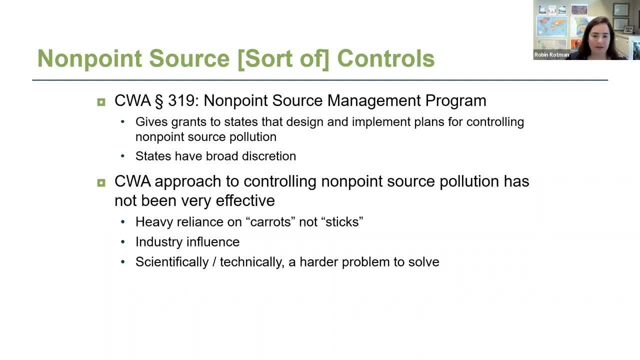 interest and not seen further regulatory measures imposed on nonpoint source pollution. And I'd also note- you know it's just harder, right, Like it's easier when you can look at a point and say this is what's happening at the 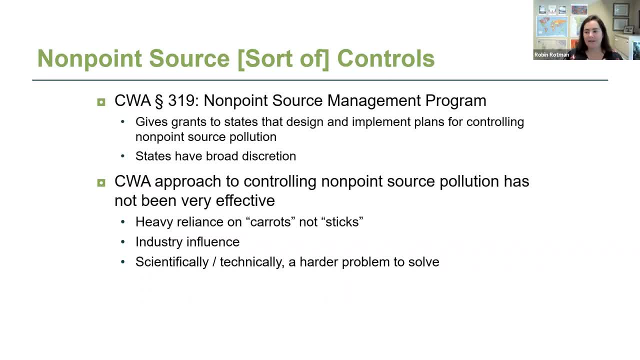 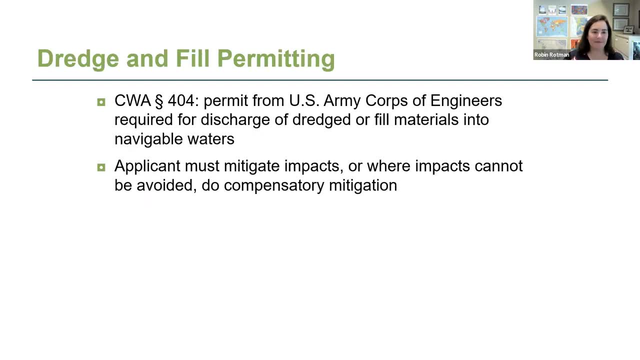 factory, we need to put on a certain control device. It's harder to identify and to address diffuse pollution sources. One other item I wanted to note, just to kind of round out this Clean Water Act one or one, is the dredge and fill permitting requirements under Section 404.. 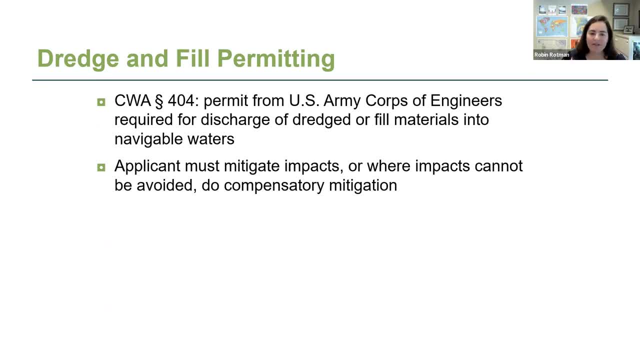 So, going back to this origins, on navigation, even today a permit is required from the Army Corps of Engineers for discharging dredged or fill materials into navigable waters, Where this really comes up. I mean, I guess you could, you could want to fill the Missouri. 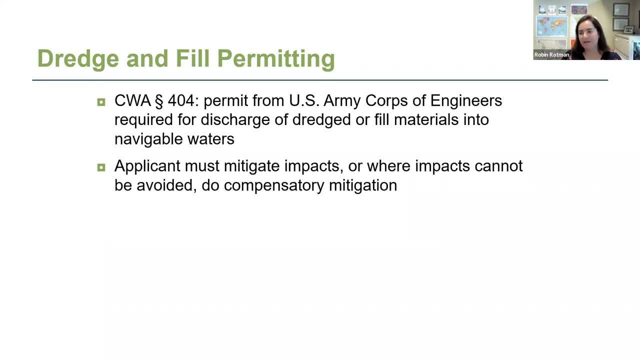 River, but that's not not really where it happens. It really happens in the wetland context, often when there's urban development, wanting to build commercial or residential development on areas with wetlands, And so this section says that, to the extent possible, those impacts need to be mitigated. on. 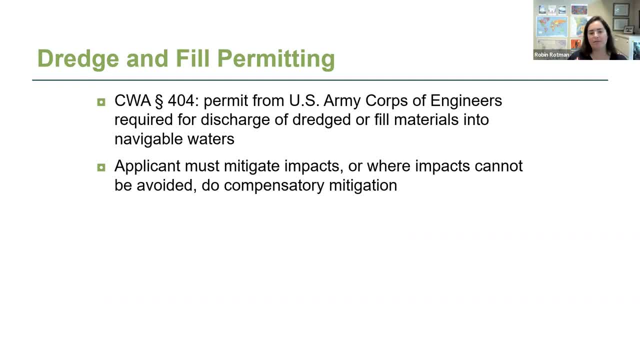 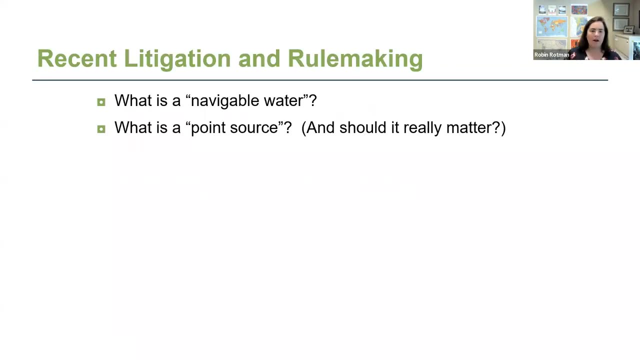 site, And if they can't be mitigated, there's the possible to essentially buy wetlands to be built somewhere else through wetland banking, which it calls compensatory mitigation. I know, Okay, Thank you. Thank you, my time is running short, so i'm just going to tee up these two issues, um so, two big issues. 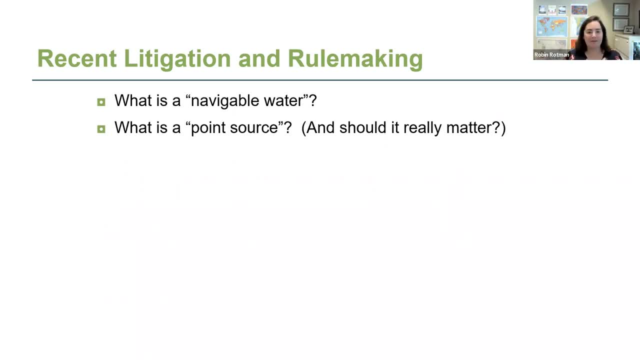 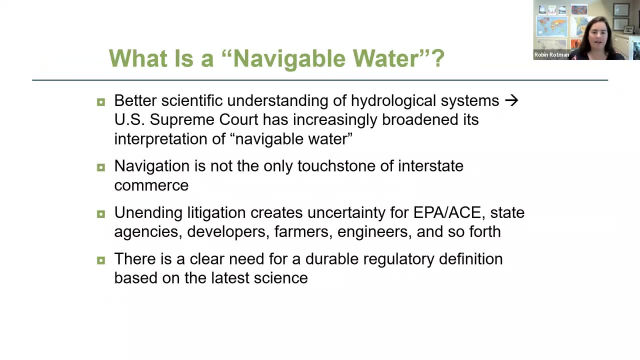 like: what is a navigable water, or what is the water of the united states, and further, what is a point source? so we saw that the early case law for navigability focused on navigability, in fact, like: can we float a boat carrying goods or passengers and commerce? 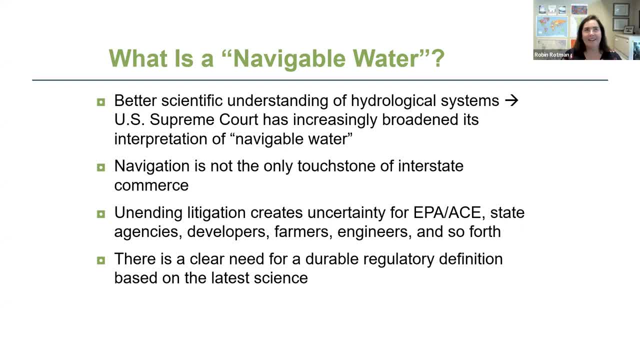 but of course, if you think about it today, navigation of water bodies is not the only issue that's relevant to interstate commerce. certainly, water quality, like we could think about um pollution from nitrogen or phosphorus that is causing um algal growth downstream, those are all issues that are also relevant to congress, to commerce. 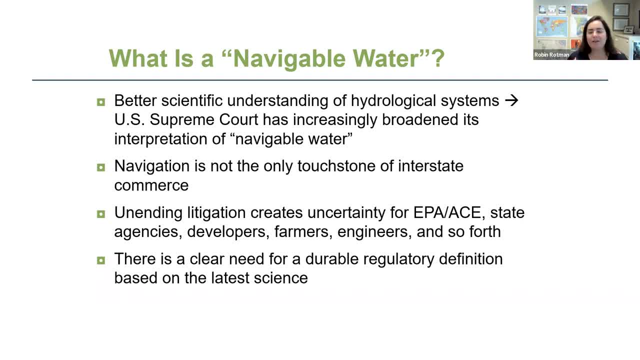 whether or not a boat is involved. uh, and so, over the past- well, at least 50 years- there's been a lot of talk about the importance of water quality in the interstate commerce. but of course, if you think about it today, navigation of water bodies is not the only issue that's relevant to interstate commerce. 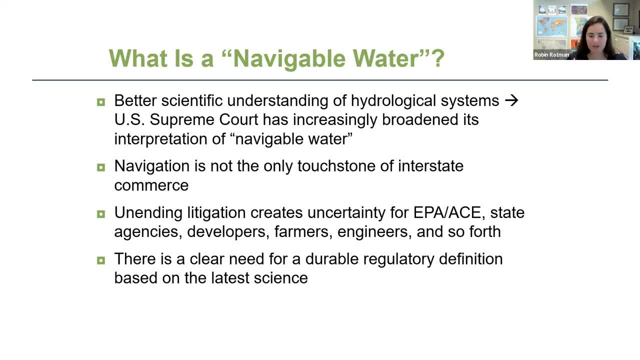 has been just an unending um pattern of litigation: rule making, litigation about the rule making, new rule making, litigation about the new right. you know about the old room like it just goes in circles and this becomes very difficult for everyone, right? so for the state agencies that. 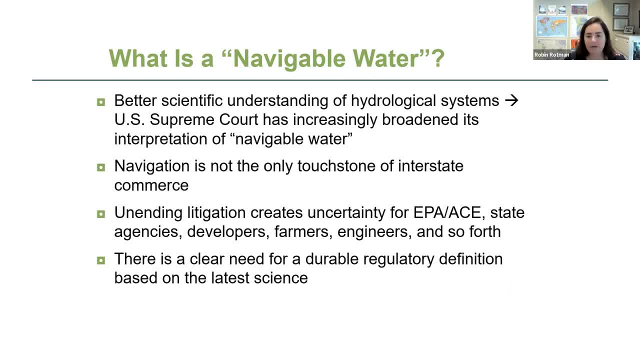 implement permitting programs for the regulated community, for environmental advocates, for engineers and attorneys that provide compliance assistance, and so i certainly believe that there is a need for a durable definition, so meaning one that that's lasting beyond the presidential administration. i think that that will be better for everyone. 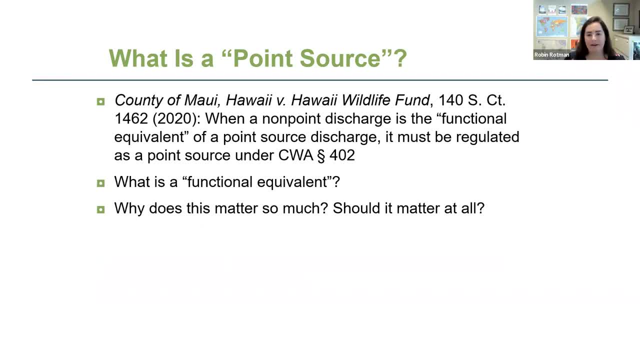 aaron's going to talk about this seminal case of the county of maui, which introduced this concept of a functional equivalent of a point source discharge. so it says that sometimes a non-point source can be the functional equivalent of a point source and therefore needs an npdes permit. didn't provide a lot of details on what constitutes. 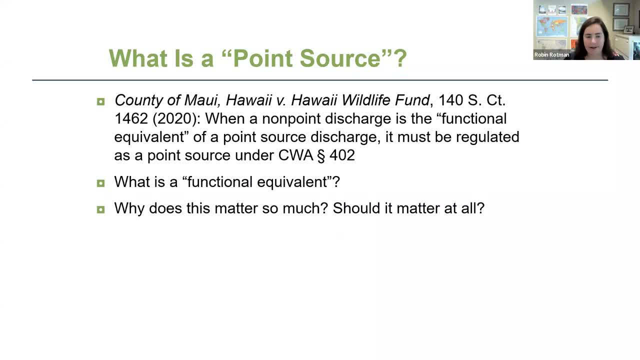 a functional equivalent. ultimately, the supreme court said it's a case-by-case basis. i just wanted to go kind of meta for a minute, which is: you know, why does this matter so much like? why do we even need to have this paradigm of this functional equivalent? um well, the answer is because we have inadequate regulation of non-point source pollution. 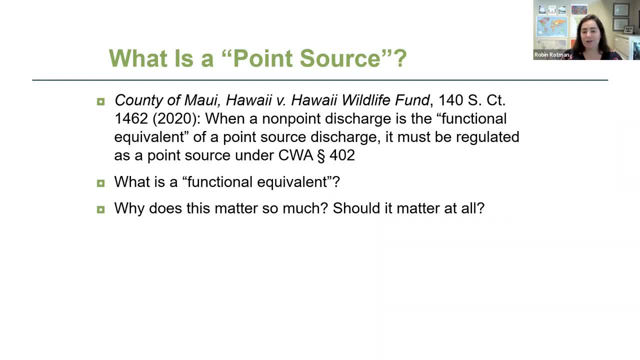 and so i think that the court, recognizing that, was trying to find any way to get at this pollution, which is clearly having an impact on the environment, by creating this construct of the functional equivalent. um, i'll be curious to hear what aaron has to say in her remarks. 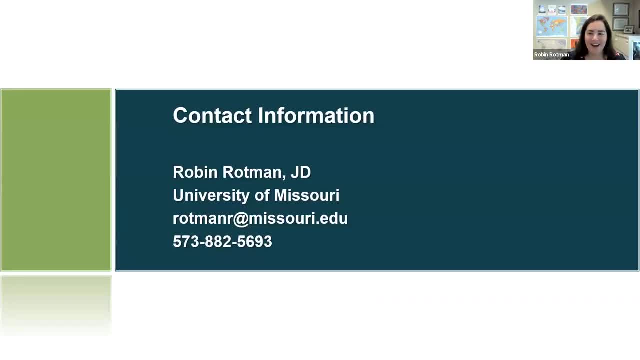 so that's all i've got. i really appreciate your time and attention today and i look forward to speaking with you in the q a. all right, robin, thank you very much. before we move over to jonathan, i do want to ask two quick questions for you all, okay? so first we took a look at the poll and we're gonna 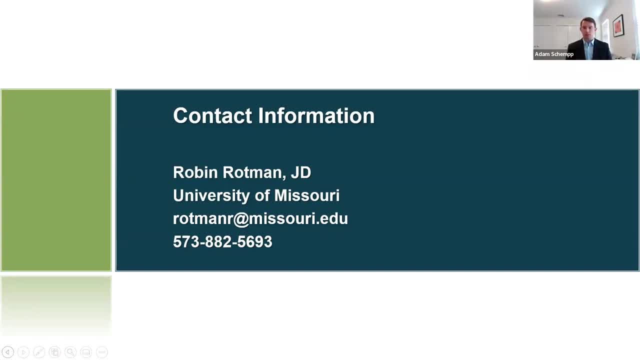 have a lot of questions and we're gonna get to your answers. so if you could take a look, so i'm gonna questions that came in and, by the way, thank you everybody for the questions that you've been submitting. uh, several of them are are lengthier. we won't get into that yet. we'll save them for. 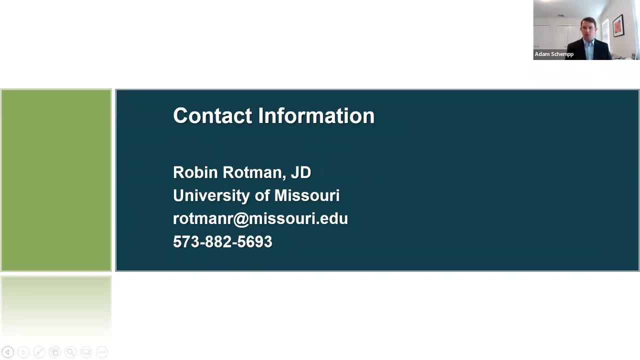 the full q a, but i have two that are more clarifications that i think could be helpful to cover right now. one of them you saw: uh, how do combined sewer and uh, combined water and sewage systems in cities like kansas city, missouri, pollute our river when there's flooding or is? 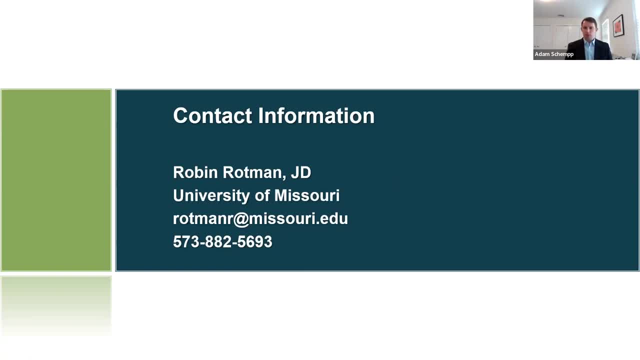 there anything? uh, sorry, uh, yeah, i think i think i know where jayla's going with this. um, so this question is about combined sewer overflows. uh, so i i wouldn't necessarily say um sewage and water system, but it's two different kinds of sewers in the same system. so the sanitary sewer, which is 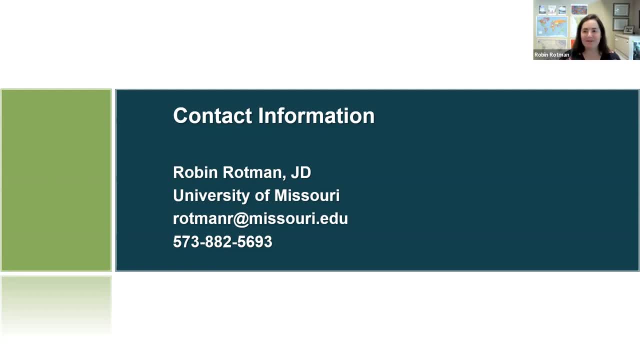 like the sewage collection from our toilets and the things we flush down the drain, um, as well as the stormwater, which is the rain that runs off of the river, uh, you know parking lots or roof surfaces during rain? um. so cities like kansas city, missouri, um, especially older cities, have a 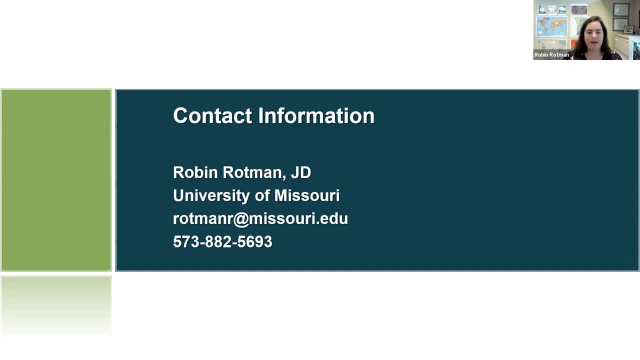 combined system where the sanitary waste as well as the stormwater runoff ultimately go into one sewer. uh, that feeds the wastewater treatment plant, but when it rains heavily, um all that volume exceeds what the waste treatment plant can handle, and so that's why we're talking about combined sewer overflows, um. so in some cities now there's like holding pens- at washington dc, a great example, where they built these underground storage tunnels- um. but in some cities they they just don't have the capacity for this water and it just gets discharged and the effect is after. 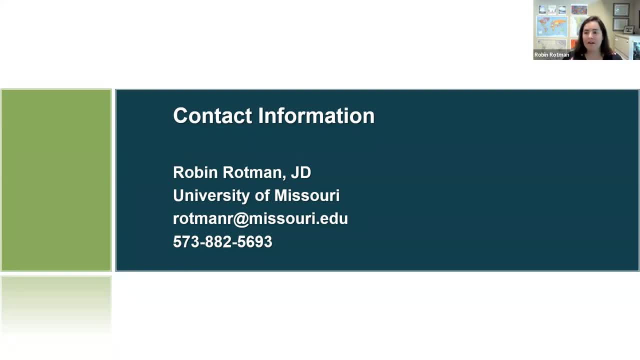 a rain, you could have raw sewage in the environment. um, as to the? as to the question, uh, let me try to see if this is what jayla was going at. so, absolutely a problem to solve, because this requires long-term investment in new infrastructure and a lot of cities like 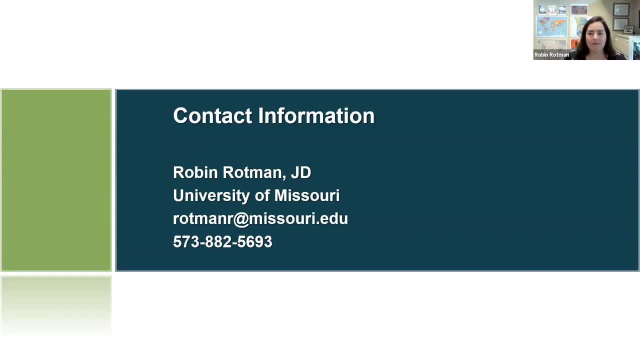 kansas city, also like st louis, missouri, um, don't have that money all up front, and so they have worked out what's called a consent decree with the epa and with the state regulator. so in this case the missouri department of natural resources. that basically says like: okay, look, we know it's a. 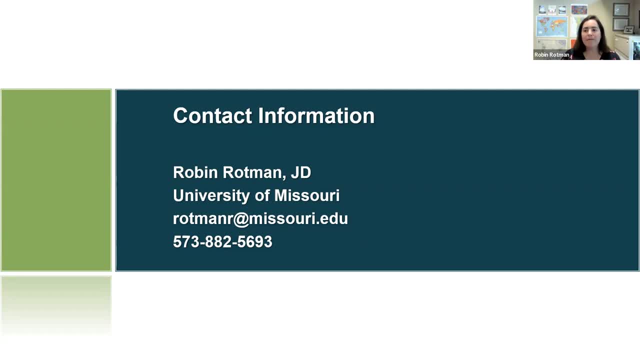 problem. we can't fix the problem overnight, but we're committing to make certain investments every year in order to generate certain improvements in water quality in the long term. so i hope that it kind of explains how the combined sewer overflow process works. and just to clarify: i think originally the concept of a combined sewer made some sense, because then you were treating your storm water before it went back into the system. it wasn't just flushing everything off the streets, but the problem comes when you get heavy storms, which unfortunately, we're getting more and more of. absolutely the other question i want to ask quickly before we move to jonathan, is: 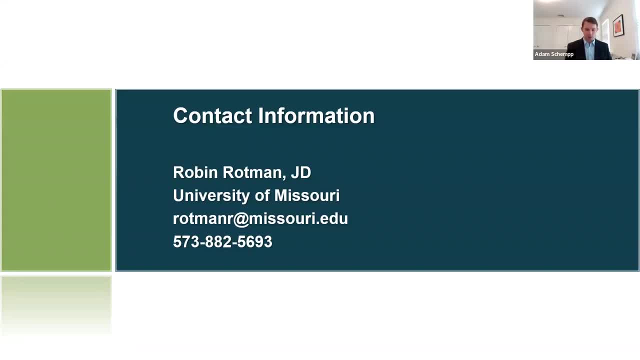 uh, why wouldn't states allow the federal government to bear the cost of regulation? this goes back to your point about delegated authority. why wouldn't 402, et cetera? um, so is is what the is what the question is. hey, it costs a lot of money to actually operate a clean. 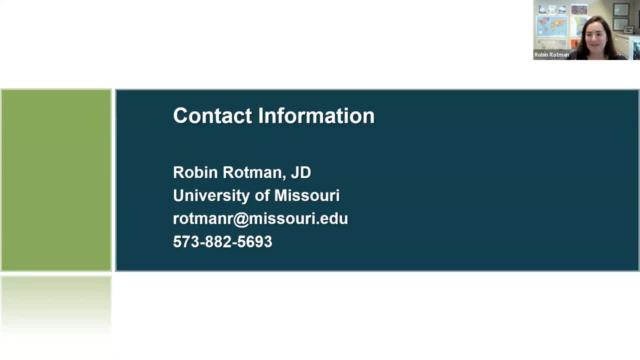 water program. um, like my, my first job out of law school was here in missouri, in the missouri department of natural resources, which is the clean water act permitting agency for the state, and so we had a whole team of permit writers and standard setters and inspectors and enforcement people in 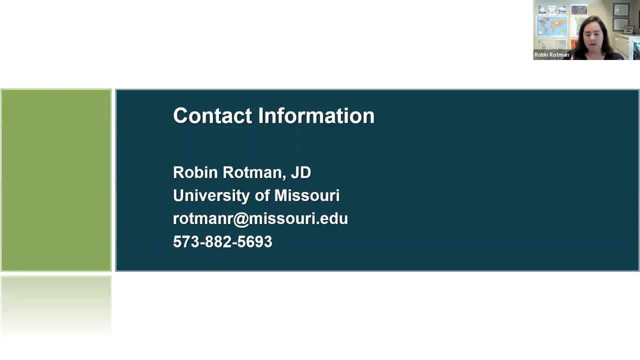 it. um, that is a real cost that the state incurs. well, i can say some reasons why i think in missouri they made that choice, and perhaps why other states did as well. um, one, um, it is possible to recover some of those fees through through permit fees. so, um, if you apply for a permit, that 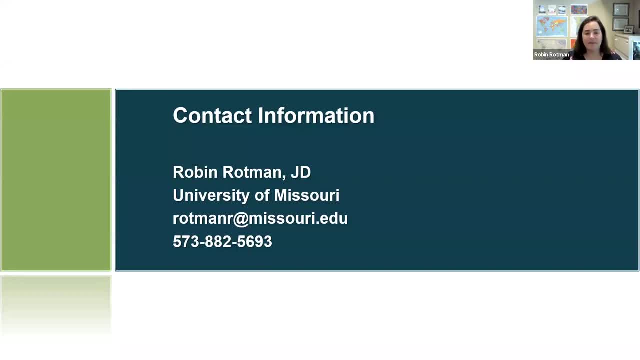 is not necessarily a free or even a cheap process, so some of those fees can be recovered um. secondly, there's a notion that the local personnel have a better understanding of local issues and are going to do a better job um treating local people in a fair? uh and efficient. 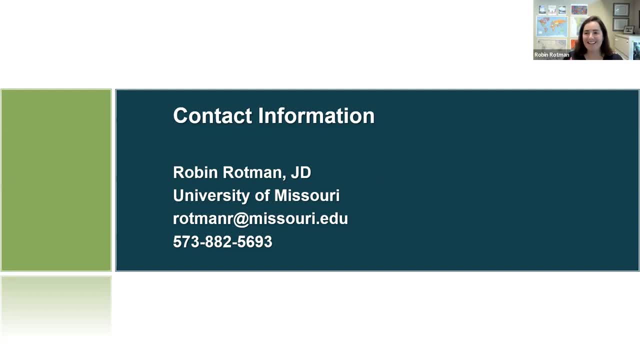 manner. um, there's a sense that you know, like those big old bureaucrats back in washington, like they're just so disconnected from what's happening on the ground, how could we trust them to be handling this issue? you know, up in some rural county in missouri. now you could debate whether that is sound policy making or not, but i think that that 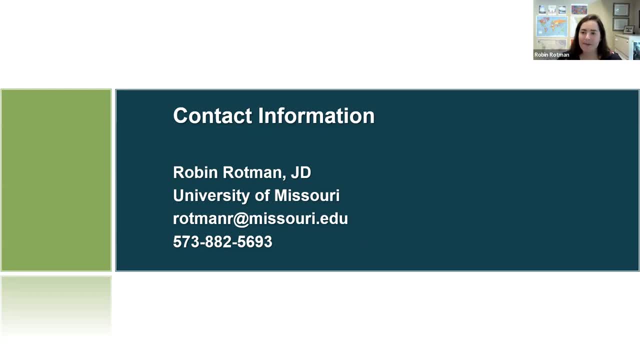 line of thought is common in most states, which is like it's better for us to handle these issues locally and not have the epa so involved. and i would just quickly add to that: i think a lot of it comes down to that authority. we would like to do it, we want to have that back, that power, that 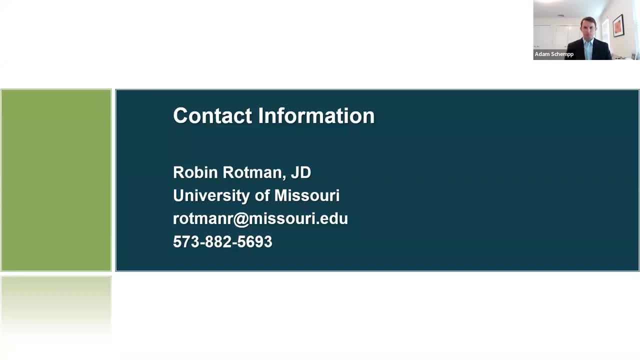 control and going back to your point about tribes, there are about around 50 tribes that currently have water quality standards, settings um, and as we're building that up, i wanted to take a question that we have developed for you from you in general: the development in fairest in the midwesterly states. you know we we've got a lot of resource in there for us, but this is the most important part of the project, so we wanted to bring those to the table. we would like to bring those to the table, to the table overall. you know we've got a. 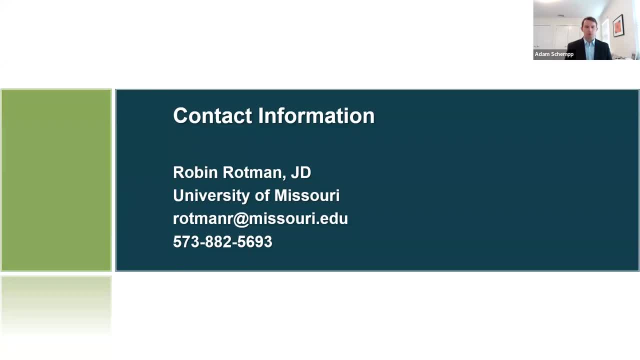 setting authority. About three years ago, the EPA developed guidelines for states or for tribes to be able to have clean water 303D authority. No tribes have yet sought that And I think it is very much. this balance of what's it going to cost, What are the expectations on us going to be? 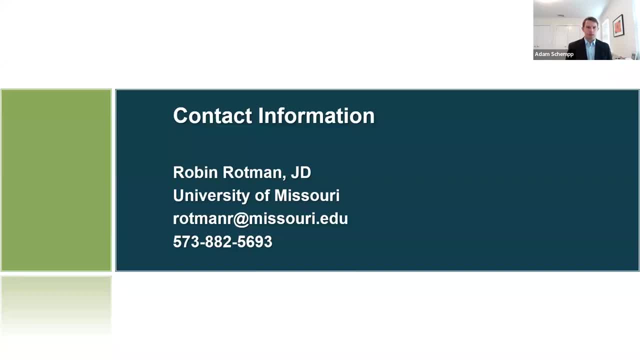 versus what are the benefits and authorities that we will be getting out of it. And it is very much that balance And I think a tricky issue with tribes is: I mean, tribes are sovereigns that existed as sovereigns before the United States government existed, But the Clean Water Act, 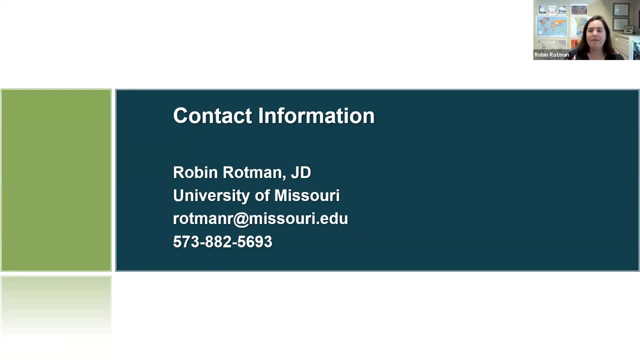 doesn't necessarily always reflect that reality, And in order for a tribe to get this treatment of state status, basically it has to prove to the EPA that it has the infrastructure in place to implement that, And I think that's a really important point, And I think that's a really 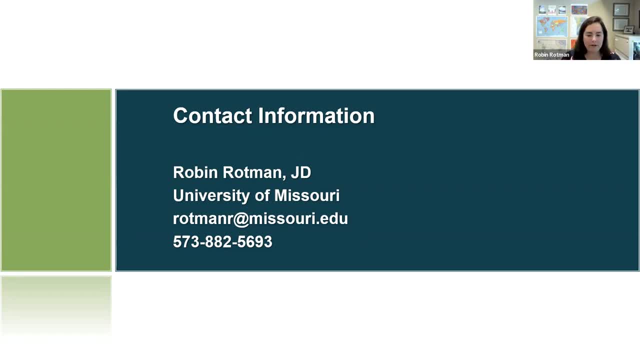 important point And I think that's a really important point And I think that's a really regulatory program. So it has internal governance, it has staff who are appropriately trained and the EPA provides some funding in order to build that capacity. But it's quite a long and 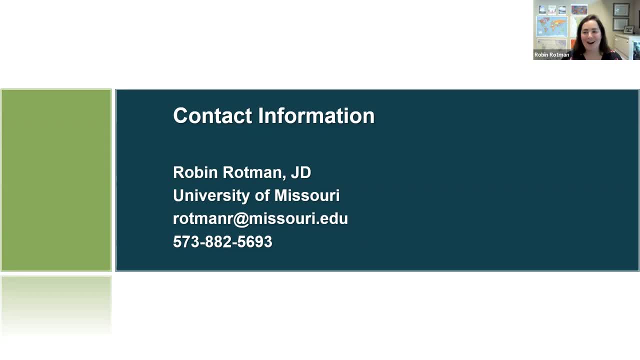 onerous process to prove to the EPA that a tribe is ready to assume that authority. So I'm not surprised that if a new authority was issued three years ago, even if some tribes have begun that process, the paperwork is probably still underway. 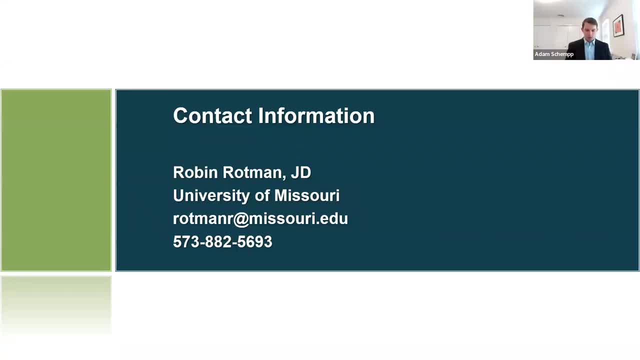 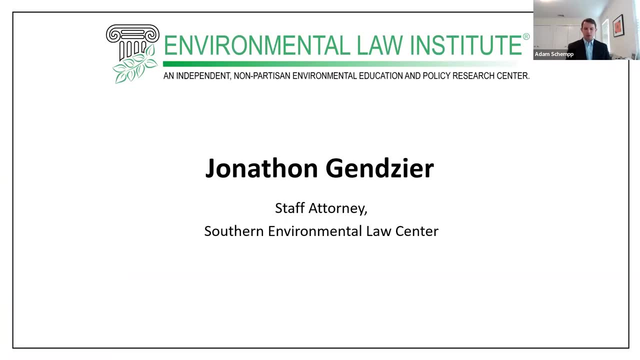 Thank you very much, Robin. I would now like to turn things over to Jonathan Genzier, who is a staff attorney with the Southern Environmental Law Center in Charlottesville, Virginia. Jonathan primarily works on water-related issues. This has included coal ash, including two Clean Water Act. 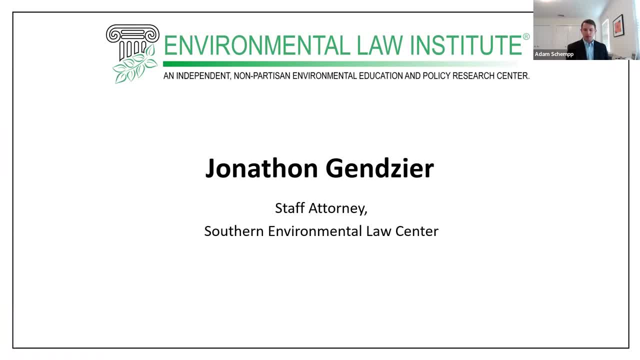 citizen enforcement cases that went to trial, and interstate gas pipelines, including the now canceled Atlantic Coast Pipeline. His work currently focuses on water quality in Virginia and Federal Clean Water Act regulatory matters, including rulemakings on waters of the US and Section 401 certification, which are the focus of his remarks today. Jonathan received his law. 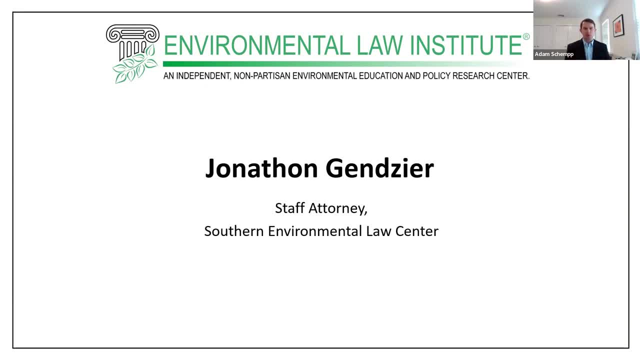 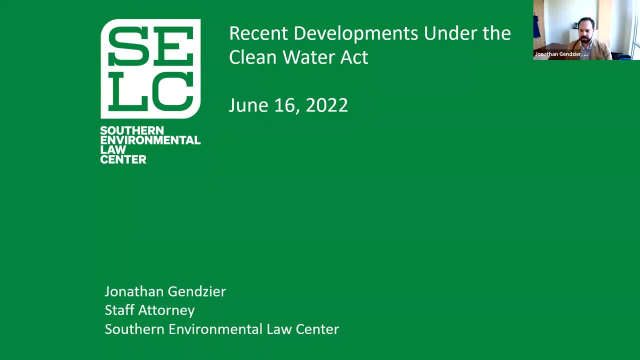 degree and bachelor's degree from Vanderbilt. and with that, Jonathan, the floor is yours. Thanks, Adam, and yeah, thanks to ELI for having me here today. When I was in law school, I worked on the Environmental Law and Policy Annual Review which ELI publishes with Vanderbilt, so it 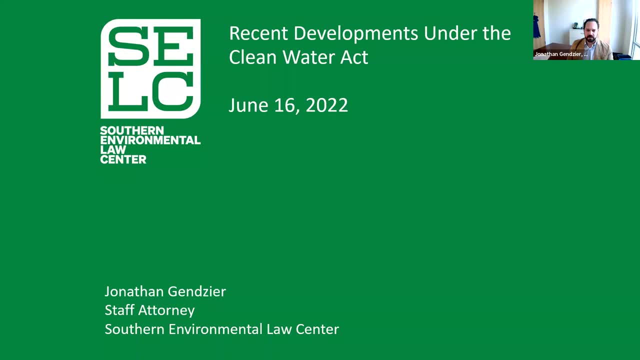 feels great to be here. Thank you. I'd like to just tell you a little bit about SELC to start off. We're a non-profit law firm that represents conservation and community organizations. We work in six states in the South- That's, Virginia, the Carolinas, Georgia, Alabama and Tennessee- and we've been involved. 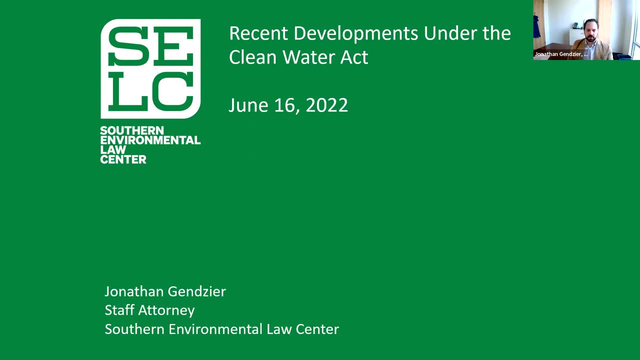 in litigation over the scope of waters of the US and are advocating for strong federal clean water protections that are going to be used in the future. So I'd like to start off by starting with the Clean Water Act, which is a definition of the Clean Water Act, As you know. 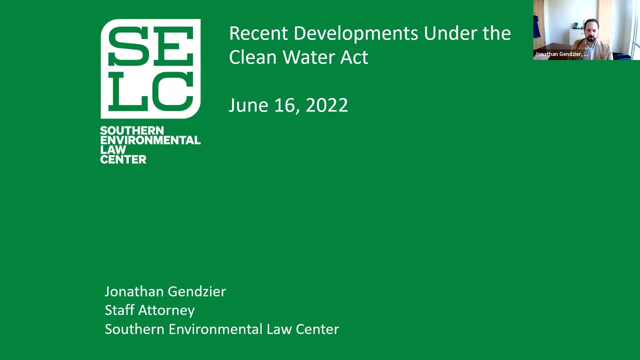 the Clean Water Act is an act that is implemented by the United States, and that's the full purpose of the Clean Water Act, which is to ensure that our communities are consistent with the goal of the Clean Water Act: to restore and maintain the nation's waters. Next slide, please. 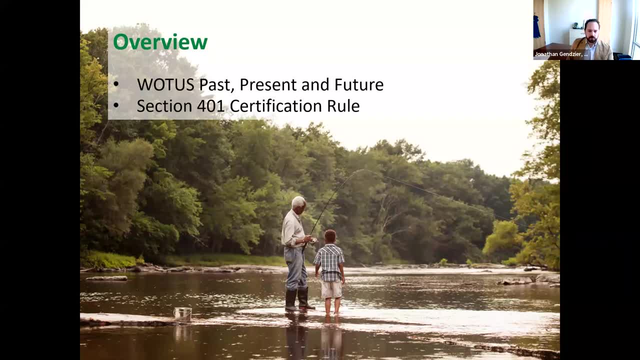 So just to give you an overview of what I'm going to cover, as has been mentioned. so I'd first just like to discuss why the Clean Water Act's definition of waters of the United States, or WOTUS, matters, and then I'll walk you through the evolution of WOTUS through the various agency rules. 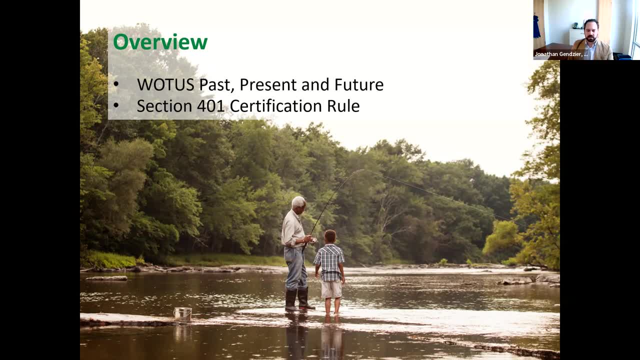 that have been implemented in the United States, and in the United States and around the world. I'd like to start with the Clean Water Act, definition of the waters of the United States, or WOTUS matters- to find that term- and then talk about where we are today. 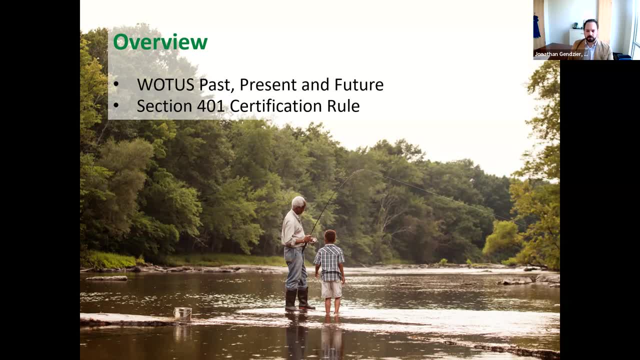 which is awaiting finalization of a jurisdictional rule proposed by the Biden administration, And I'll also touch on legal challenges to the prior administration's navigable waters protection rule, the status of the pending litigation on that and just what to expect from the Biden administration. 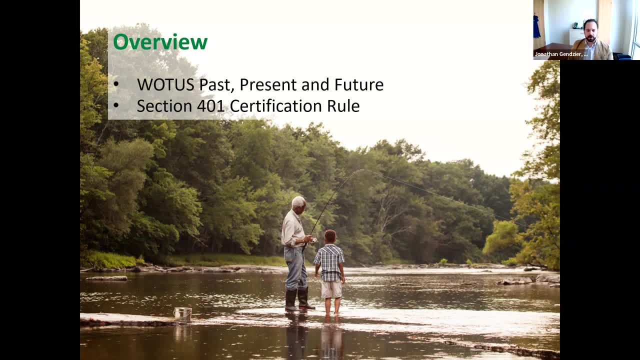 And then I'd also like to discuss proposed changes to the Section 401 certification rules under the Clean Water Act. give a brief overview of the ongoing litigation there, as well as the recently proposed 401 certification rule. Next slide, please. So why do waters of the US matter? 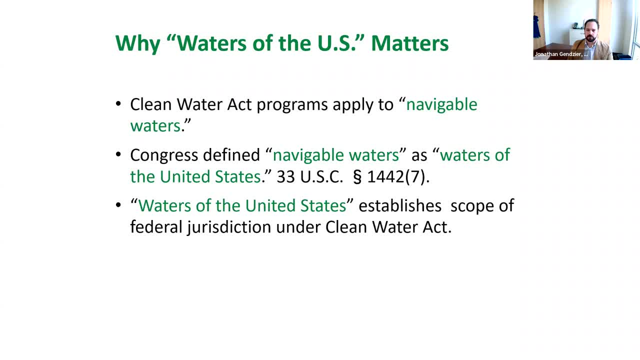 Why does the definition of that term matter- And I think you got a great preview of this from Robin. So waters of the United States is really a threshold term in the Clean Water Act. it establishes the geographic scope of the act: what waters and wetlands the Clean Water Act protects. 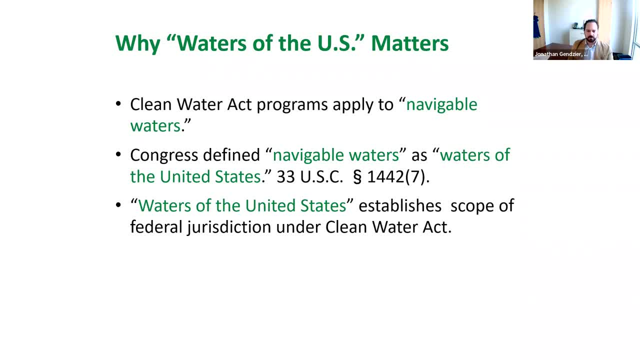 So Clean Water Act regulatory programs address navigable waters which the statute defines as waters of the United States. It doesn't define that term. it leaves that to EPA and the court to define. But that statutory term is the jurisdictional linchpin. 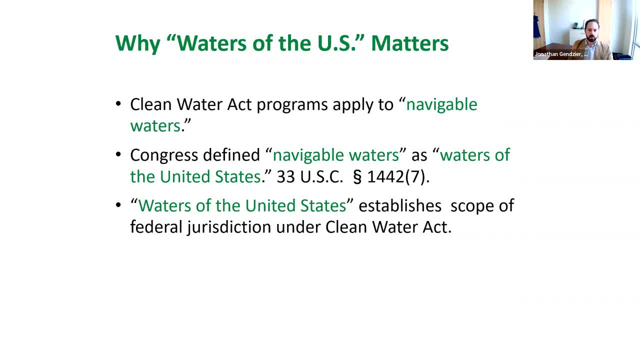 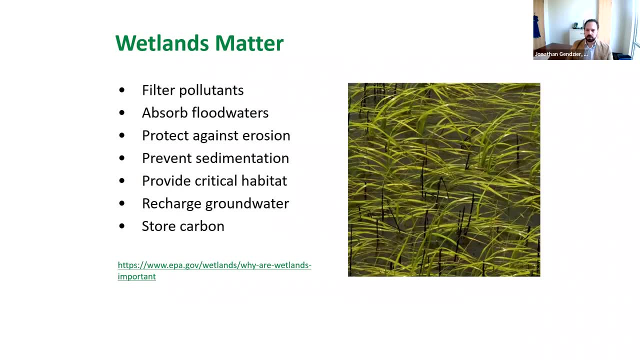 for just about every one of the critical safeguards for water quality That is contained in the Clean Water Act. Next slide, please. So why does that matter? Well, if you think about wetlands, they provide a lot of services that are quite important. 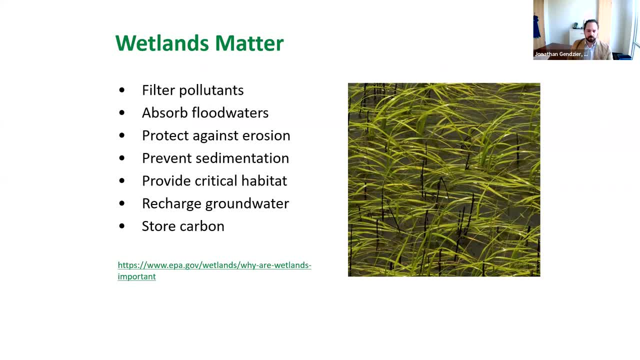 They filter pollutants. they act as a sponge and absorb flood waters. They counteract surface water runoff and sedimentation. They protect the coast from erosion. They're nurseries for a lot of species, providing habitat. they recharge groundwater supplies. So both locally and within the context of a watershed. 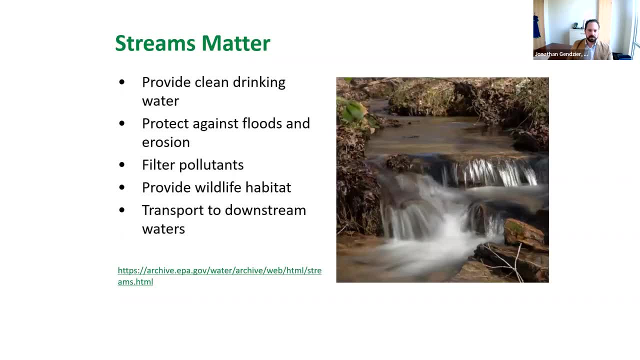 wetlands are quite important. Next slide Streams as well, So including headwater streams. there are intermittent streams that flow only part of the year, ephemeral streams that flow in response to precipitation. These provide many benefits as well. Some are similar to the functions of wetlands. 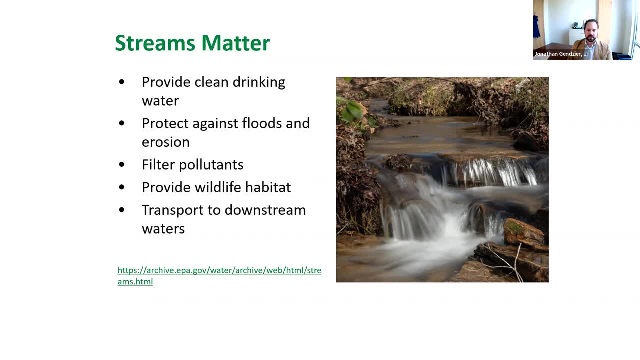 protecting against floods, filtering pollutants, providing habitat. They also transport water and sediment and organic matter and nutrients, as well as pollution, to downstream waters, And so the biggest rivers that we are all familiar with are only as healthy as what flows into them from upstream. 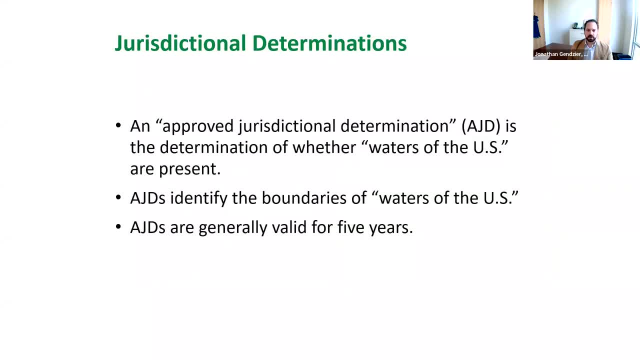 Next slide, please. So, and just to introduce another concept, a jurisdictional determination is a determination. a jurisdictional determination is a determination is a determination by the EPA or by the Corps of Engineers whether a given project site has waters of the United States present on site. 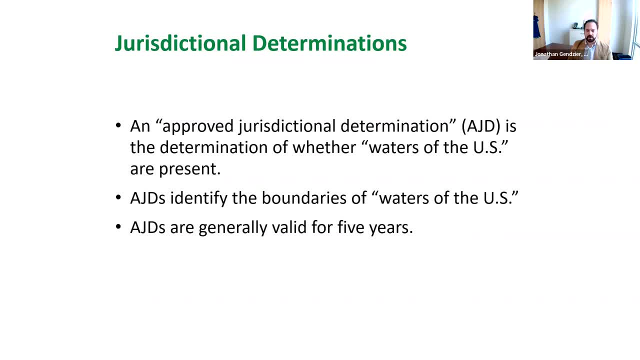 And these decisions are generally good for five years. So once you have your approved jurisdictional determination, you have a sort of a safe harbor for pollution or destruction of non-jurisdictional waters as set out in that determination, regardless of regulatory. as set out in that determination, regardless of regulatory. 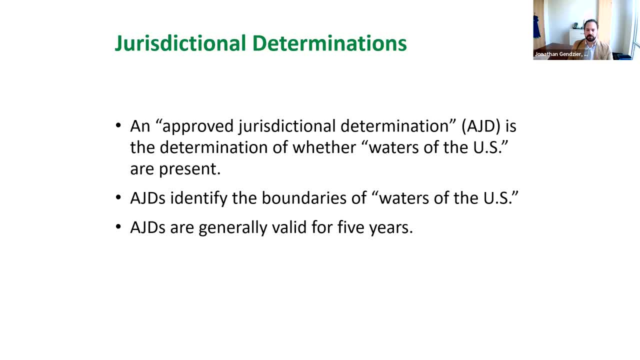 as set out in that determination, regardless of regulatory changes. So even if the definition of WOTUS changes within five years, So even if the definition of WOTUS changes within five years, you've sort of locked in the impacts that are set out there. 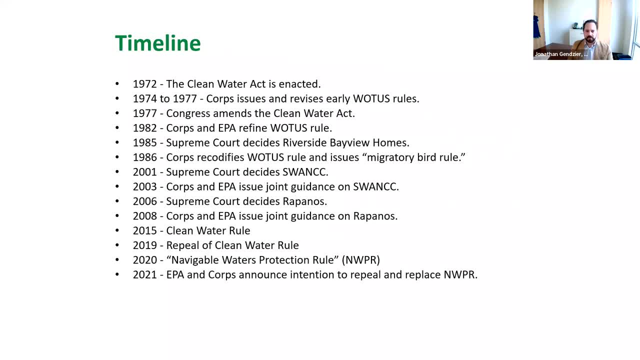 Next slide, please. So as this timeline shows the scope of the waters, which includes wetlands that have been subject to Clean Water Act. jurisdiction has really ebbed and flowed over the years, with changes in administrations and with Supreme Court. So as this timeline shows the scope of the waters. 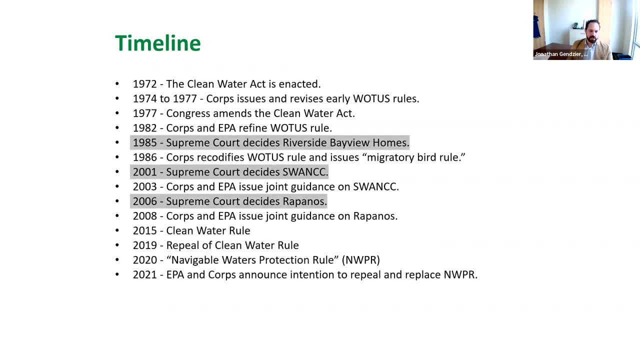 which includes wetlands that have been subject to Clean Water Act. jurisdiction has really ebbed and flowed over the years, with changes in administrations and with Supreme Court decisions. Next slide, please. So beginning with the enactment of the Clean Water Act in 1972,. 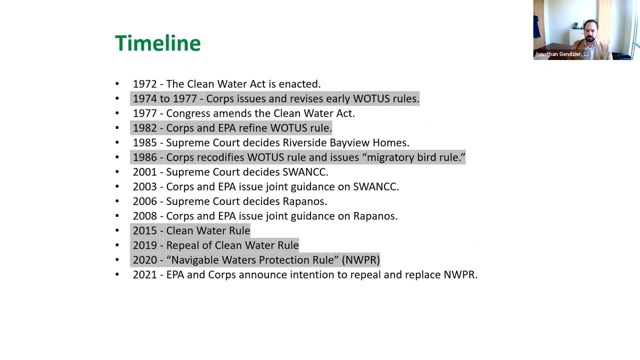 So, beginning with the enactment of the Clean Water Act in 1972, the Corps and EPA have defined waters of the United States by regulation by regulation. There has been ensuing litigation over the application of those rules, as well as responsive Supreme Court decisions. 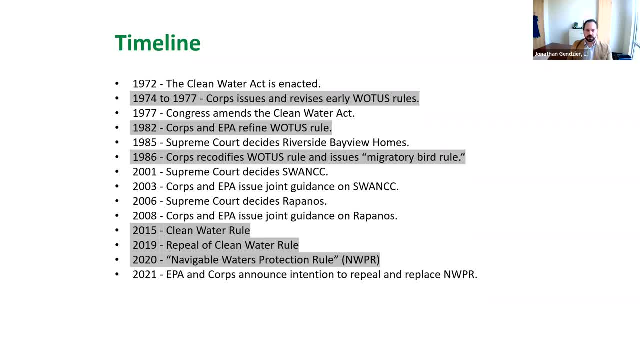 of those rules, as well as responsive Supreme Court decisions and regulatory changes. So, in the interest of time, I'm not going to do a detailed review of the waters. So, in the interest of time, I'm not going to do a detailed review. 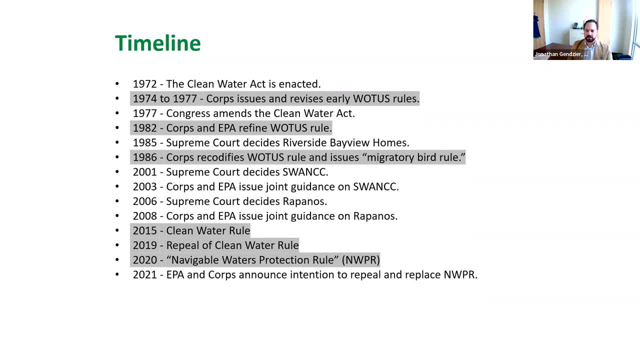 a deep dive into every aspect of this, but it does give you a sense of the history here. Next slide, please. So there are really three key Supreme Court decisions that you know. if you've taken environmental law, you have likely heard of. 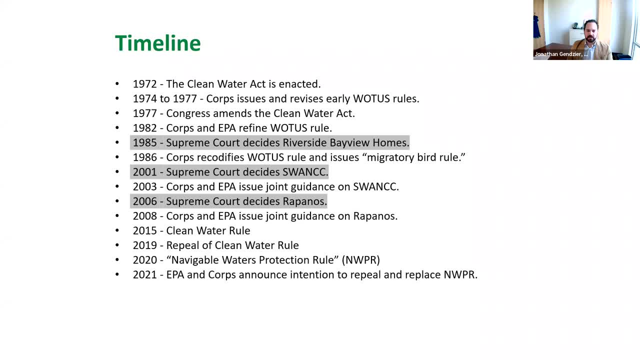 And those are Riverside, Bayview Homes, Swank and Rapanos, And these have been really critical as the definition has ebbed and flowed over the years. Next slide, please. And the agencies have responded to these Supreme Court decisions in between rulemakings by issuing guidance as well. 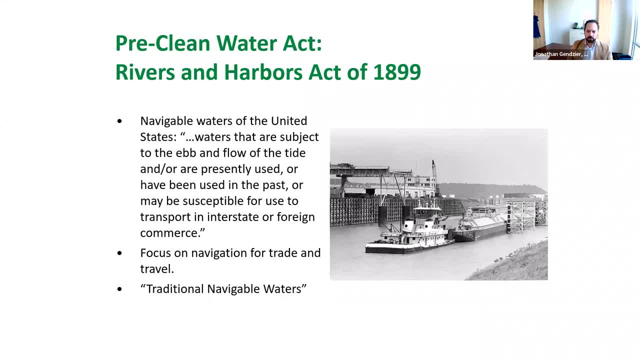 Next slide, please. So- and you know Robin covered this very well- The focus of the pre-Clean Water Act laws that focused on navigability was really preserving the navigability of the nation's waters for commerce, And by navigable they really meant navigable. 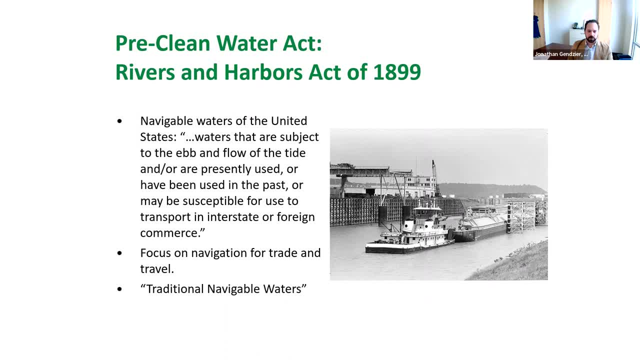 The water had to be currently used for transport, or historically used for transport, or potentially could be used for transport in interstate or foreign commerce, And so that definition is that refers to what you'll hear, you may hear me refer to as traditional navigable waters. 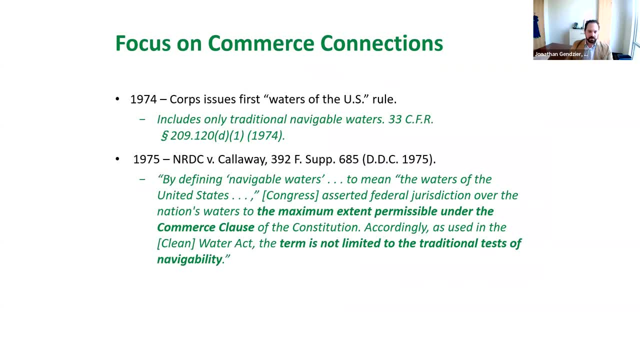 Next slide, please. After the 1972 Clean Water Act, the core issues that were the most important. you know the first waters of the US rule and this limited jurisdiction to traditional navigable waters only. So you know those main stem rivers and lakes and the oceans that could be. 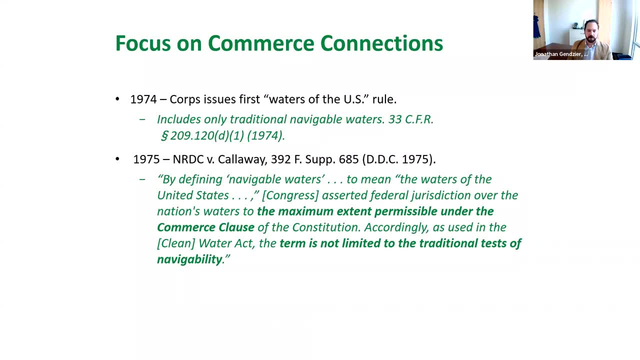 plied for commerce, And so environmental groups considered this definition to be too narrow, And so the Natural Resources Defense Council sued the Corps of Engineers, And in a 1975 decision the court agreed that jurisdiction was not limited by the traditional test of navigability, but that Congress intended jurisdiction under the Clean Water Act to extend. 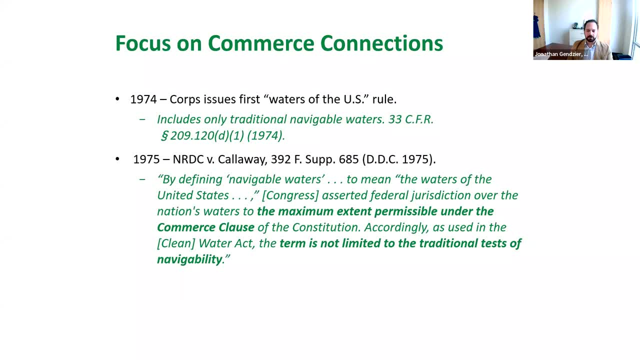 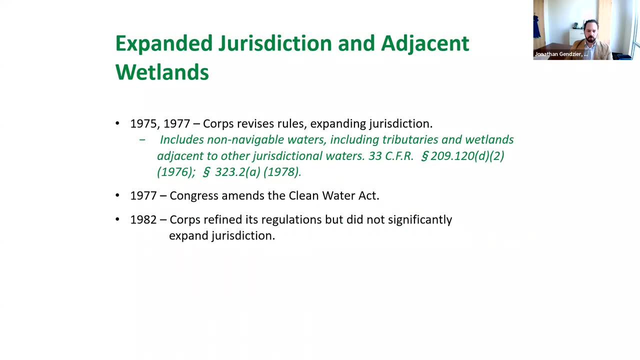 to the maximum extent of Congress's Commerce Clause authority. Next slide, please. After this, the court amended its regulations, And the then later Congress amended the Clean Water Act in 1977. And so there was further debate in Congress about the extent of the scope of the Clean Water Act. 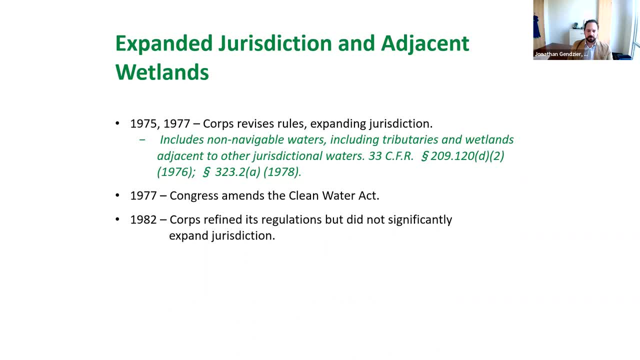 And I think it's notable that Congress did not limit the definition of navigable waters or waters of the United States And it didn't otherwise reject the Corps' expanded regulatory definition. post Callaway In 1982, the Corps refined its regulations yet again. 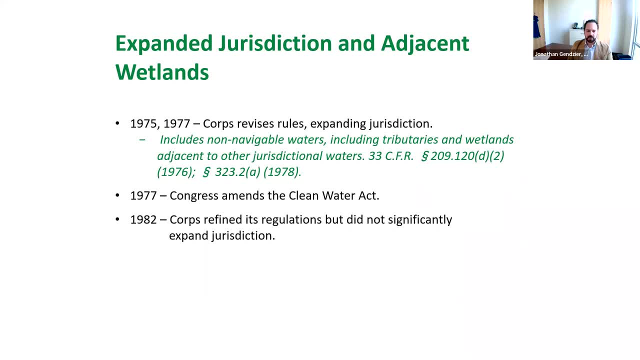 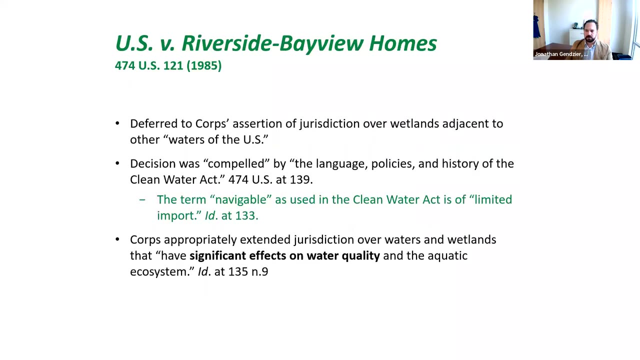 It didn't significantly expand jurisdiction there, but it did add some exclusions, some of which remain today, like the exclusions for normal farming, silviculture and ranching practices and for water treatment systems. Next slide, So the first of these three Supreme Court cases. 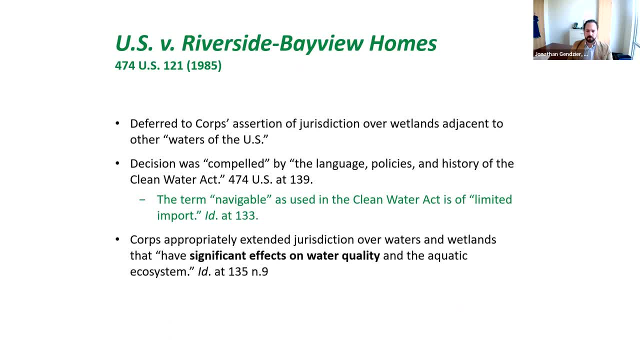 began because a housing developer placed fill in preparation for constructing homes in 80 acres of marshland. So the first of these three Supreme Court cases began because a housing developer placed fill in preparation for constructing homes in 80 acres of marshland, which is near the shores of Lake St Clair in Michigan. 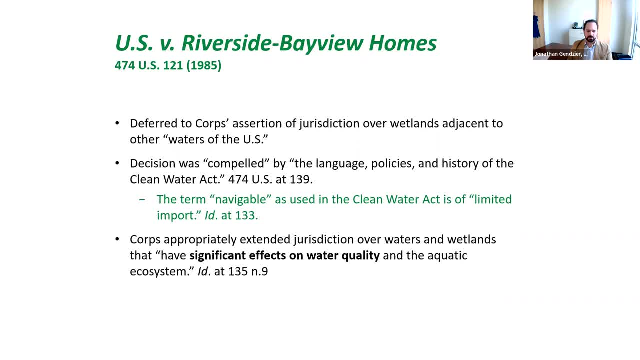 Which was, you know, which is usually called a, that the wetlands did not receive frequent flooding by nearby navigable waters and so were not jurisdictional, And in a unanimous decision the Supreme Court reversed the Sixth Circuit And it agreed with the Corps that the Corps had jurisdiction over the wetlands. 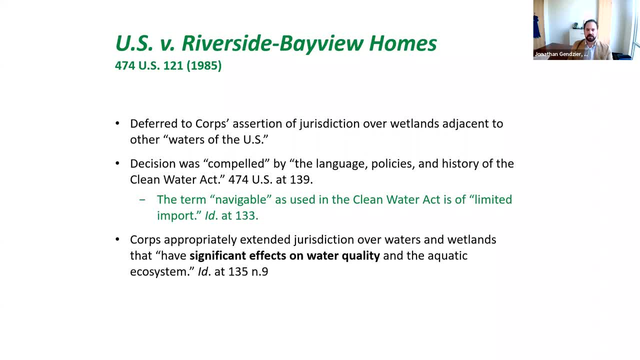 The court said that the term navigable, as used in the Clean Water Act, had what it called limited import, And so the court described its decision, though, as being compelled by the language and the policies and the history of the act, And this was the first place where the Supreme Court came out with what would later be referred. 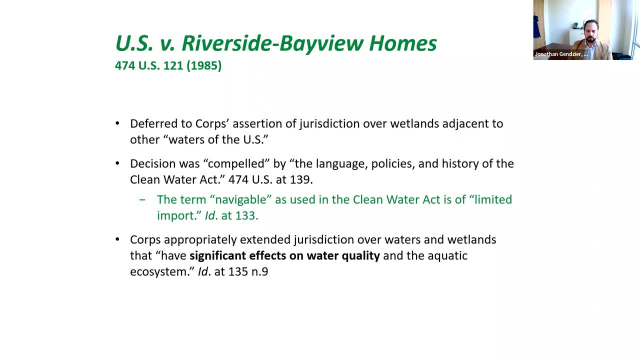 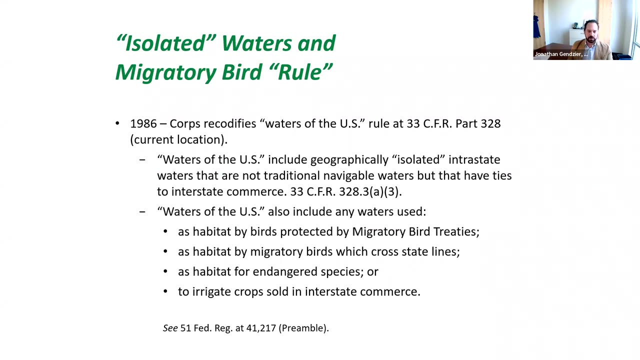 to as the significant nexus test, where the court appropriately asserted jurisdiction over wetlands with a significant effect on water quality and the aquatic ecosystem. Next slide, please. So in that recodification in 1986 by the court it included what the agency called a clarification. 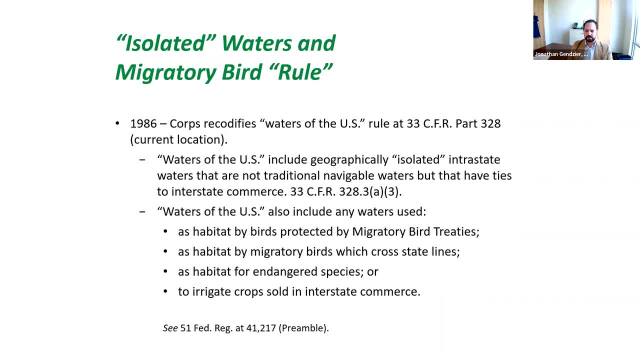 that waters of the United States actually included waters used as habitat by migratory birds that cross state lines or are protected by the Migratory Bird Treaty Act, And so you can see that commonality. You can see that there's a lot of commerce connection here, and so this was sometimes 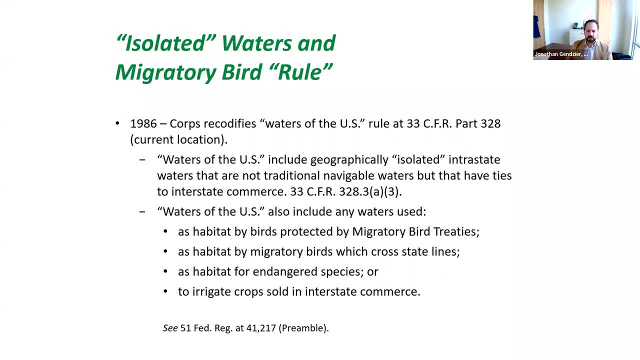 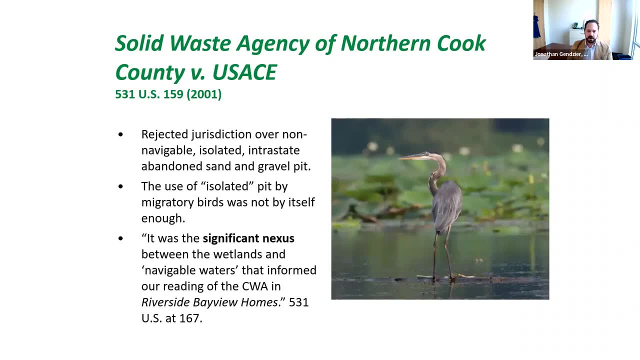 called the Migratory Bird Rule and it was an issue in the in the next Supreme Court case. Next slide, please. So this solid waste agency of Northern Cook County, Shorthand Swank, involved an attempt to build a waste facility on an abandoned sand and gravel pit in northern Illinois. 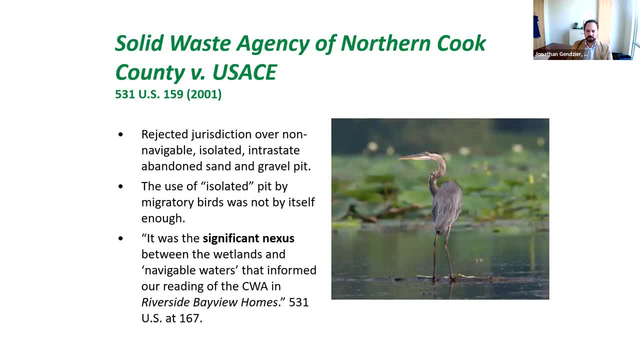 And I think it's worth noting. the pit was not navigable, It didn't cross state lines, It was not adjacent to another jurisdictional water, It was geographically isolated and, under the Migratory Bird Rule, the court asserted jurisdiction and denied the application for a permit. 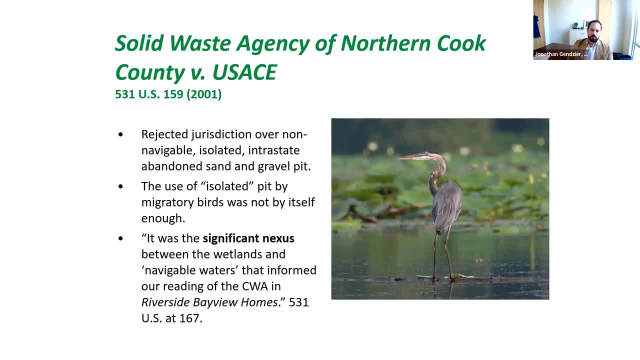 And so this eventually reached the Supreme Court, which, in a 5-4 decision, rejected the court's assertion of jurisdiction because it rested solely on the fact that the pit was used as habitat for migratory birds. The Supreme Court said that that was not the case. 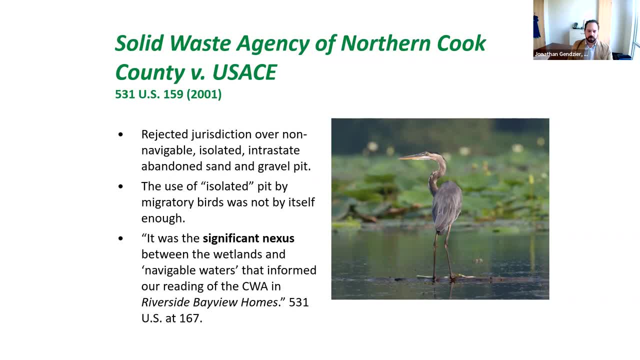 that that by itself was not enough and it reiterated that the significant nexus between wetlands and navigable waters was what had informed its reading of the clean water act in in the riverside case, and it found that that nexus just was not present here. next slide, please. 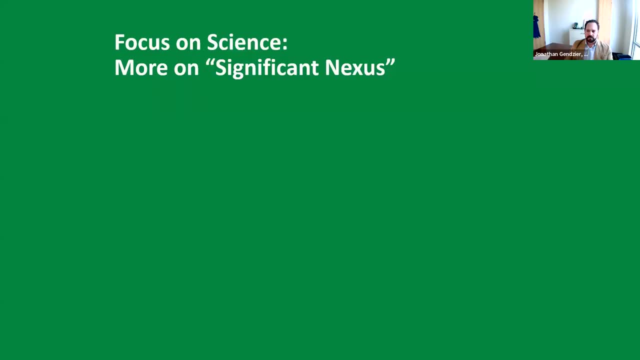 so, just in the interest of time, we'll go ahead one more slide. so as we've moved into the 2000s, the agency started to focus more on science, updated scientific knowledge and and learning more about what it means for water to have a quote significant nexus. next slide, please. 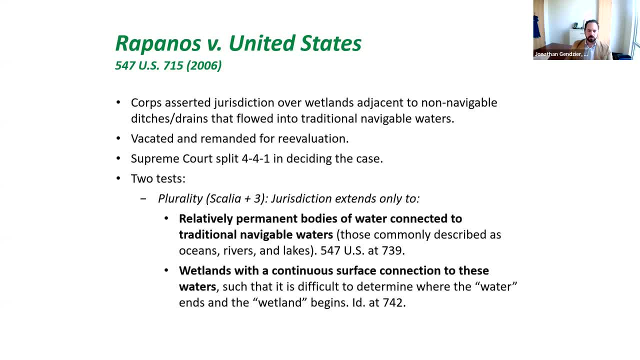 so, um, to date, this is the most recent supreme court decision, uh, on waters of the united states or upon us, and it arose from two consolidated cases. in both of those cases, the core had asserted jurisdiction over wetlands at issue, not not because they were adjacent to traditional. 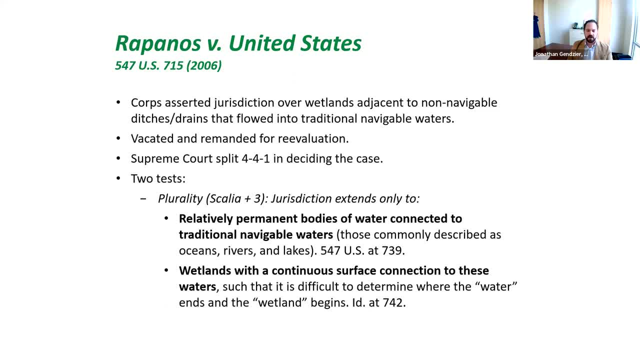 navigable waters, but because they were adjacent to non-navigable tributaries of navigable waters, so sort of one step removed from being adjacent to navigable waters. and in both of these cases jurisdiction under the clean water act was upheld by the district court and by the sixth circuit, and so the opinion here is, uh is fractured. 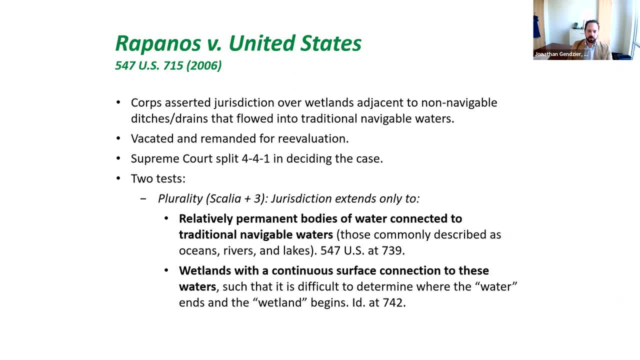 the court did vacate the lower court decisions upholding jurisdiction and it remanded both of these cases to the core for reevaluation under the 1980s regulations and consistent with the courts- uh, with the court's opinion. but two tests for jurisdiction arose from rapano. so first, 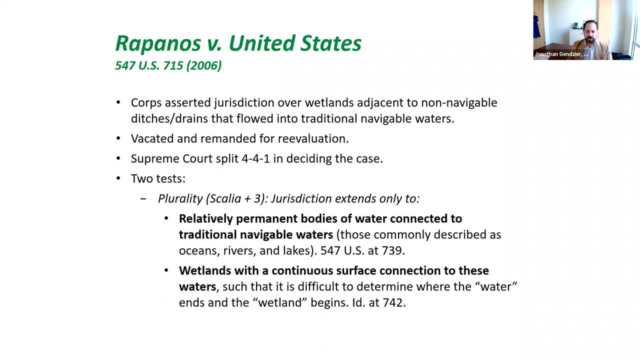 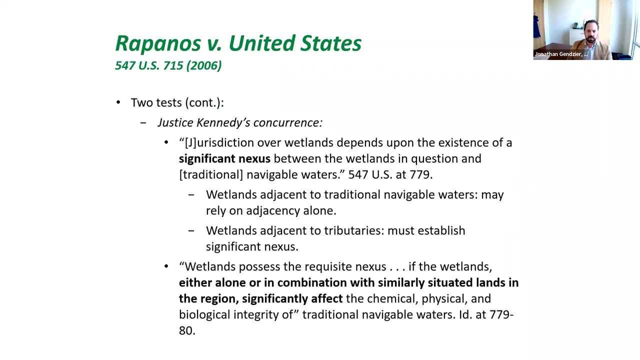 in the plurality uh led by justice scalia. their test covered only relatively permanent waters that are connected to traditional navigable waters and wetlands that have a continuous surface water connection to those waters. next slide, please. in contrast, the second test was announced by justice kennedy in a concurrence which built on the past two cases. 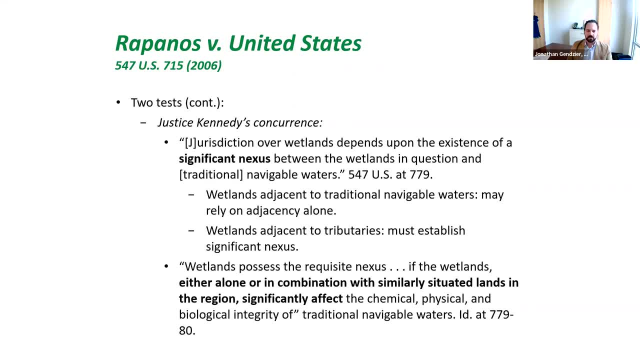 that we talked about and extended jurisdiction to non-adjacent or geographically isolated wetlands with a significant nexus to traditional navigable waters. so for a wetland to possess the requisite nexus for jurisdiction, either alone or in combination with- uh, with what justice kennedy calls similarly situated. 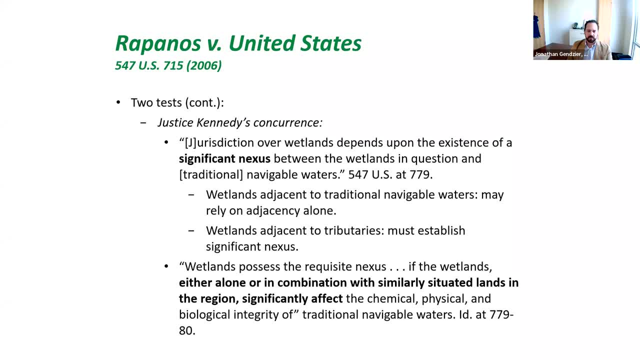 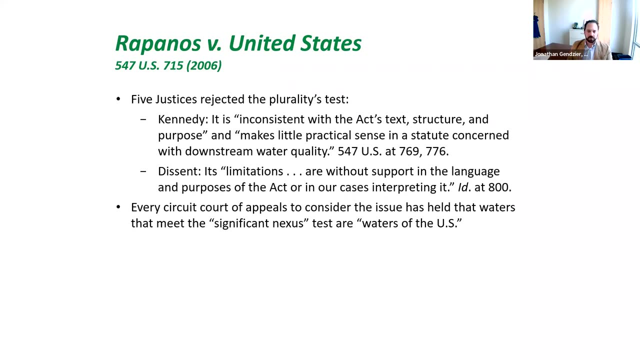 wetlands in the region has to significantly affect the chemical, physical and biological integrity of traditional navigable waters. next slide, please. so although the four dissenter's in this case would have actually affirmed clean water act jurisdiction, they agreed with justice kennedy that the plurality opinion was inconsistent with the text and the structure and the purpose of. 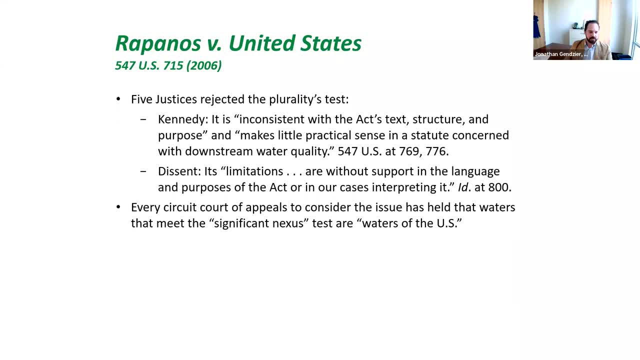 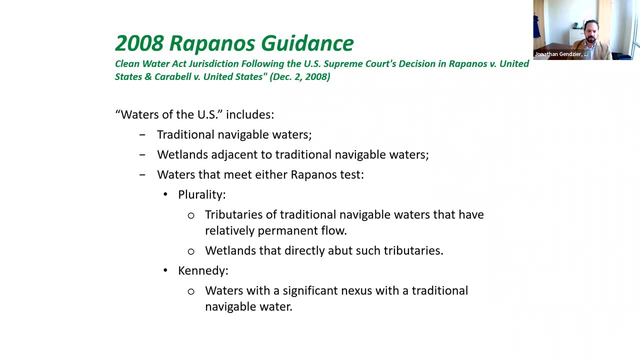 the clean water act. um next slide, please. so, after ripanes, the agencies issued guidance to try and apply this decision on the ground, and under that guidance, waters of the united states included traditionally navigable waters, wetlands that are adjacent to traditional navigable waters and the 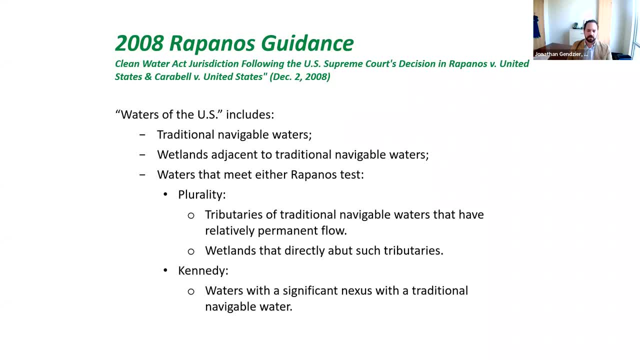 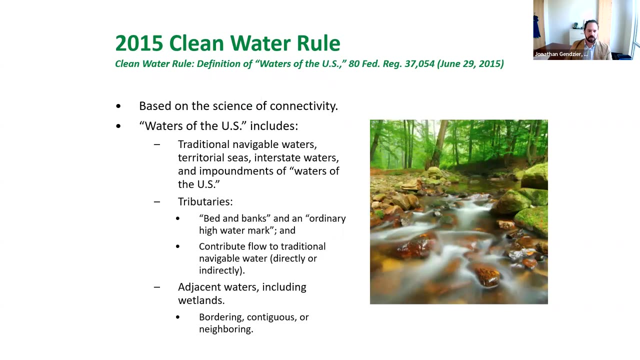 waters that satisfied either of the two jurisdictional tests put forward in the ripano's decision. next slide, please. so, following this, the obama administration promulgated the uh 2015 clean water rule, which was heavily reliant on the signs of connectivity between waters. this was a, a, four. 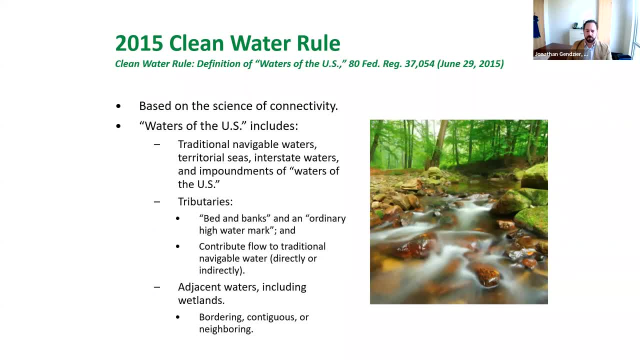 year rule making process. uh, that was affected by the convalescent waters act of 2015, the lots that making process. There was a large empirical record and they used the record to determine which waters satisfied the significant nexus test to mandate inclusion as waters of the United. 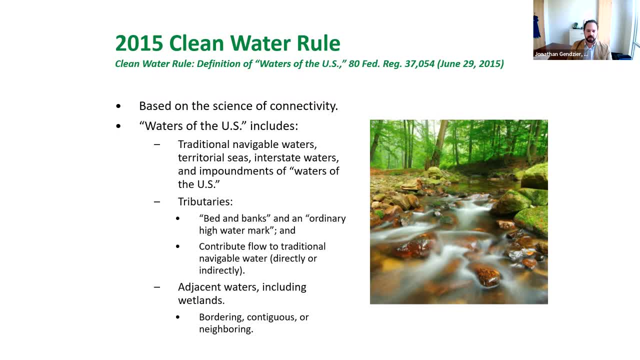 States And specifically the rule identified eight categories of waters that are covered as waters of the United States. So the first three long regulated traditional navigable waters, interstate waters, including interstate wetlands, and the territorial seas, any impoundments of those waters or tributaries of those waters as well. 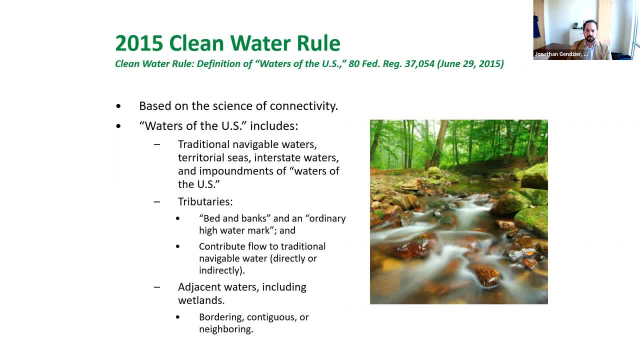 Prior regulations had included wetlands that were adjacent to other waters of the United States and defined adjacent to include bordering, contiguous or neighboring. But the Clean Water Rule included adjacent waters as opposed simply to adjacent wetlands, and it defined waters that were adjacent to other waters of the United States. So the Clean Water Rule. 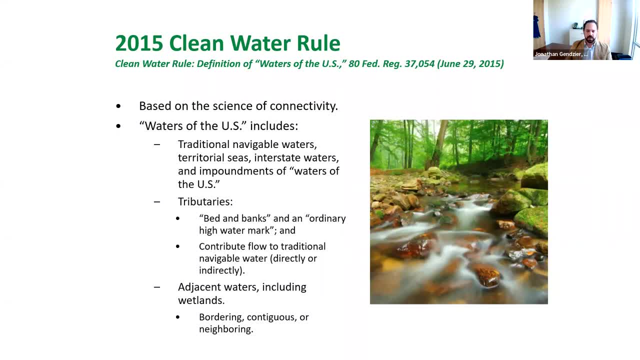 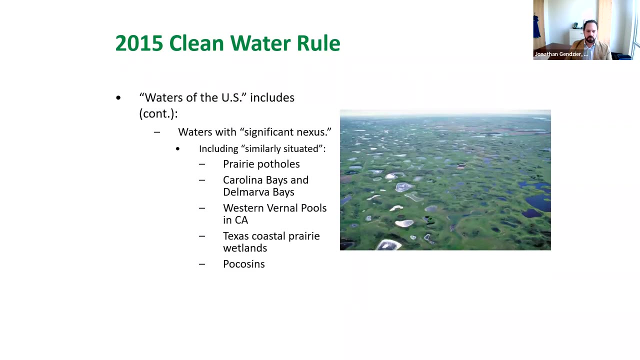 included adjacent waters as neighboring, based on distances between waters and features of other jurisdictional waters, like the 100-year flood plain, the high tide line, the ordinary high water mark. Next slide, please. So the Clean Water Rule also included some basically categorical. 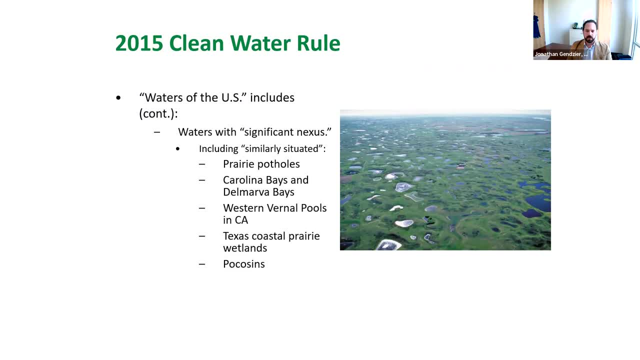 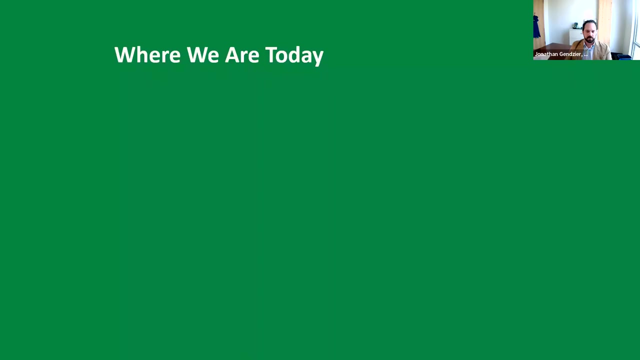 protections where it enumerated certain categories of geographically isolated waters. So the Clean Water Rule included adjacent waters as those. Почему had These Publicities been所? And so these Wetlands were said to be families? heavy participants know that at date 67, there are An cheque term, Leariat by case, to address case-to-case cases. The rules were qualified. Mod 있around resolution made a ought to follow the scenario and sweater policies were requested. So the rule clarified that for the purpose of a significant nexus analysis, those wetlands are similarly situated and should be. 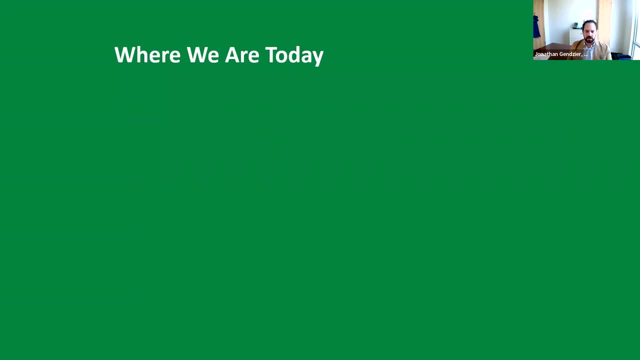 because there were plans for an isolated wetland management complaints. the�� envelop is scene reflected and it yolotl. The Trump administration promulgated the Navigable Waters Protection Rule, which has since been invalidated by a couple of courts. Next slide, please. 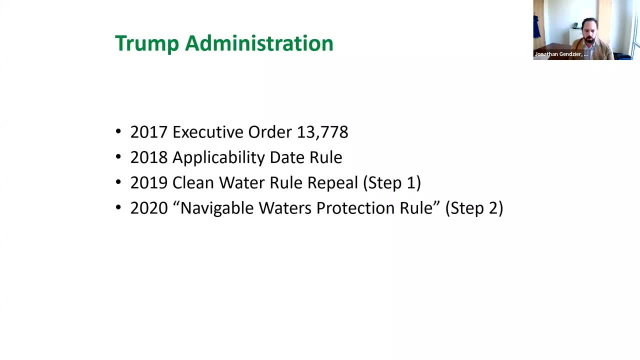 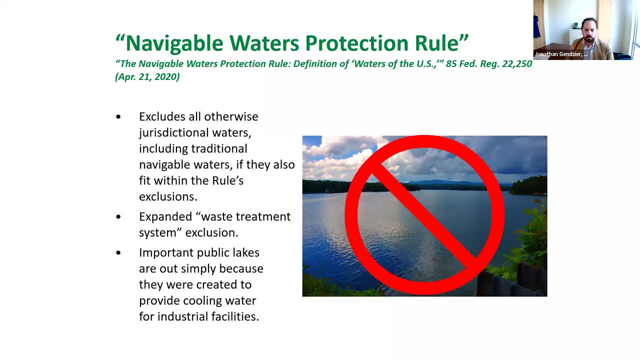 The Trump administration's rule. they engaged in a two-step rulemaking process, but their Navigable Waters Protection Rule, which substantively defined Clean Water Act jurisdiction- Next slide: please Excluded all otherwise jurisdictional waters, including traditionally navigable waters, if they fit within the rule's exclusions. 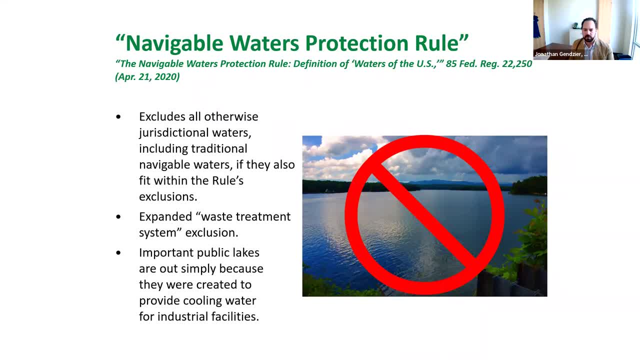 So one example here is the expansion of the waste treatment system exclusion so that traditionally navigable waters used as cooling ponds are excluded from Clean Water Act jurisdiction, even if they're used for drinking water or public recreation and in interstate commerce. Next slide, please. 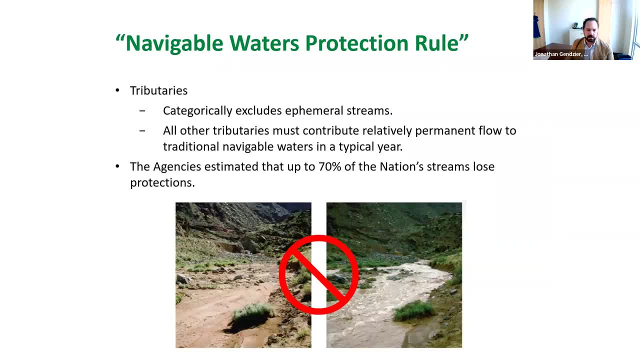 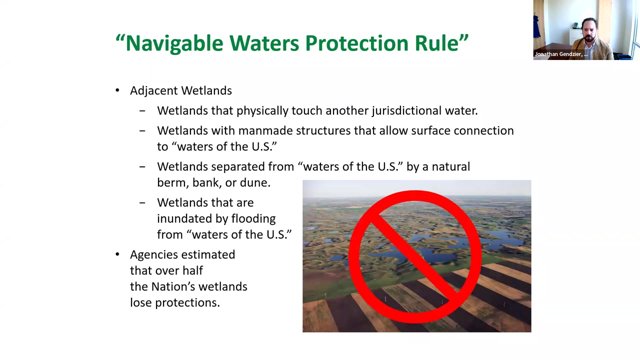 The rule categorically excluded ephemeral streams. It adopted the Rapanos pluralities emphasis on permanent flow, And the agencies acknowledged in the rulemaking that even some intermittent and perennial streams would be eliminated from jurisdiction. Next slide, please. The rule also severely restricted wetland protections and it emphasized the need for a wetland to touch or have a permanent surface water connection with. 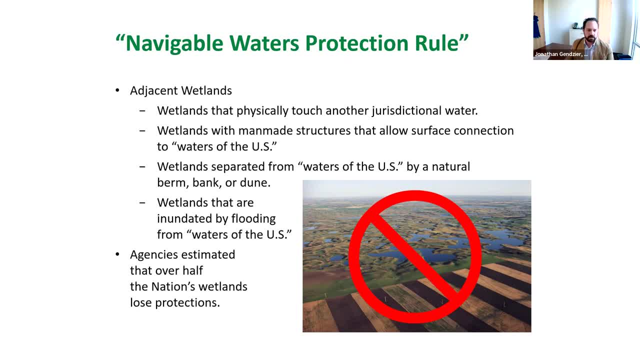 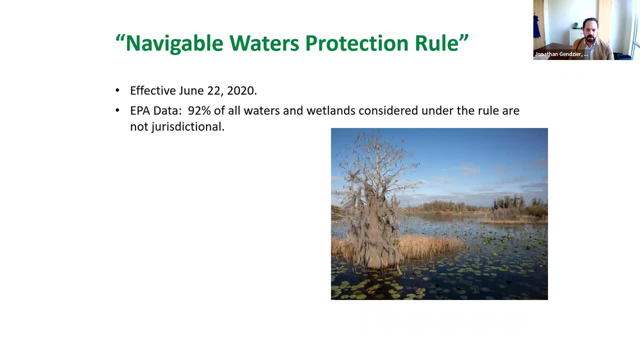 a jurisdictional water as defined by the rule. Next slide, please. So, according to data from EPA on the actual implementation of this rule, 92% of waters that were considered in issuing approved jurisdictional determinations were found not to be jurisdictional, not to be protected by the Clean Water Act. 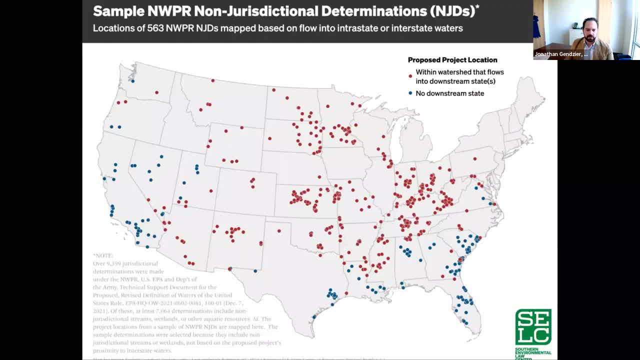 Next slide please. This is just a map of 563.. Next slide please. Next slide please. Next slide please. These are the non-jurisdictional determinations. We've talked some previously about downstream effects of pollution and interstate effects. 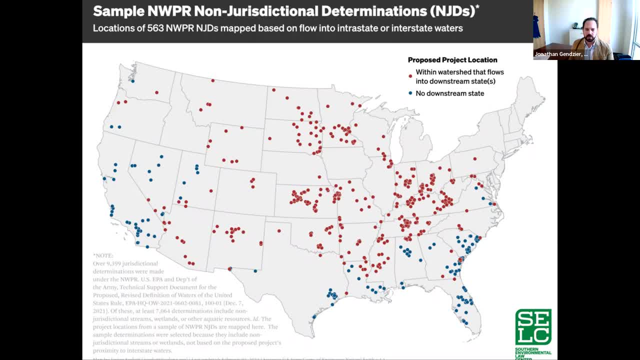 So the red dots show sites where the waters on site were determined not to be protected by the Clean Water Act in watersheds that flow into another state. I think that illustrates that issue, that the downstream state is left powerless to regulate the discharge flowing in from upstream. 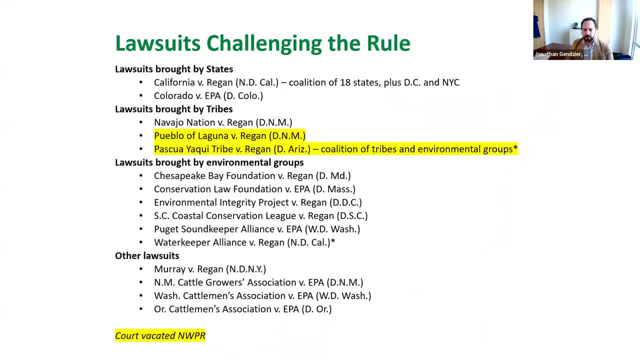 Next slide, please okay. so, as i mentioned, two district courts vacated the rule. there were a number of challenges to the navigable waters protection rule. some of these have been remanded without vacature, others have been stayed and we don't expect a merits decision in any of the still pending cases. next slide: 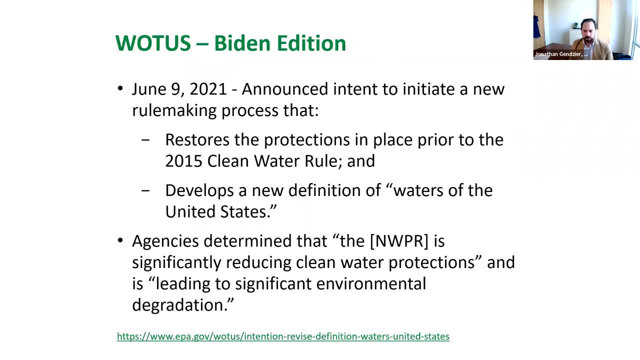 please. so last summer, almost exactly a year ago, the agencies announced their intent to initiate a new rulemaking process to restore the pre-2015 clean water rule protections. so not going back to the clean water rule, but going back to what it was in place before that next slide, please. 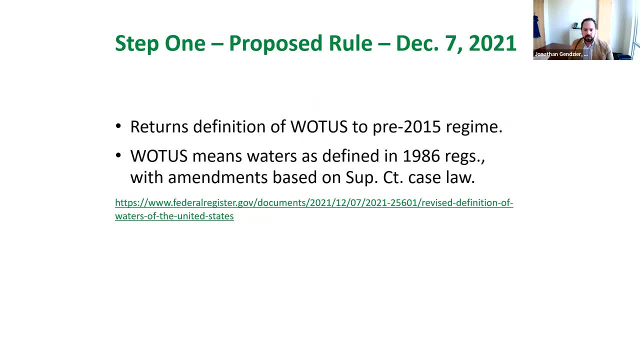 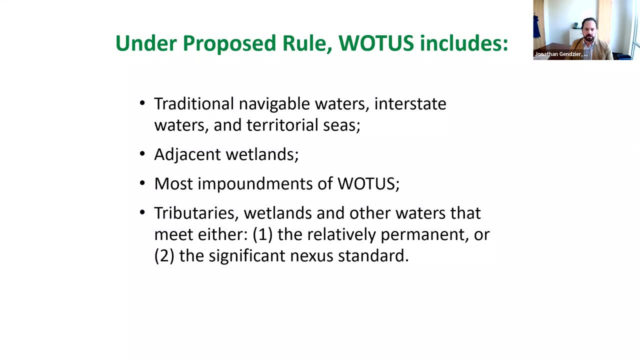 the. so the proposed rule came out in december of last year and the comment period closed in february of this year. next slide, please. so under the proposed rule, waters of the us includes the traditional, traditional navigable waters, interstate waters and territorial seas and adjacent wetlands to those most. 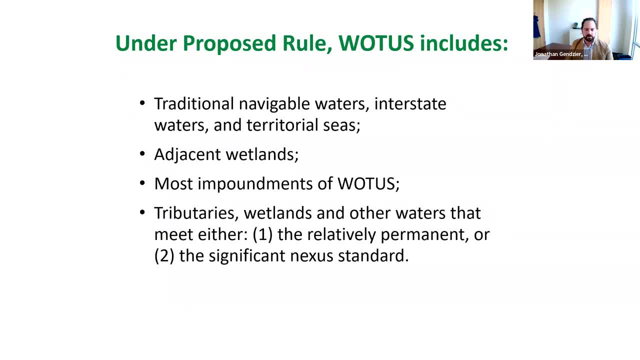 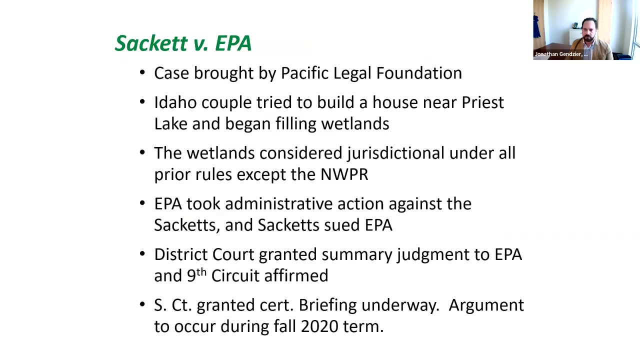 impoundments of waters of the us and tributaries, wetlands and other waters that meet either the permanent or the significant nexus standards from the rapanos rule. next slide, please. we'll go ahead to the next slide as well, so i'd be remiss not to mention a pending supreme. 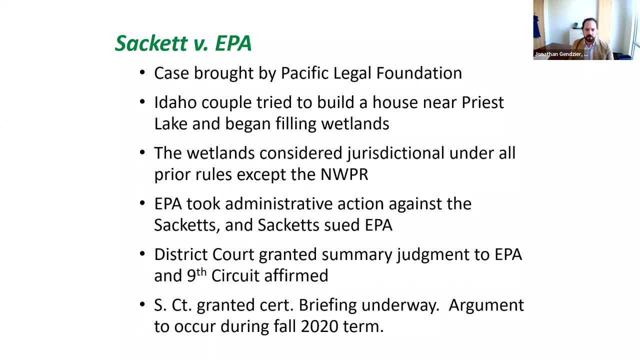 court case on this issue. saket v epa involves construction or attempted construction of a house in idaho where wetlands were filled that had been considered jurisdictional under all prior laws, except for the navigable waters protection rule, the. the district court granted summary judgment to epa when that finding of jurisdictionality was challenged, and that was. 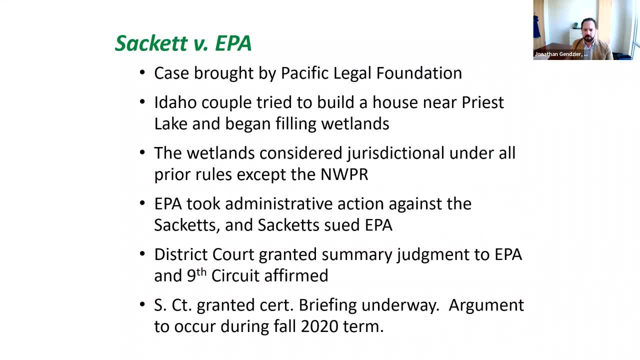 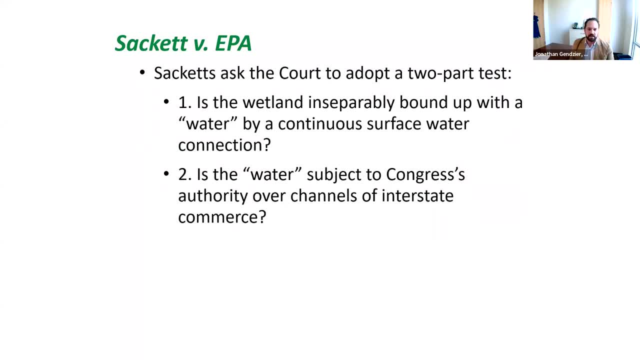 affirmed by the ninth circuit. the supreme court then granted cert and briefing is underway. now next slide, please. so the? the opponents in this case have asked the court to adopt a two-part test for jurisdiction: is the wetland inseparably bound up with a water by a continuous surface water connection? and two, is the the water that they refer to? 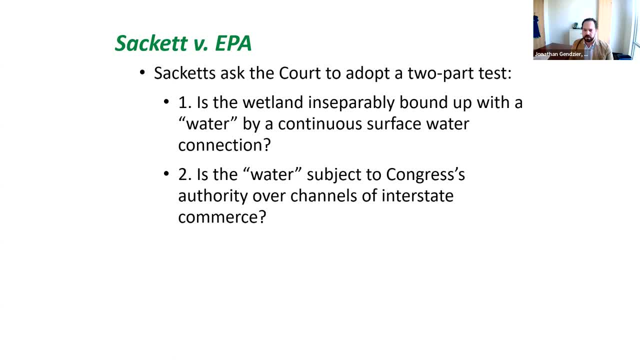 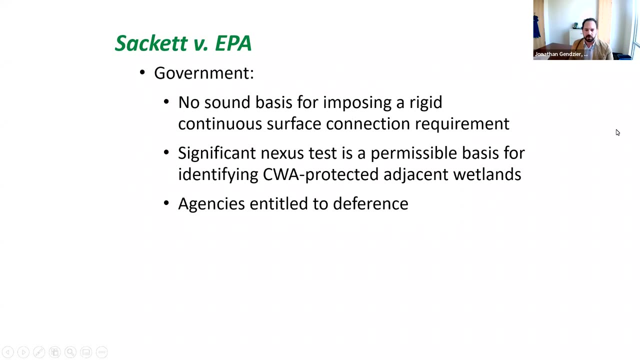 subject to congress's authority over channels of interstate commerce. this is arguably more restrictive than the scalia test set forth in rapanos. next slide, please. the? the government has argued that there's no sound basis for imposing a rigid continuous surface water connection requirement and that the significant nexus test is a permissible basis. 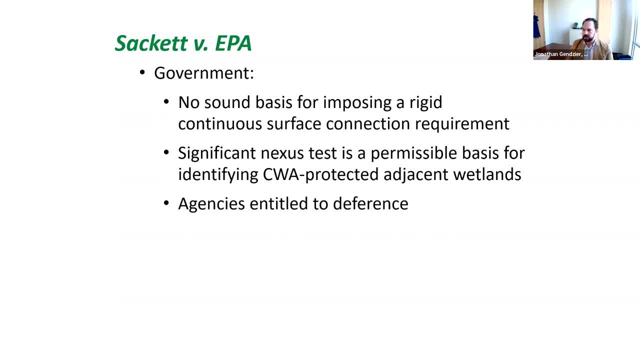 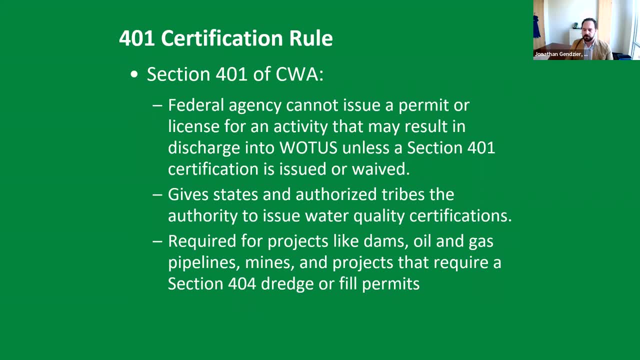 for identifying protected adjacent wetlands. next slide, please. so i'm aware i'm running short on time and i'd like to just give you an overview of a different clean water act topic: the 401 certification rules. so this is the mechanism under the clean water act for states. 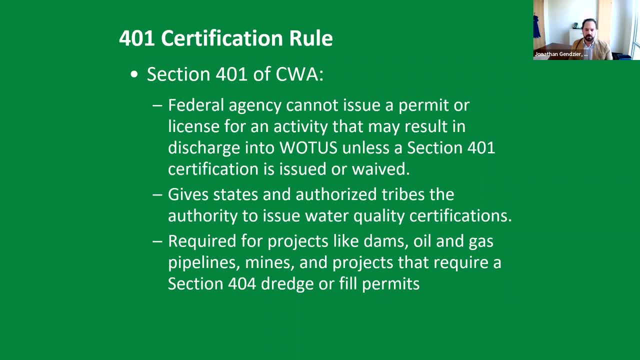 to review and condition projects with federal licenses or permits to ensure that they will comply with state water quality standards. Some of the projects where a Section 401 certification is required include dams permitted by FERC interstate oil and gas pipelines. Also, this is required for dredge and fill permits. 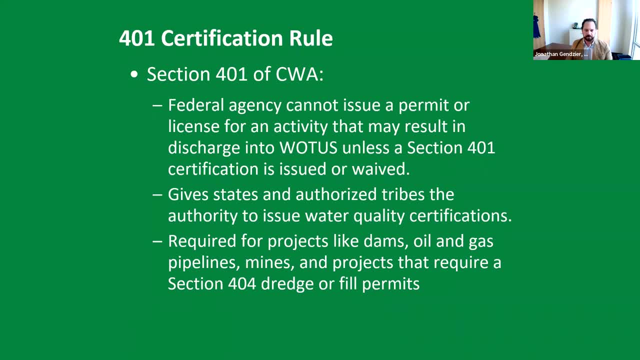 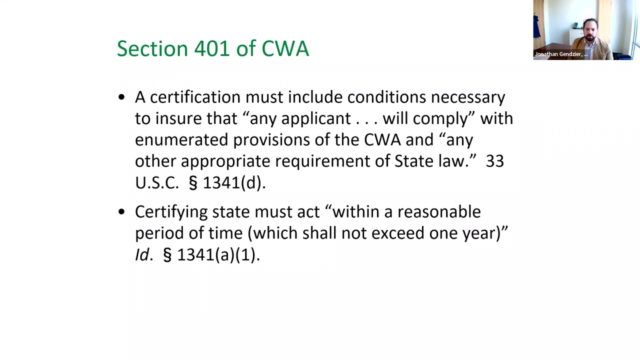 under Section 404 of the Clean Water Act. Next slide, please. So the certification has to include conditions that will ensure that the applicant will comply. Oh sorry, next slide, There we go. Will comply with enumerated provisions of the Clean Water Act itself. 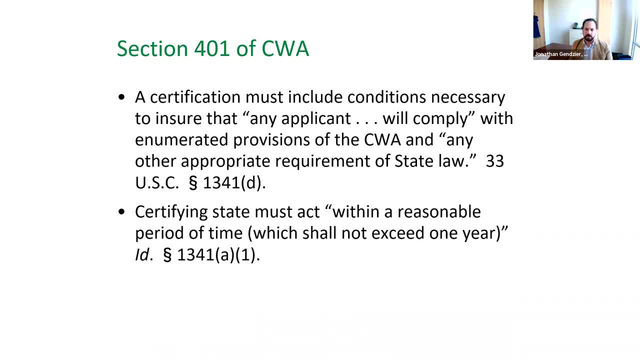 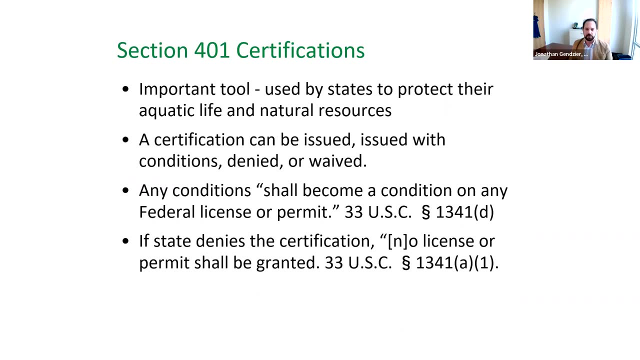 and then any other appropriate requirement of state law. It also sets out a reasonable period of time, not to exceed one year, for the certifying state to take action on a request for certification. Next slide, please. So why is this important? It's used by states to protect aquatic life. 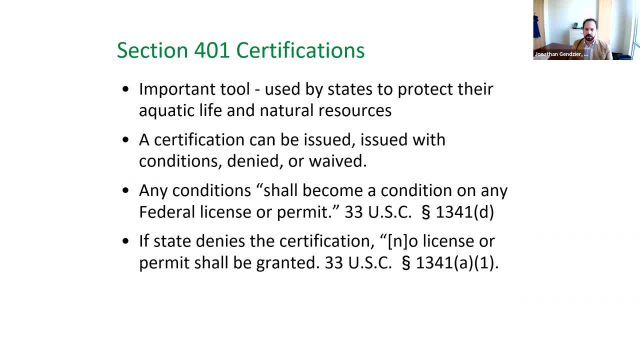 and natural resources to protect those designated uses of their waters. The certification can be either issued or issued with conditions, excuse me- or denied or waived And once issued, any conditions in the certification become a condition on that federal license or permit. 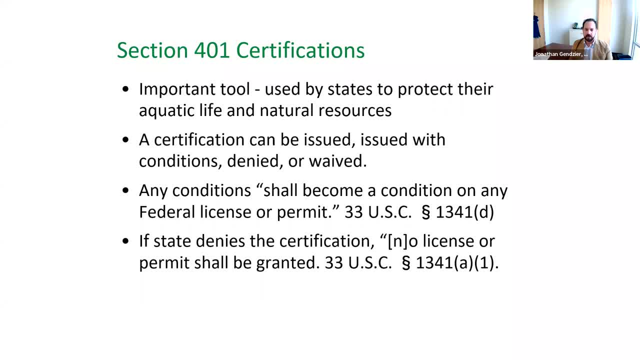 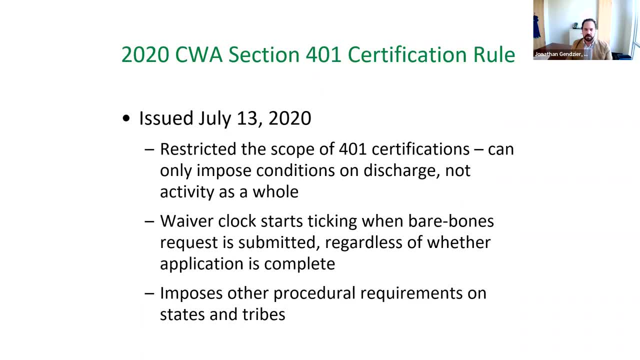 And importantly, if the state denies the certification, then no license or permit can be granted. Next slide, please. The Trump administration issued a rule on Section 401 certification in 2020 that severely restricted state and tribal authority to impose conditions the scope of their review of projects. 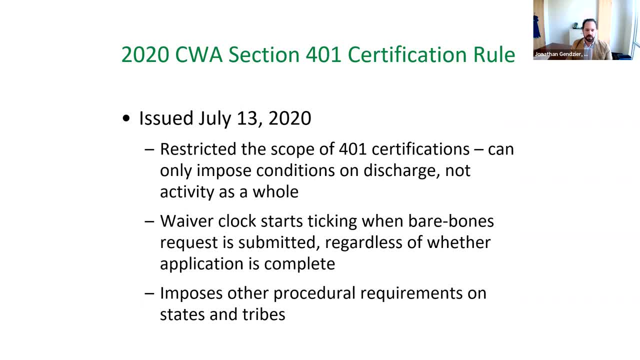 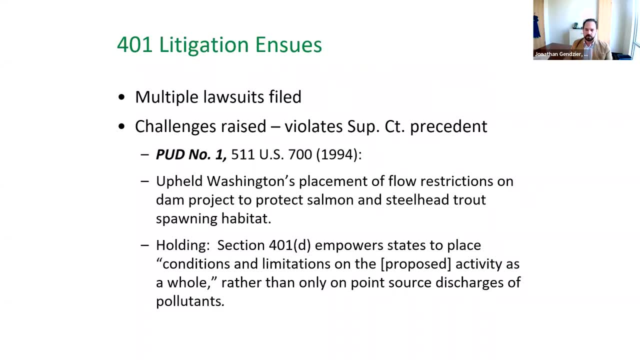 and the timing that they had to do that. review Next slide, please. There were a number of challenges to this 2020 rule. One important issue was there is Supreme Court precedent that allows states to review the activity as a whole, not merely the triggering point: source discharges. 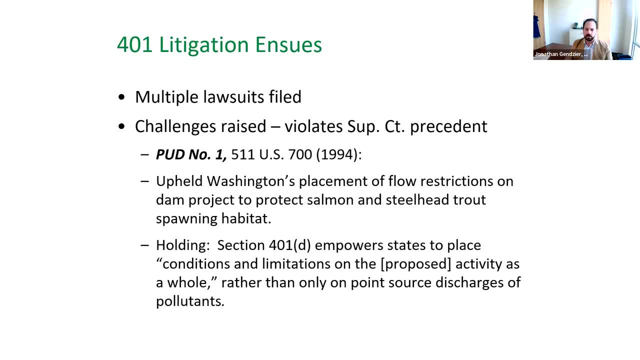 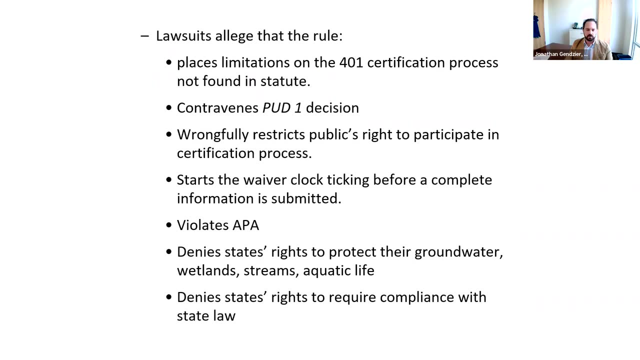 that trigger the certification requirement and state's ability to review other aspects of the project and their impact on state water quality was curtailed by the 2020 rule. Next slide, please. So here's just a list of some of the allegations. 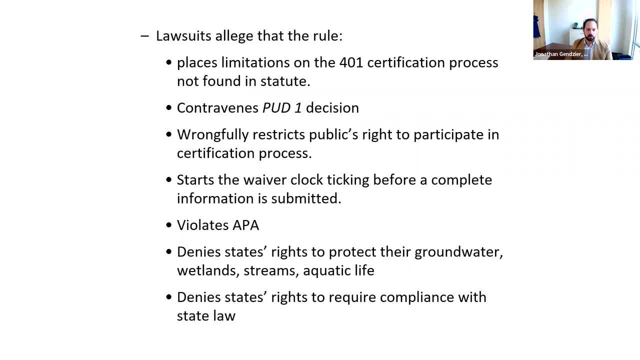 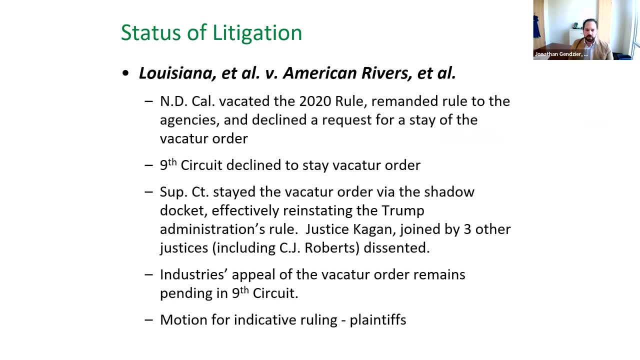 in the various lawsuits challenging the 2020 rule. Next slide, please. So current status here in the Louisiana v American Rivers case, which is pending in the 9th circuit, the Northern District of California vacated the 2020 rule. 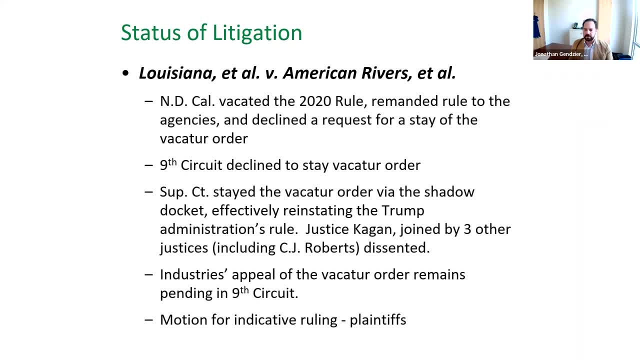 and remanded it to the agencies. The 9th circuit Circuit declined to stay that vacature. while the appeal is pending, However, the Supreme Court did issue a stay of the vacature order and it has effectively reinstated the 2020-401 certification. 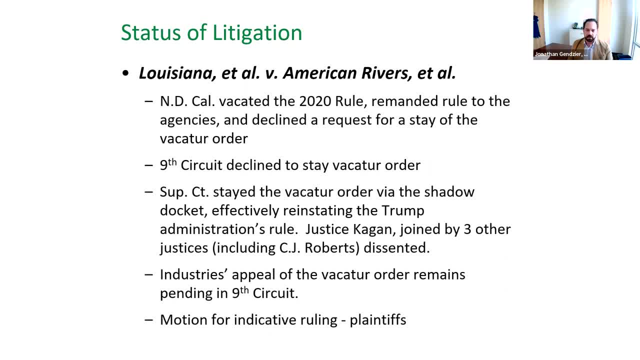 rule while the appeal is pending in the Ninth Circuit. Interestingly, the plaintiffs- if you will- blue states, tribes and environmental groups challenging the 2020 rule- have now moved for an indicative ruling in the district court, And so they're allowing asking the judge there. 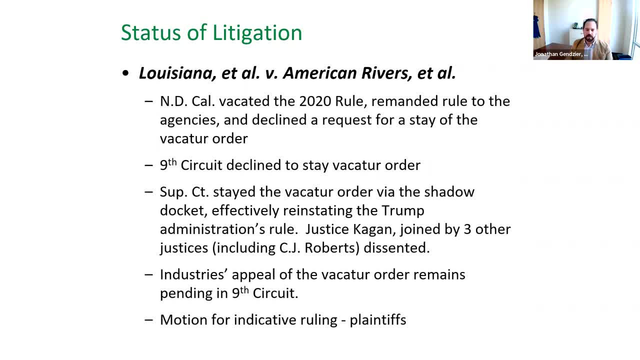 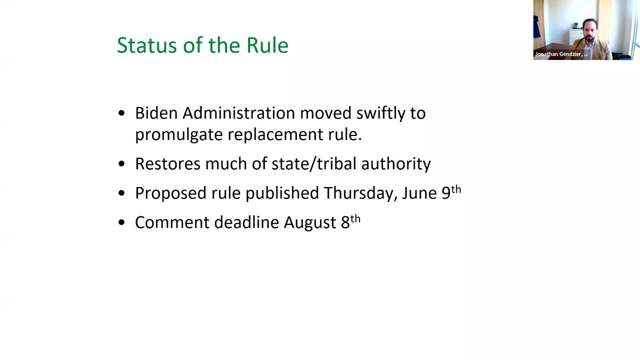 to allow the case to move forward to the merits, And that looks like it has now been fully briefed as of June 7th and is awaiting a decision by the judge. Next slide, please. So the Biden administration has moved swiftly to promulgate a replacement rule here that came out on June. 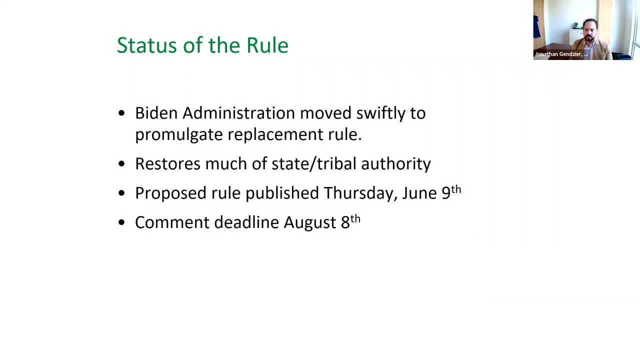 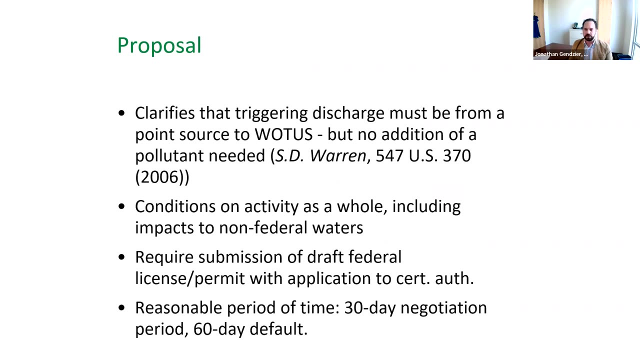 9th and it appears to restore much of the state and tribal authority under the Clean Water Act to review these federally licensed projects. Next slide. please Just a couple of highlights from the rule As proposed. it clarifies that the triggering discharge is from a point. source. 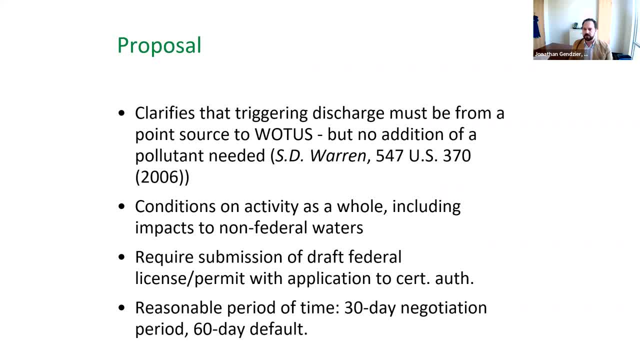 to a water of the United States, but that no addition of a pollutant is needed, And that's consistent with Supreme Court precedent and is important in the context of things like dams that may be discharging water that has an impact on state water quality. 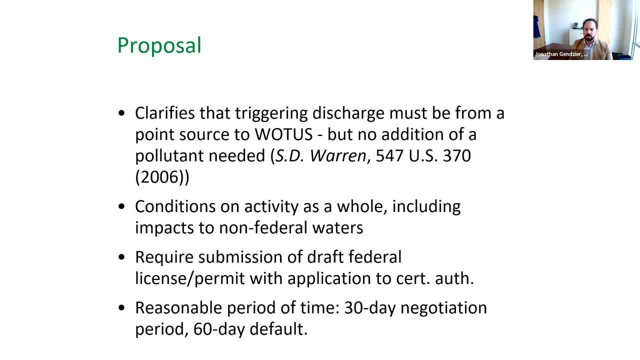 but it's not in fact adding a pollutant to that water. It also allows states and tribes to place conditions on the activity as a whole. that's being reviewed And that includes impacts to non-federal waters, once that point source discharge to a water of the United States is. 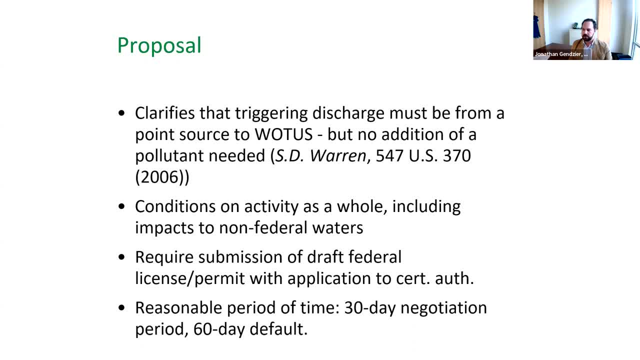 triggered Also requires submission of a draft of the federal license or permit itself To the certifying authority. That's something that was not previously required and would appear to allow states and tribes to have access to more information about potential impacts to state waters. Thank you very much and I look forward to discussing your questions later. 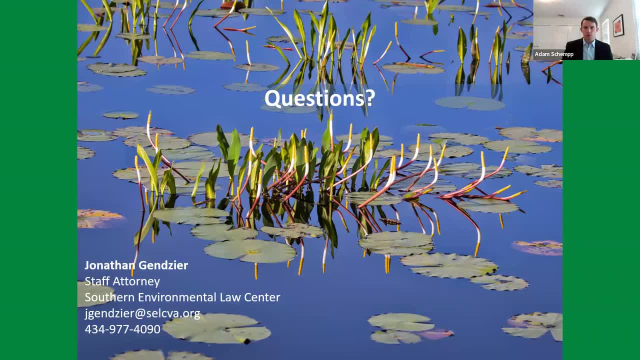 Thank you very much, Jonathan. Just two quick clarifications here before we move on to Aaron. One is: is similarly situated, defined by Kennedy. The phrase similarly situated, Do you recall? I don't recall. I believe that he may provide some detail about what that might look like. 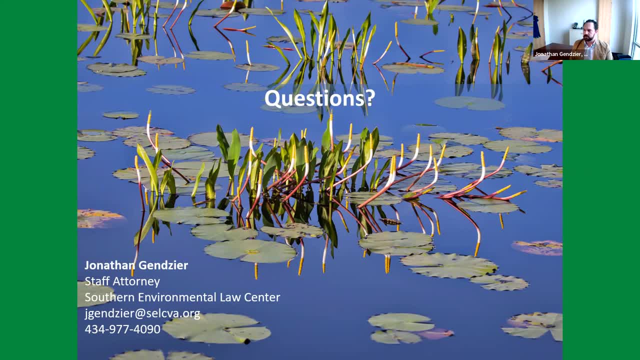 but it's going to be left to the agencies to formally define that. Okay, thank you. And the other was just a clarification that the Sackett case is indeed ongoing. Is that right? That's correct, And oral argument was just scheduled, I believe, for October 3rd, if I remember correctly. 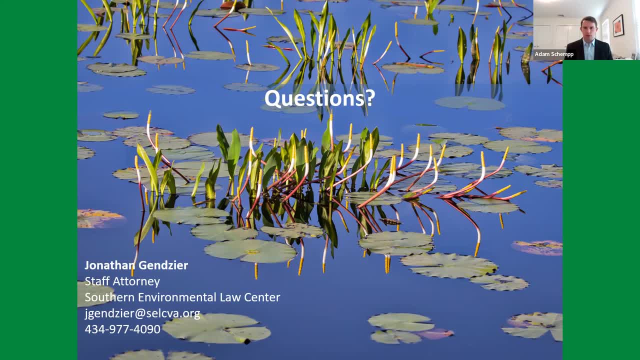 And one more just came in: Does the proposed Clean Water Act regulation include discussion on PLA wetlands? That may have been an error. I don't know what PLA wetlands are. Okay, I'm not certain either. Okay, All right, We'll come back to that, Leslie. 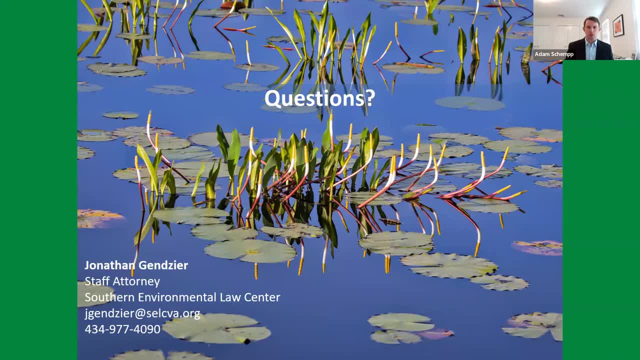 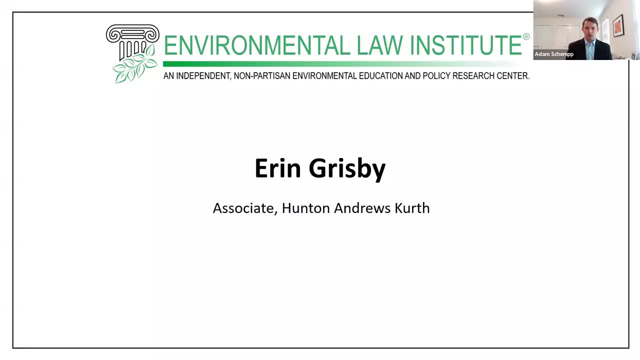 if you're able to clarify that, that would be great. We'll address it in the main Q&A. All right With that? I would like to first of all thank you, Jonathan, And now hand things over to Aaron Grisby. So Aaron is an associate at Hunt & Andrew Curse and part of their environmental 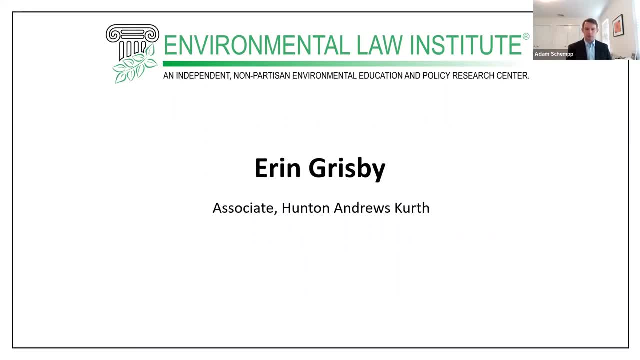 practice group, She advises clients on regulatory and compliance issues, with a specific focus on clean water in the Clean Water Act. Prior to joining the firm, Aaron was an Attorney at EPA Headquarters in the Water Enforcement Division and the Air Enforcement Division of the Office of enForcement and Compliance. With this, he's a communityम. Sofia andise is a technologist with. 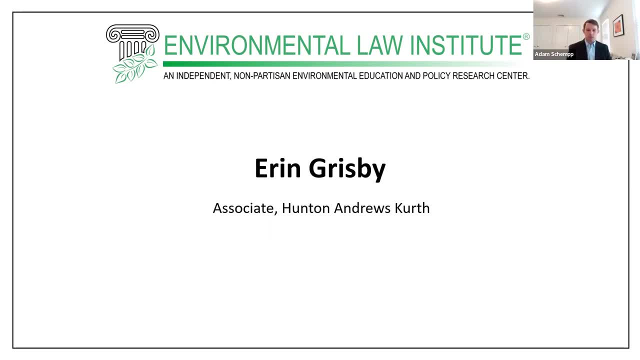 iar enforcement division and the Air Enforcement Division of the Office of Enforcement Compliance. She also has worked in several US Department of Justice branches and at the White House Council of Environmental Quality. Erin received her law degree from the University of San Diego School of Law and her bachelor's degree from UC Santa Barbara. 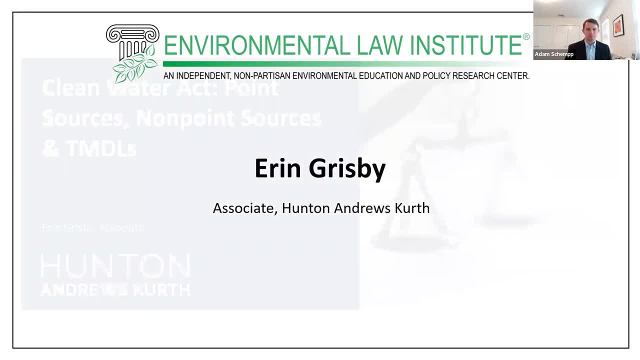 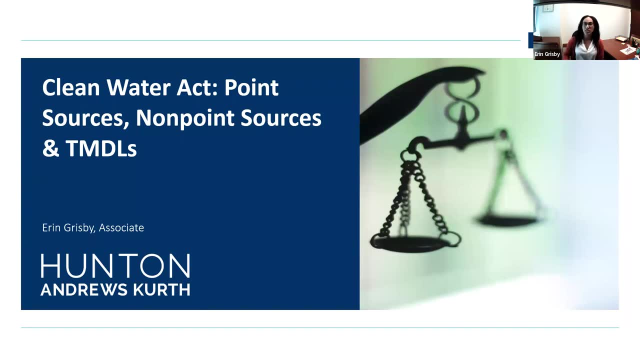 And with that, Erin, the floor is yours, Thank you. So today I'll be discussing point sources, non-point sources and total maximum daily loads, And so I know we're a little. I'll kind of go through this all quickly- I know we're a little bit behind on time- and answer your questions. to leave some time to answer your questions. 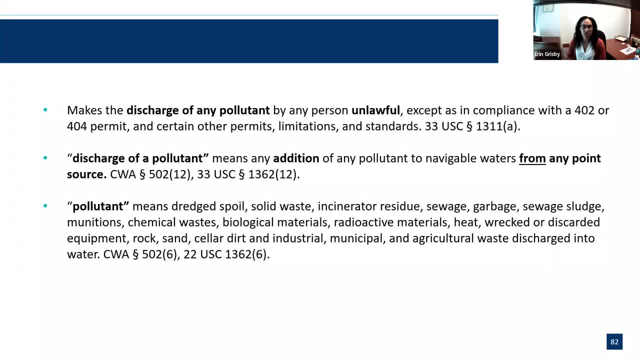 So next slide. As mentioned already, Section 301 of the Clean Water Act makes the discharge of any pollutant by any person unlawful except as in compliance with a section 301 of the Clean Water Act, Section 402 or 404 permit or other certain other permits, limitations and standards. 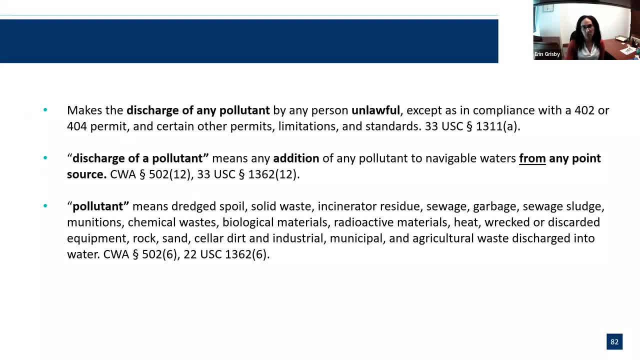 So the discharge of any pollutant is defined by the Clean Water Act to mean any addition of any pollutant to navigable waters from any point source. Pollutant you'll see here is defined quite broadly, covering everything from sewage, dried soil, rock, chemical waste, industrial, municipal and agricultural waste. 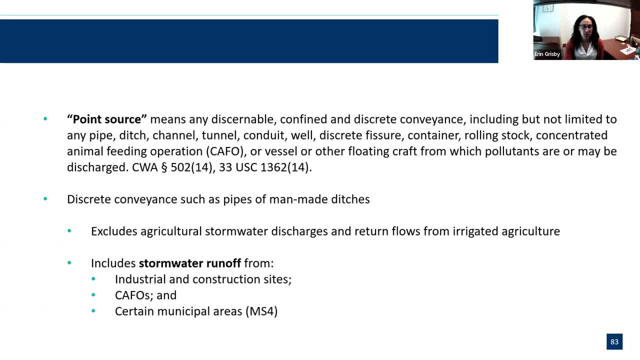 Next slide And the Clean Water Act goes on to define point source also quite broadly. You'll see, you can read there all the different categories, which also include CAFOs, which I'll mention later. So effectively any discrete conveyance such as a pipe or manmade ditch is is a point source under the Clean Water Act. 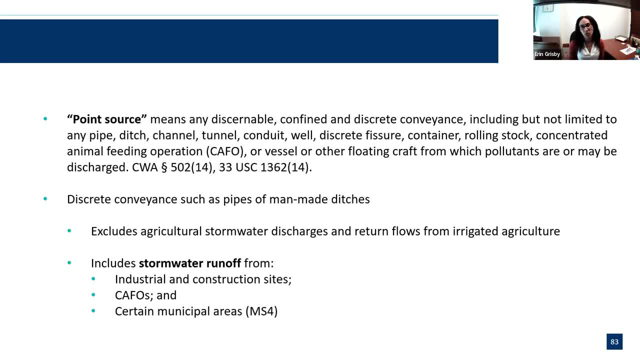 The definition excludes agricultural waste. It excludes agricultural stormwater discharges and return flows from irrigated agriculture. However, the Clean Water Act does include stormwater runoff as a point source from industrial and construction sites over a certain size, From CAFOs. CAFOs are animal feeding operations that meet certain conditions. 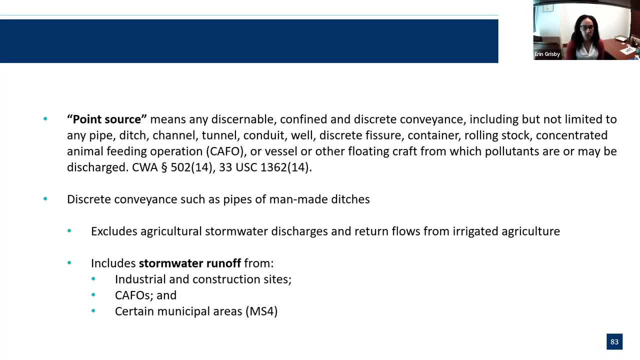 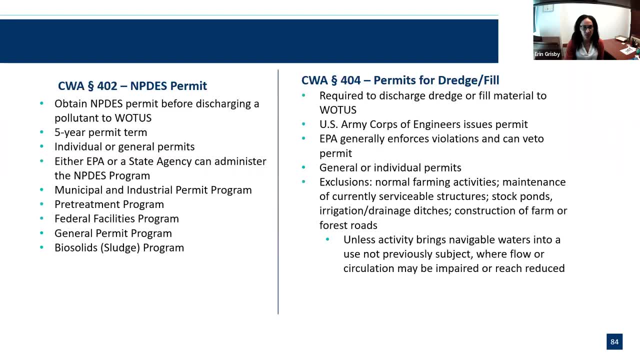 and it also includes stormwater runoff from certain municipal areas under what are known as MS4.. Next slide. So, as I mentioned, under the Clean Water Act, discharge of pollutants are allowed so long as they are permitted. So the NPDES, the National Pollution Discharge Elimination System, controls discharges of pollutants to our waters. 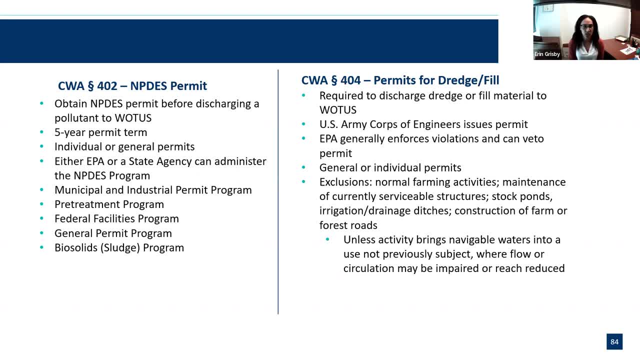 I'm not going to focus too much on permitting, but I just wanted to go over a little bit here on some of the two basic permits. The NPDES permit is one of the primary ways the US controls water pollution, as Robin already mentioned. 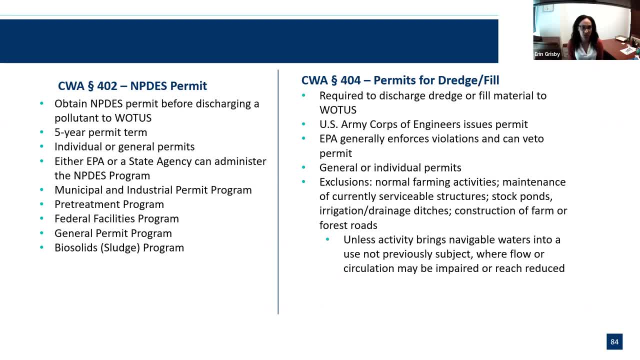 So you must obtain the NPDES permit before discharging a pollutant to waters of the US, which is what the water of the US is. It's controversial, as Jonathan just went through, So these permits are five-year-long permits. 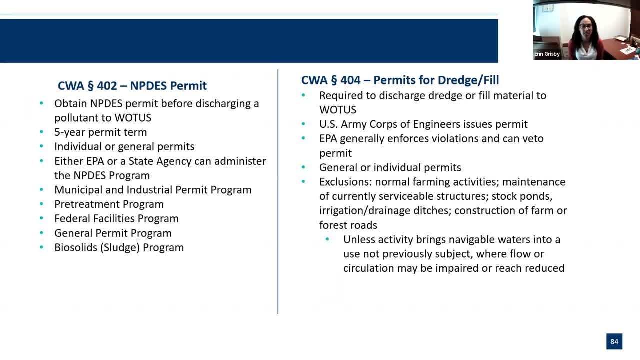 That's the term They need to be renewed. after that You may see some permits renewals happening after the five-year mark, but the permit itself continues on until sometimes, while they're sorting out a renewal. The permit can be an individual permit or a general permit. 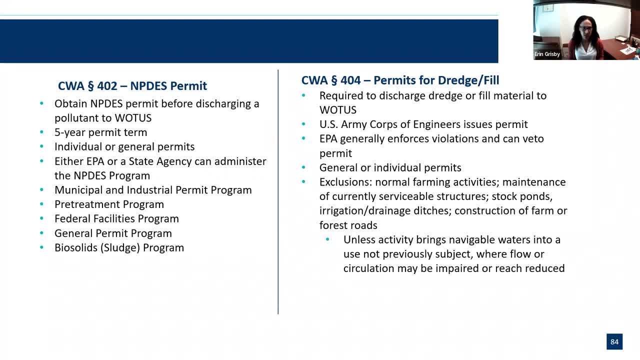 And what that means is. the individual permit would be site-specific and with conditions that address a particular facility or location. The permit can be issued to an individual permittee or co-permittee that are co-located at a site. For a general permit, this would be a permit that's issued by the permitting authority generally. 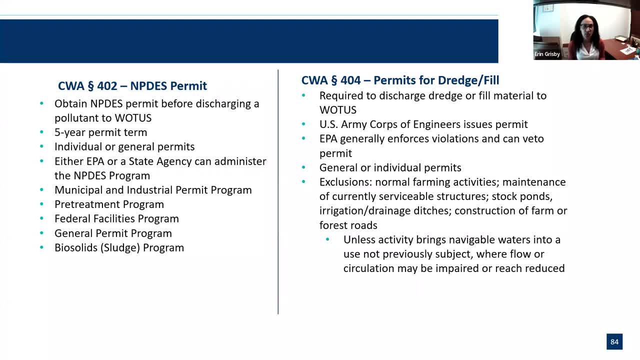 And then those that fit the contours of the permit can apply for coverage under the permit. So multiple entities would apply for coverage under one general permit. Either EPA or state agency can administer the NPDES program, And I think today there's less than a handful of states that haven't taken over administration of their own programs. 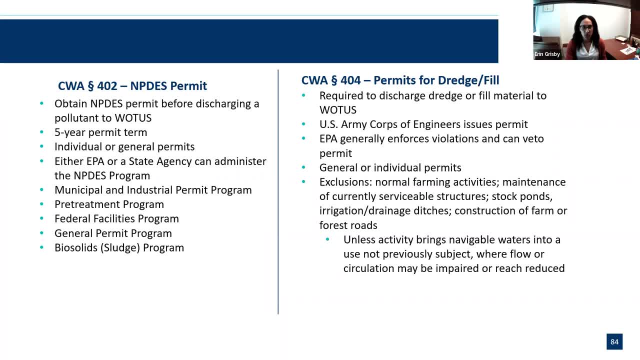 This just outlines a few of the different programs. The Municipal and Industrial Permit Program. Robin mentioned some aspects of the Municipal's program dealing with the sewerage And combined sewer systems for sanitary sewer systems. The Pretreatment Program ties in with those publicly owned treatment works handled by the municipalities. 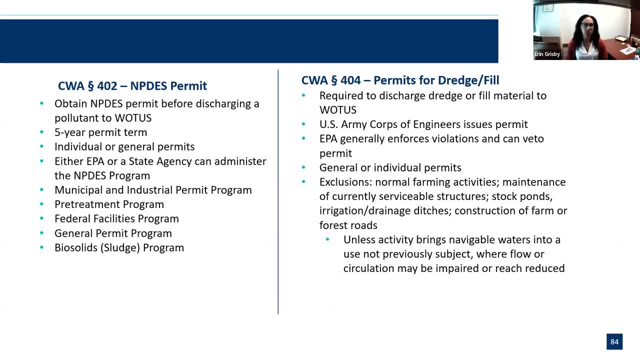 The Pretreatment Program serves to protect the treatment facility, So the facility might not be designed to handle certain types of waste streams or pollutants. So an industrial user would need to treat their wastewater prior to discharging to the local wastewater system under the Pretreatment Program. 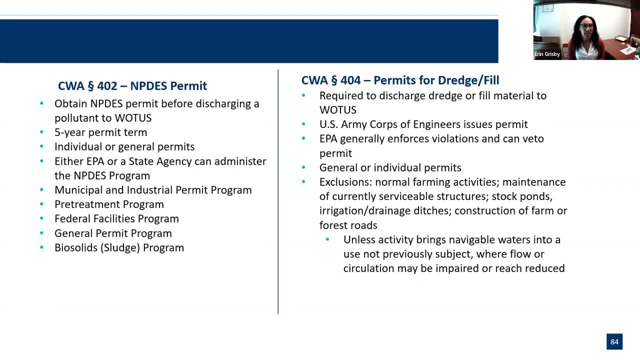 Federal facilities also have to comply, And you'll see here. there's also aspects that deal with the Biosolids Sludge Program, Under which certain solids are separated during the municipal treatment process And those are used for land application, Such as for non-polluted land. 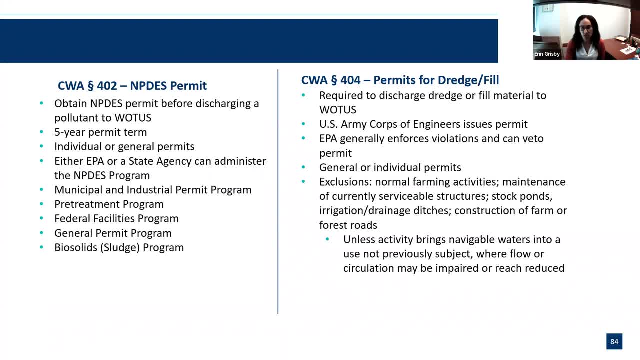 Such as for non-food crops, For landscaping, Or they're taken for surface disposal. So there's part of the program to make sure that those are handled correctly, And then there's interplay with the Corps. Jonathan mentioned some of this. So under Clean for the Section 404, permits are for dredging and fill permits. 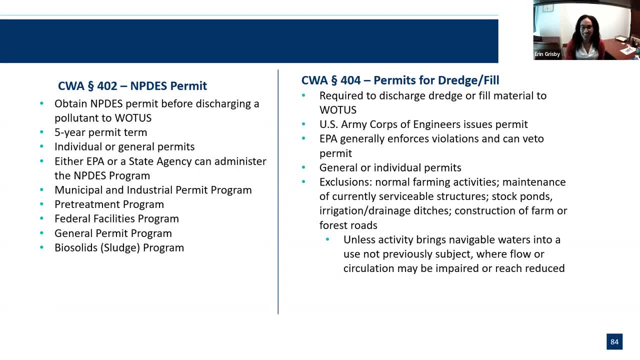 And, as Robin mentioned, these are kind of dating back to the very beginning of our environmental laws, Whereas the dredge and fill program And these require the permits if you're going to discharge retrofuel material to waters of the US. The Corps issues these permits. 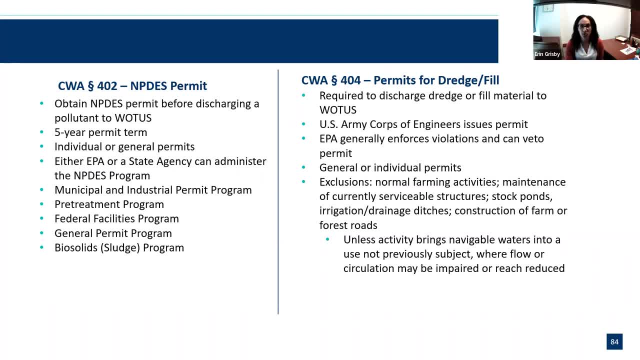 EPA generally enforces. EPA does have veto authority. It can veto these permits. These can be general or individual as well. There are some exclusions laid out in the law And here they are listed here. But then those exclusions don't apply if the activity 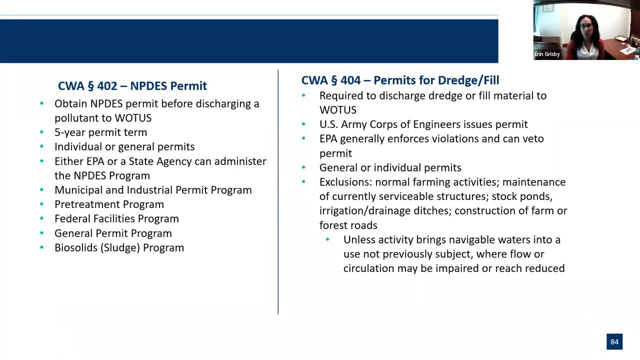 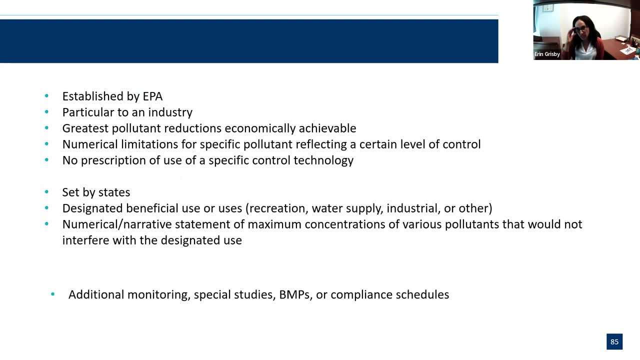 Nevertheless brings navigable waters into a use that it was not previously subject to. That changes the flow, The circulation, Or reduces the reach of the waters. Next, slide As far as the content of an NPDES permit. What you're going to find in each permit will be what we commonly refer to as T-bells or Q-bells. 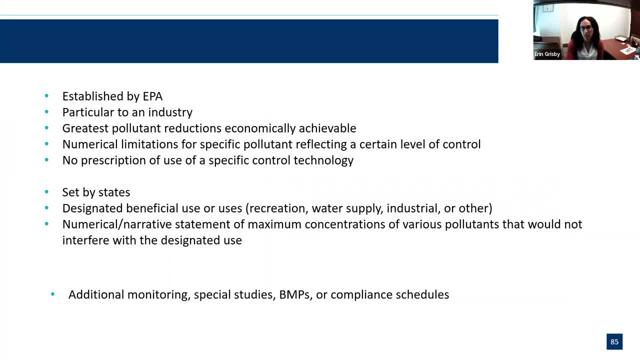 So you're going to have your technology-based effluent limitations. These are established by the EPA. They're particular to an industry. They seek the greatest pollutant reductions economically available or achievable, And so they are numeric limitations for a specific pollutant that reflect a certain level of control. 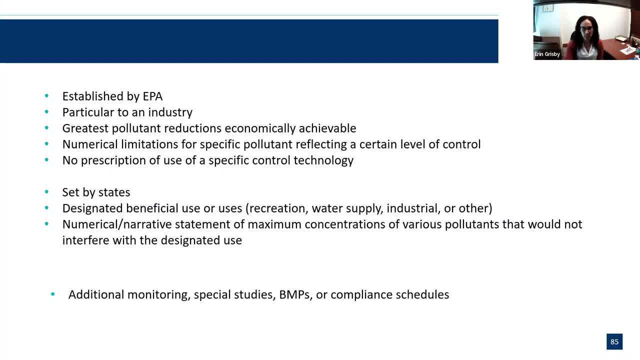 So, while they're called technology-based effluent limitations, they don't prescribe the use of a specific control technology. You'll also see water quality-based effluent limits in these permits. These are set by the states. They're based on designated beneficial use or uses for the particular water body. 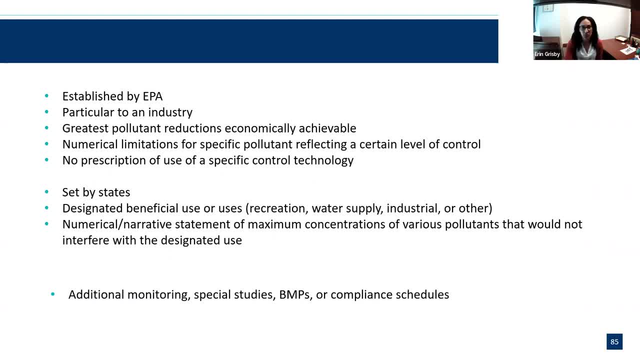 And here I've listed a couple of those uses: Recreation, water supply, industrial or other. The water quality-based limitations can be numerical or they may be narrative, And they provide the maximum concentrations of various pollutants that would not interfere with whatever the designated uses are. 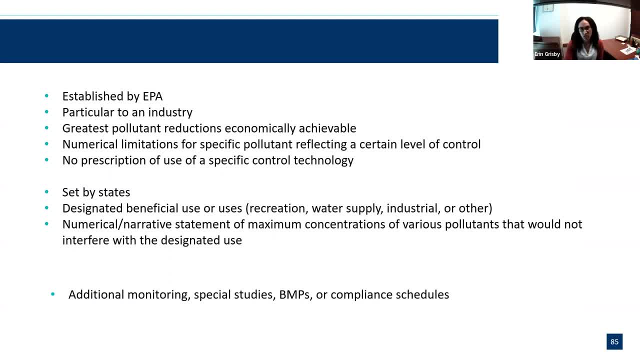 And so they're based on designated For the particular water body. You'll also find monitoring and reporting requirements. There may also be special conditions for additional monitoring, special studies, best management practices or compliance schedules, especially if there had been some prior violations that need to be incorporated into the next iteration of a permit. 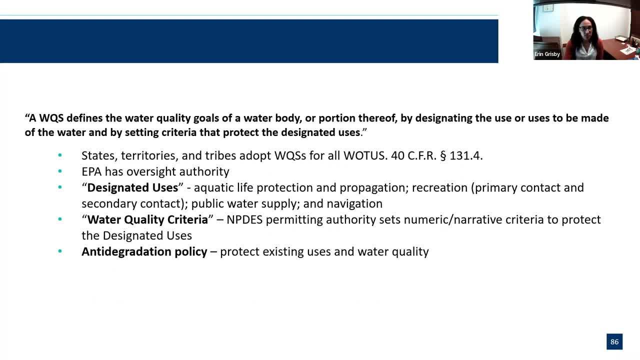 Next slide. So the water quality-based Effluent limits in the permits are based on water quality standards, And so it's explained in Title 40 of the regulations. Water quality standard defines the water quality goals of a water body or a portion thereof, by designating the use or uses to be made of the water and by setting criteria that protects the designated uses. 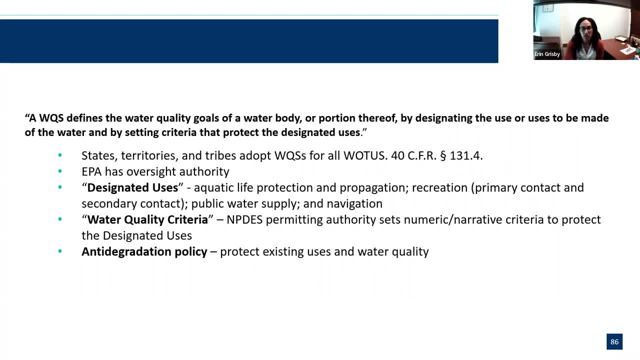 So the regulations also say that, wherever attainable, they should provide the water quality standards for water quality, The water quality standards should provide water quality for the protection of the propagation of fish, shellfish, wildlife and recreation in and on the water. 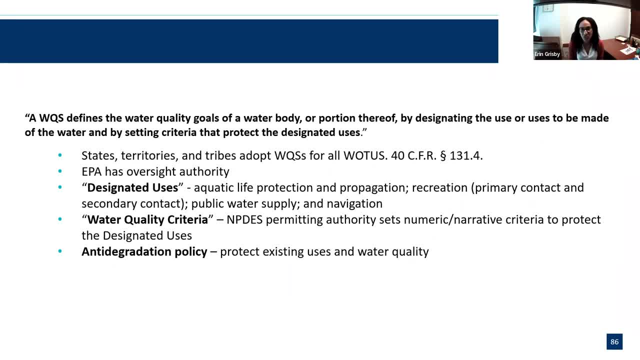 States, territories and tribes adopt water quality standards for all waters of the Us, And epa has oversight authority. So there's pretty much 3 elements to water quality standards. There's designated use, and there you have it listed there. And then there's the water quality criteria which I mentioned. you find inside the permits. 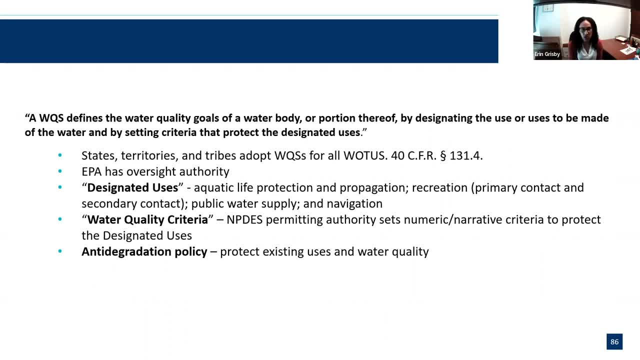 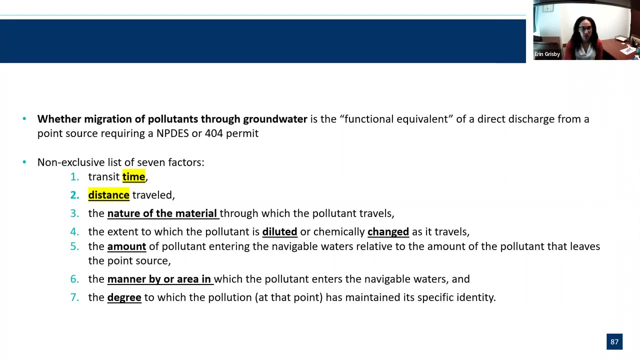 And there's also the anti-degradation policy which Robin touched upon. That's protects existing uses and the water quality so that it does not degrade. Next slide, please. So I actually I spoke about those, I pointed out those water quality standards because they're part of the content that's in the the Mpds permits. 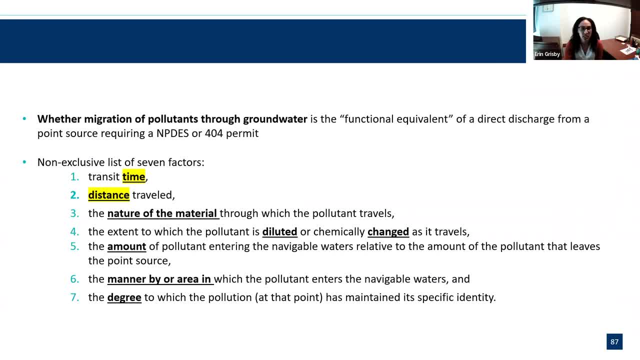 But i'll come back to those because they're relevant to something we're gonna talk about later on, But relevant to point sources. So one of the more recent developments in point source regulation was the county of Maui versus the Hawaii. Well, it's been a wildlife fund case, Supreme Court case in 2,020, which i'm sure most of you have already heard about by now and and gone through. 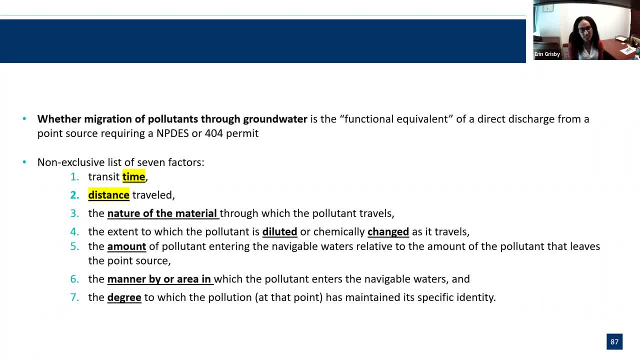 And so that's up for the functional equivalency test that helps determine whether migration of pollutants through groundwater is the functional equivalent of a direct discharge from a point source requiring a permit, And that. so they adopted that test, And so this is gonna help discriminate between what is point source and what is not a point source for purposes of Clean Water Act permitting. 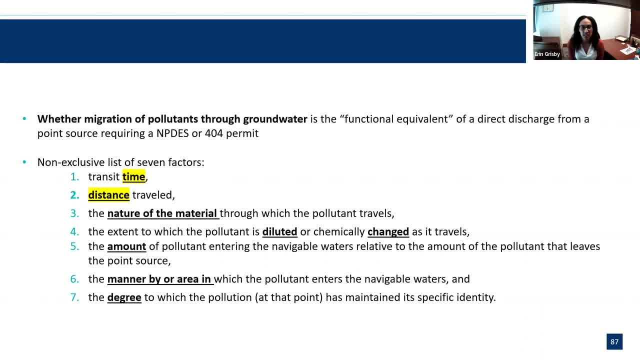 They. so it's a very fact, specific analysis. But the Supreme Court provided 7- non. It's a list of 7 non-exclusive factors. So here they are, listed here. They look at the transit time for the pollutants to get to the water of the Us. 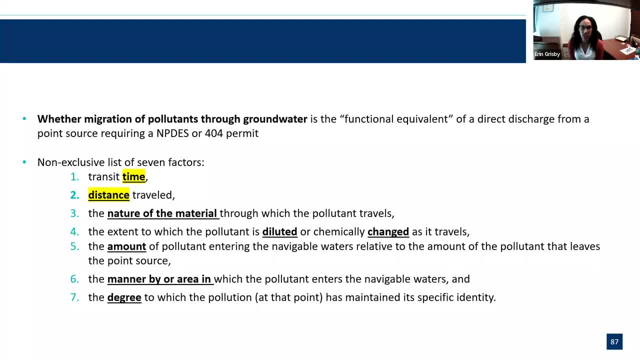 From the point source If it passed through the groundwater. the distance that it had to travel. the nature of the material through which the pollutant traveled. the extent to which the pollutant is diluted or chemically changed as it travels. the amount of the pollutant entering the Navigable waters relative to the amount of food. 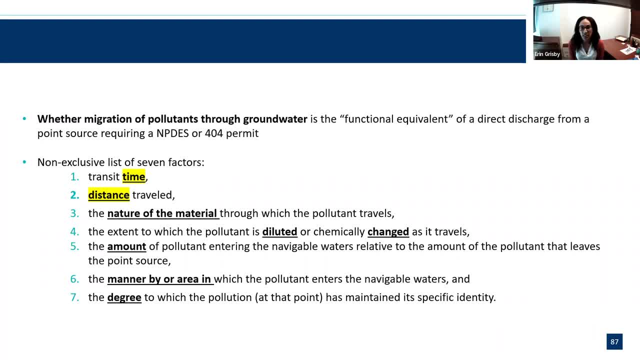 If it leaves the point source and the manner by or area in which the plan enters the Navigable waters and the degree to which the pollution at that point has maintained its specific identity. So the court did note that time and distance would be the most important factors in most cases, but not necessarily in every case. 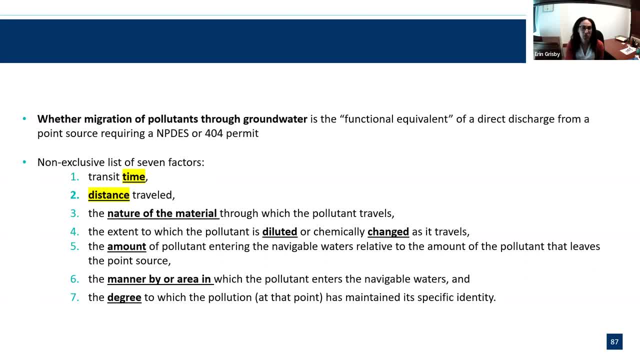 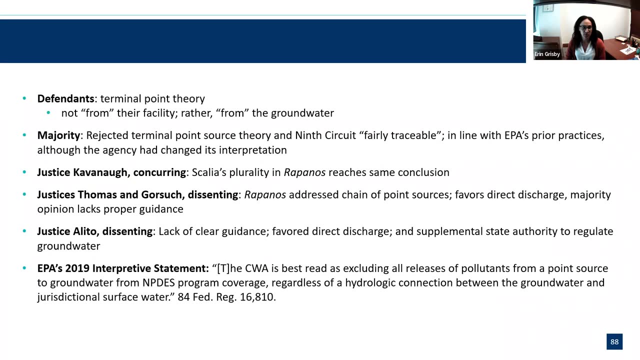 So it this decision continues to have major repercussions on clean water app liability cases. It certainly did for cases that were pending at that time. Next slide We'll go through a little bit of the arguments, probably as a refresher to some. So the defendants, among other things, argued pretty much the terminal point, source theory, that that the gluten didn't come from their facility. 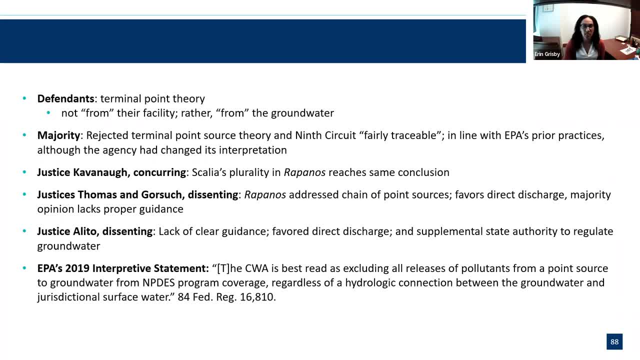 Rather it came from the groundwater And so, since it didn't come From their facility to the waters, That it was not within the Clean Water Act coverage. So the majority opinion rejected that terminal point source theory. They also rejected the Ninth Circuit standing fairly traceable test. 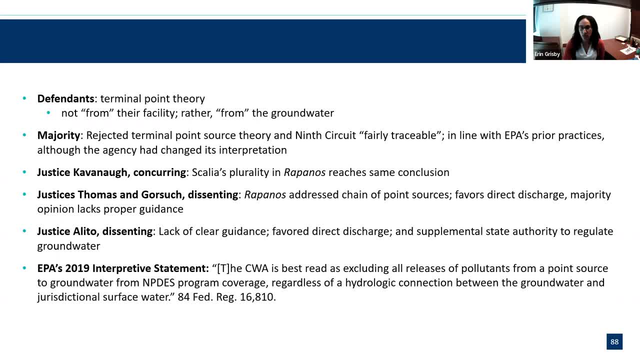 They found the fairly traceable test is overly broad, though, And they found that the The defendants argument that rejected for kind of the terminal point source theory providing total exclusion from clean water coverage was also objectionable. So the majority noted that their new functional equivalent test was in line with EPA's prior practices. 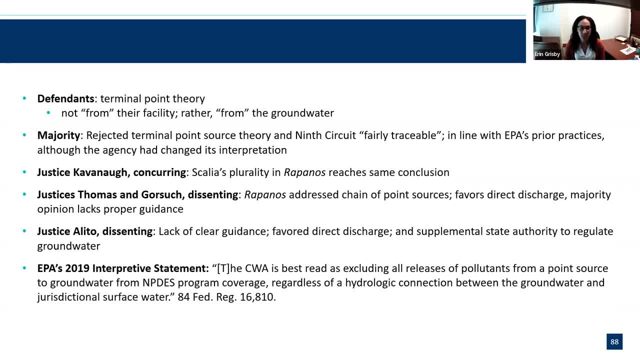 And even though, at the time of the opinion, EPA had Changed its interpretation And you can see that EPA's 2019 interpretive statement right there down at the bottom, The EPA- although Let's see In practice, I believe they had allowed for. 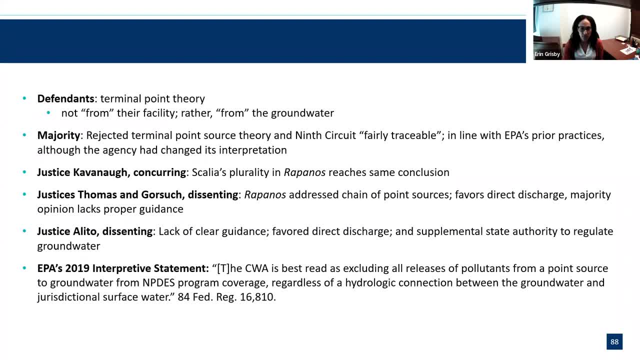 Let's see They had allowed for. Let's see here in my notes: They actually had prior version to discharges that reached groundwater only after lengthy periods of time, But they also did permit for situations where the discharge had gone through groundwater. But then their 2019 statement was different. 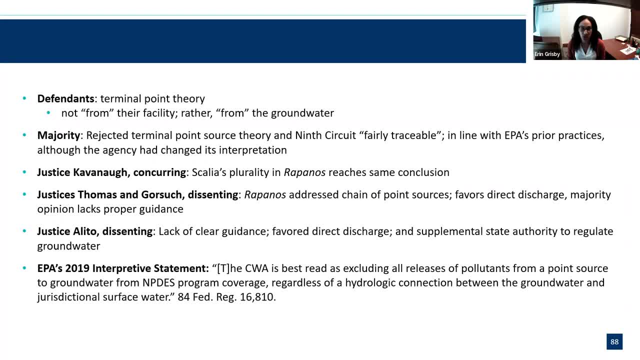 It said that the Clean Water Act is best read as excluding all releases of pollutants from a point source to groundwater, So regardless of any hydrologic connection between the groundwater and the jurisdictional surface waters. Justice Kavanaugh concurred. But he concurred And made it clear that 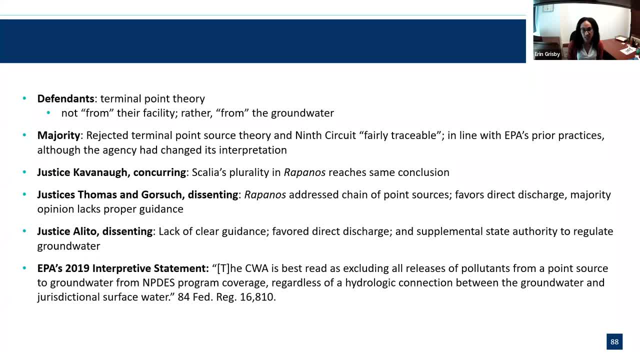 Scalia's plurality opinion and Rapanis would have reached the same conclusion That you didn't have to create this new test effectively. but he did agree. in the results, Justices Thomas and Borsas dissented. They looked at Rapanis and they said Rapanis was different. 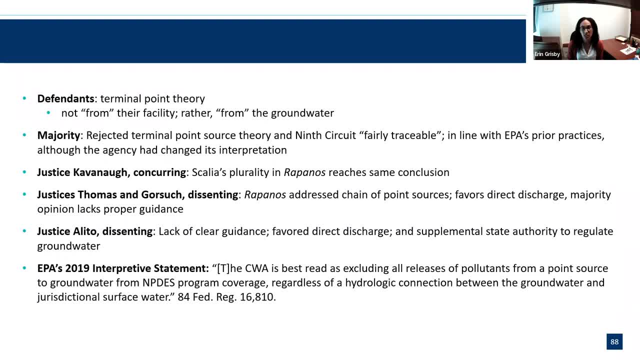 And actually perhaps would not have reached the same result because, Rapanis, They addressed It was a chain of point sources Which, in this case, The groundwater, In their opinion would not have been part of a chain of point sources. So 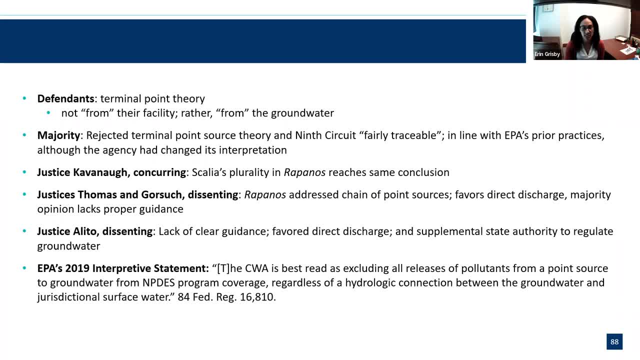 Justice Kavanaugh's dissenters favored the direct discharge theories And they felt that the majority opinion that set up for the seven Factors to consider lacked proper guidance and would potentially lead to inconsistent application. Justice Alito also dissented. He also felt there was lack of clear guidance. 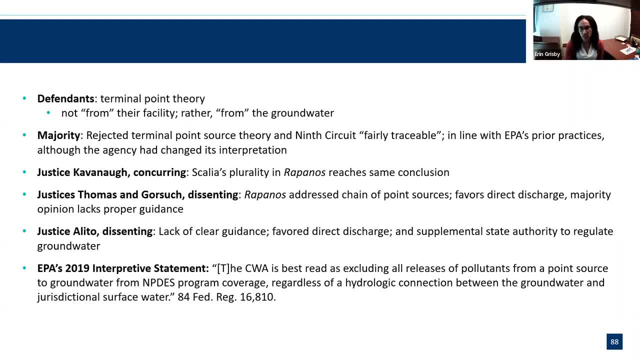 He gave her more of a disc direct discharge. But his theory of direct discharge was slightly different Than those other dissenters, And so Justice Kavanaugh's dissenters Decided Specifically that Supplemental state authority would be able to regulate groundwater. 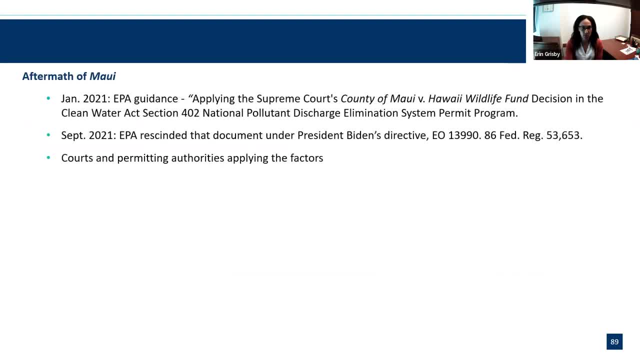 So that there was no need for EBA to necessarily reach so far Next slide. So, looking at the aftermath- Maui- In January of 2021, EPA issued a guidance applying the Supreme court's on applying the Supreme court's decision. 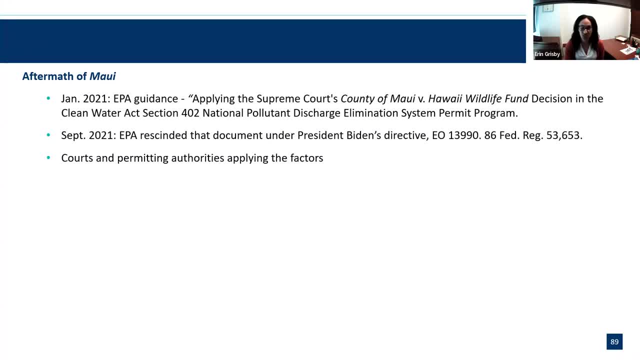 And And. Then, Not too long later, The Biden administration rescinded that document Under his EO 13, nine nine zero. They rescinded the prior guidance because they said the guidance had added an eight factor on the design and performance of the system. 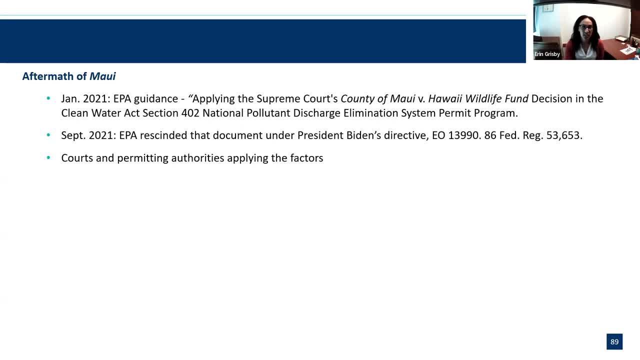 Or facility from which the pollutant was released, And they said that that That additional factor was not consistent with Maui because it added an element of intent. So what you have now, today, are courts and permitting authorities Applying these factors in in practice. 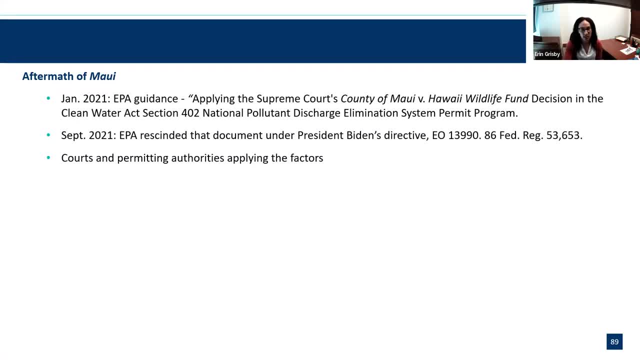 So Since Maui you had- I'll just give a couple of examples- There was a district court in Montana. They actually requested each party brief, Brief them on each of the seven, nine factors and 30 words or less, And then they added an eight factor. 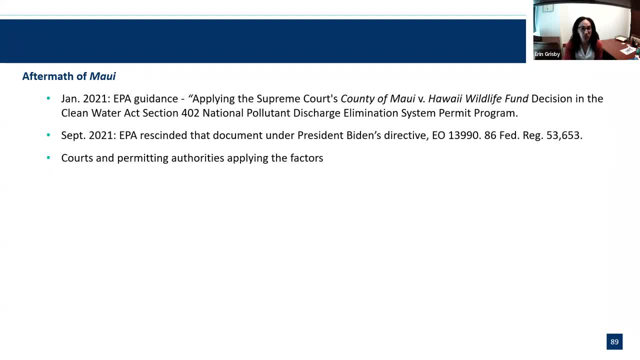 And this eight factor was whether or not there could be some other Contributing source for the pollution That was at issue in that case. You can see here there's. the permitting authorities are having to grapple with this. I think it was a pollution control agency. 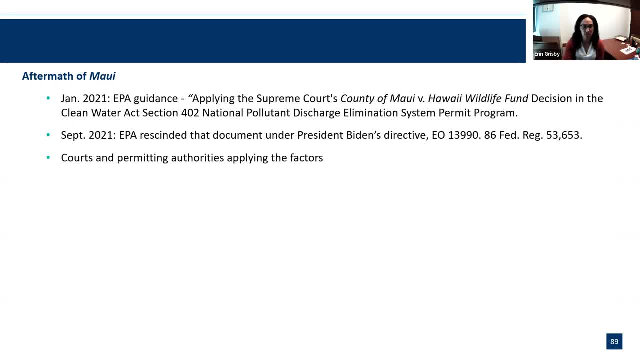 I want to say miss Minnesota in 2000.. I think this may be earlier this year. Based rebound And one of their. they issued a permit and the Minnesota appellate court remanded the print back to them Because they had not considered. 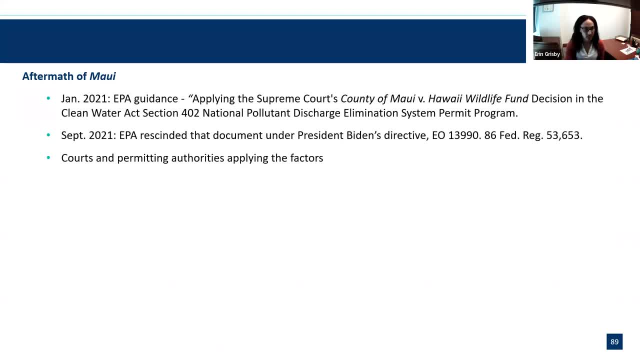 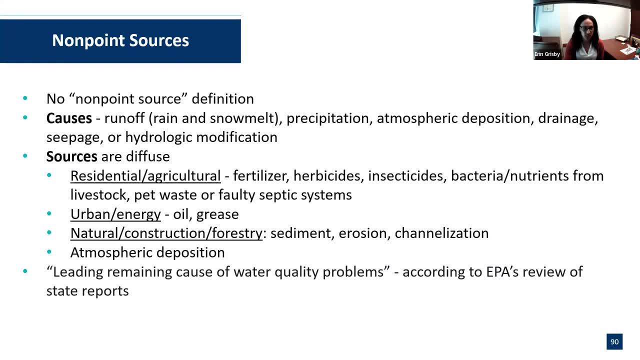 The Maui factors Next slide. So Turning to- so that was kind of the late, you know- developments in point sources. Now turning to nonpoint sources. Nonpoint sources are defined by exclusion, So they mean any other, any source that does not meet the 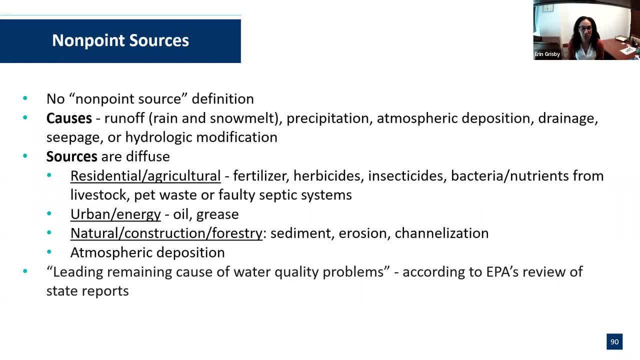 Section five of two, 14, definition of point source. So there is no clean water act. definition of nonpoint source And causes of Nonpoint Pollution are Runoff. That can be from Different types of precipitation: Atmospheric deposition, Drainage, seepage or hydrologic modification. 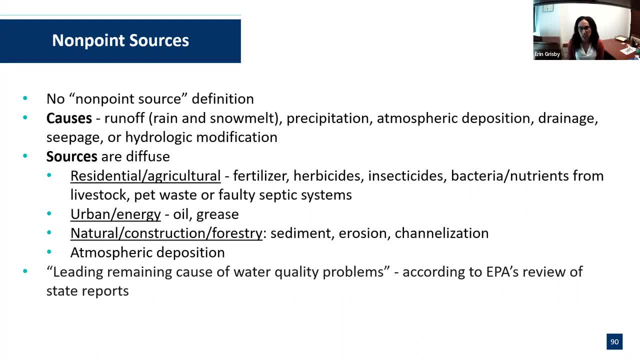 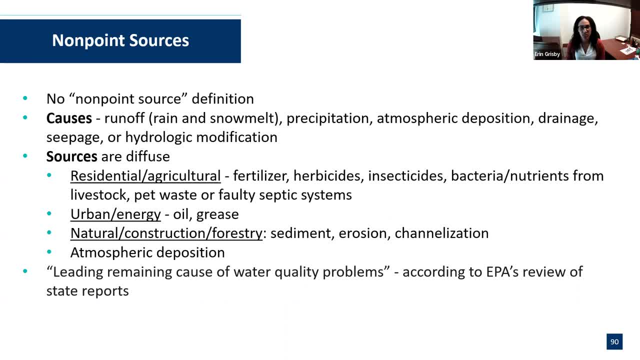 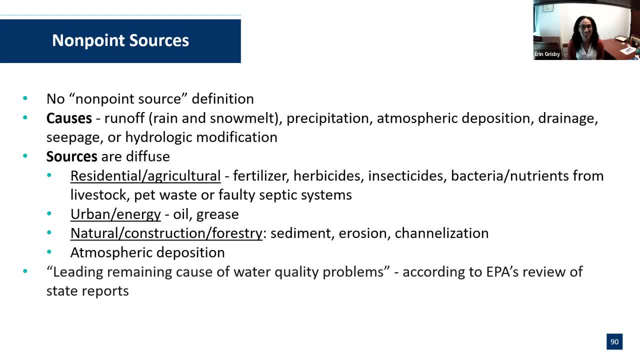 pet waste or faulty sector systems. So you all can help find making sure you're pet waste It goes where it should You have a pet. Then there's also other urban energy like oil and Greece, the type of runoff, The pollution. 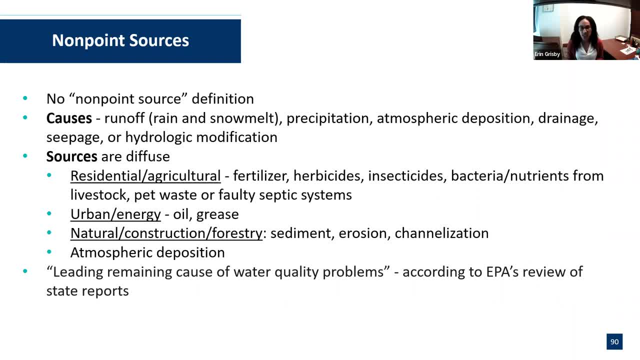 sources would be sediment erosion, channelization and then the atmospheric deposition is air pollutants that deposit back onto the land or the water through precipitation, falling particles or gas absorption. As Robin mentioned, non-point sources are the leading remaining cause of water quality problems according to EPA's review of state reports. So it was section 319 that 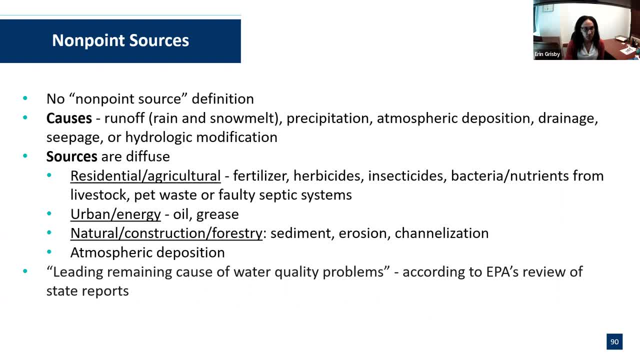 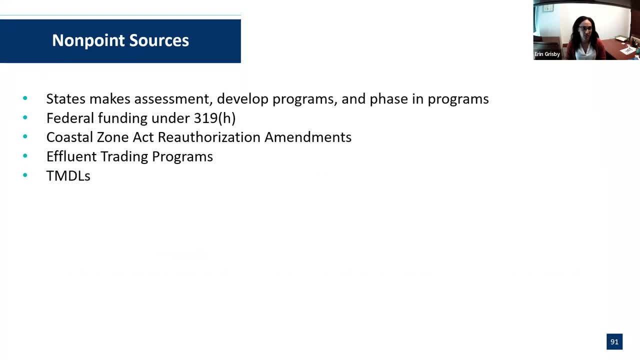 laid out the non-point source management program and we'll talk more about that on the next slide. So under the program, states make certain assessments about their water bodies within their jurisdictions and they develop programs to help manage non-source pollution. Then they 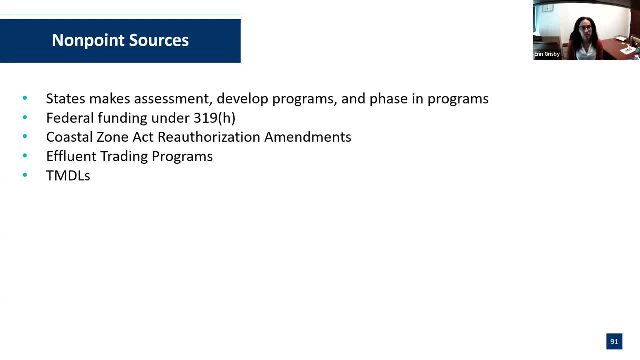 phase in those programs There's federal funding for states under section 319H, and so the states would submit a funding form to the United States and then the state would submit a funding form to the United States and then the state would submit a funding form to the United. 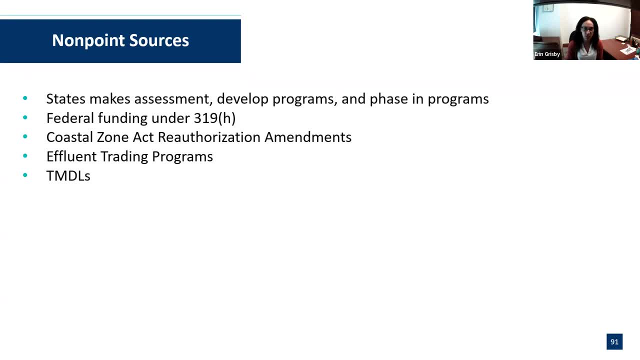 funding plan to EPA. EPA determines if the plan meets the eligibility needs of requirements And then, if so, they go ahead and issue some funding. And the states may be surprised that they can include more than just controls. They can include technical assistance, education, training. 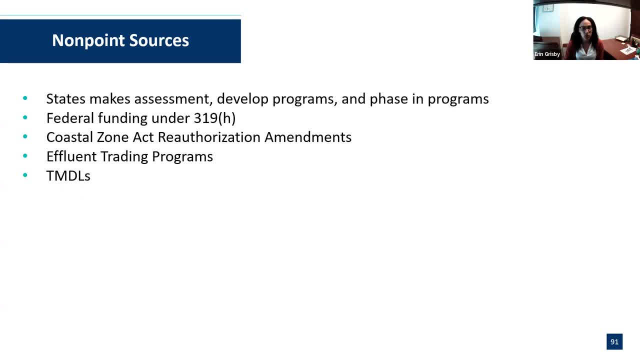 technology transfers, in addition to, you know, their regulatory programs and financial assistance to help get some pollution controls in place. So the Coastal Zone Act Reauthorization Amendments- I believe those were in 1990, established the Coastal Nonpoint Pollution Control Program. that 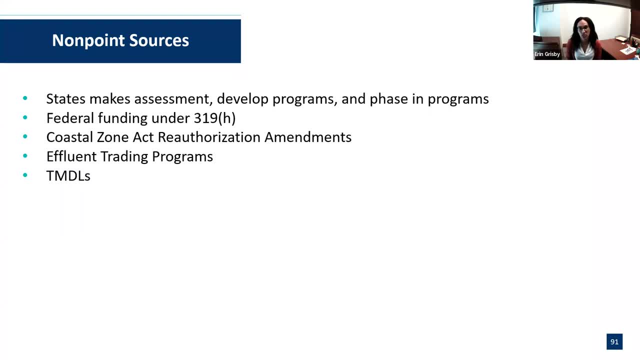 EPA administers with NOAA, That's the National Oceanic and Atmospheric Administration. So that program addresses nonpoint source pollution problems in coastal waters And understandably it's a program that's been used to address nonpoint source pollution problems in coastal waters And understandably it's a program that's been used to address nonpoint source pollution problems in coastal waters. And 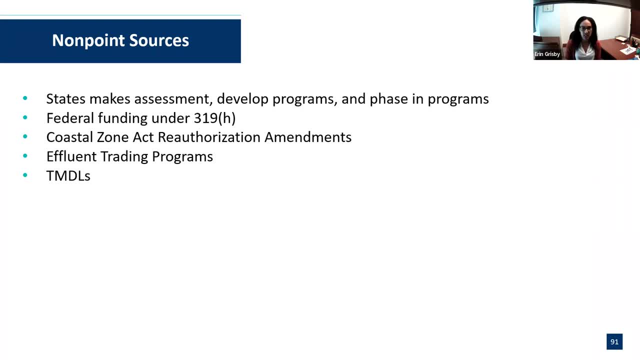 under Section 6217 of that act, states and territories are required to approve coastal zone management programs, to develop coastal nonpoint pollution control programs, And those programs are supposed to include nonpoint source pollution controls. So the states, really, while the federal funds 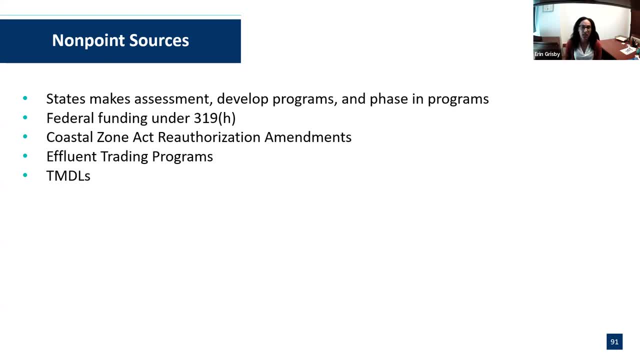 those programs are supposed to include nonpoint source pollution controls. So the states really, while the federal funds this program, federal regulations really applied to federal to point source. So there are kind of- I think Robin mentioned that there's ways to a lot of this- is incentivized: providing money, providing the tools. 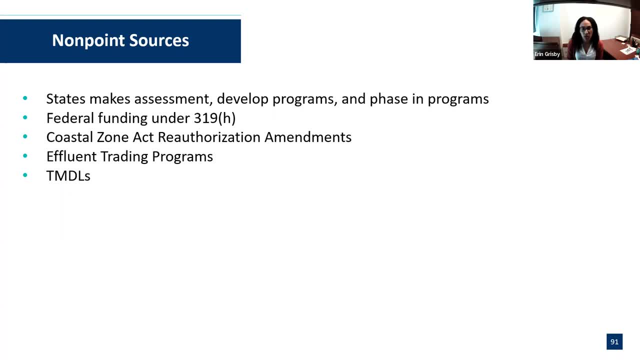 And another way to help get some more additional nonpoint source control is effluent trading programs. So these are similar to, if you think of, carbon trading programs. they allow for commodities to be traded between regulated entities. Here it would allow for commodities to be traded between regulated and non-regulated entities. So under I think some states have 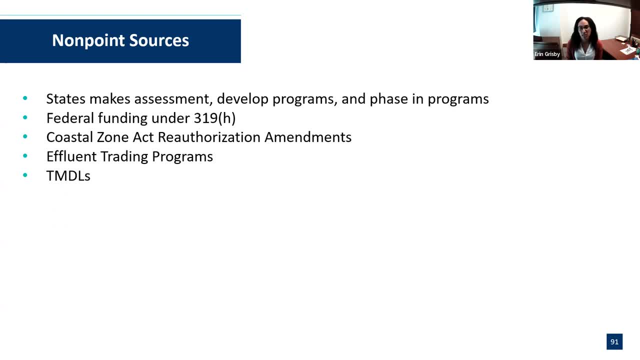 had these programs where the, under the programs, the facilities with the NPDES permanent discharges, they'll be facing higher pollution control costs and they might be able to meet their obligations if they purchased, you know, equivalent pollution reductions from other sources. 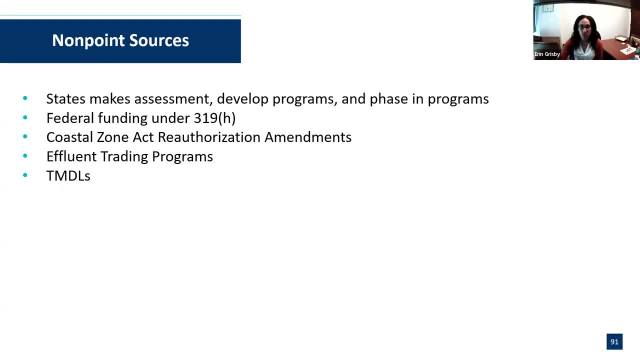 It might be a lower cost to them and that could be a non-point source. So that would then incentivize a non-point source to maybe somehow some way control so they don't need their reductions and they can sell those reductions to the regulated entity. 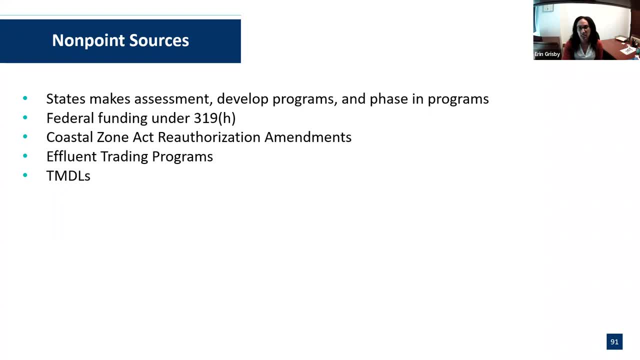 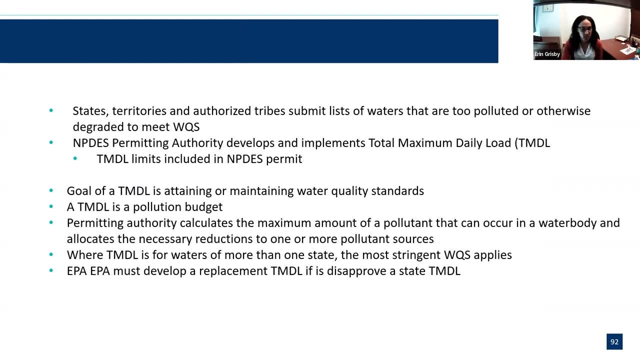 So one way that a regulated and non-regulated entity may seek to trade is with their regards to total maximum daily load- Next slide. So TMDLs apply to impaired waters, States and territories and tribes. authorized tribes submit lists of waters that are too polluted or otherwise degraded to meet water quality standards. 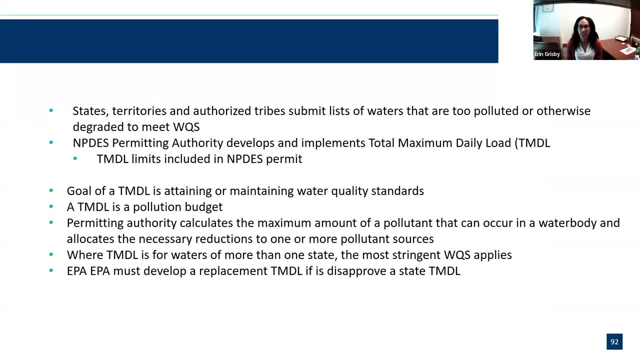 So that's what I spoke about earlier, about these. you know, these standards are based on the designated use anti-degradation policy, and they underlie the water quality based at limit limits within the permits, And so these are known as the 303D impaired waters lists. 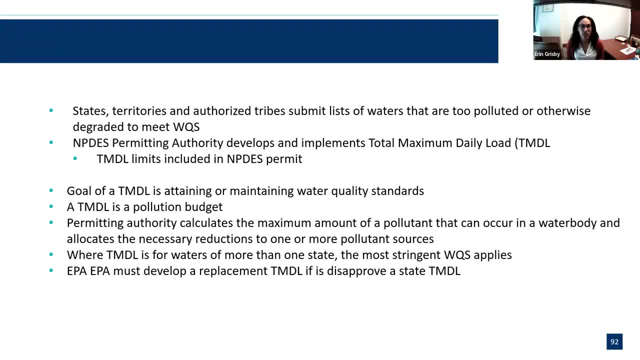 The NPDES permitting authority develops and implements the TMDLs And so, and as you already know, those, the limits are included. The TMDL limits can also be included in the NPDES permit if the water body is impaired and has a TMDL limit established. So the main goal of the TMDLs, 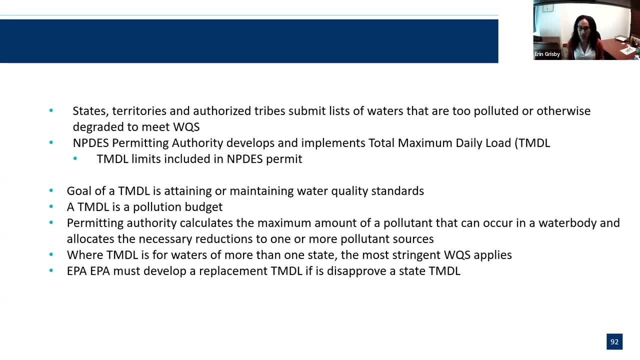 is to attain or maintain water quality standards And it's pretty much a pollution budget, like a lot of our pollution systems. It's the permitting authority, calculates the maximum amount of pollutant that can occur This is in a water body and allocates reductions to one or more. 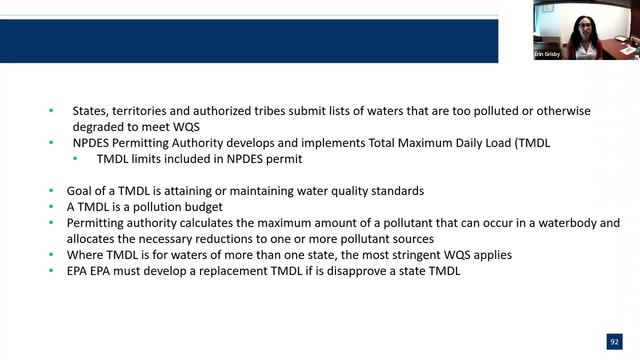 of the sources of pollution to stay safely under that maximum amount. So where there's a TMDL, that is for waters that are for more than one state, the most stringent water quality state water quality standard applies. So if EPA does look at these at the state developed TMDLs and if EPA disapproves a state, 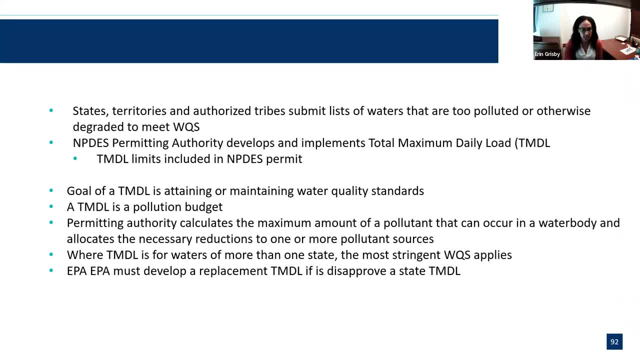 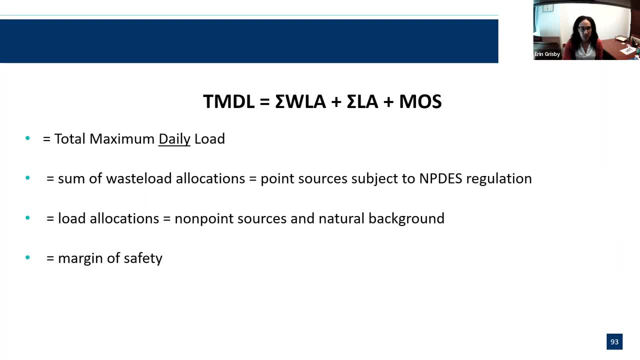 TMDL. EPA must develop a replacement TMDL on its own. And next slide. So here is how the TMDLs are calculated. So the TMDLs are developed for each pollutant, typically So if there's three pollutants impairing a single water body. 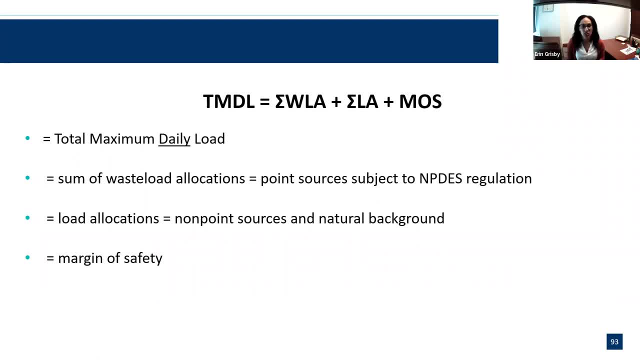 that water body could have three TMDLs. Alternatively, there could be an instance where one TMDL may be able to address multiple pollutants. So, looking at the formula here, so you take the sum of the waste load allocations, So that would be all of the. 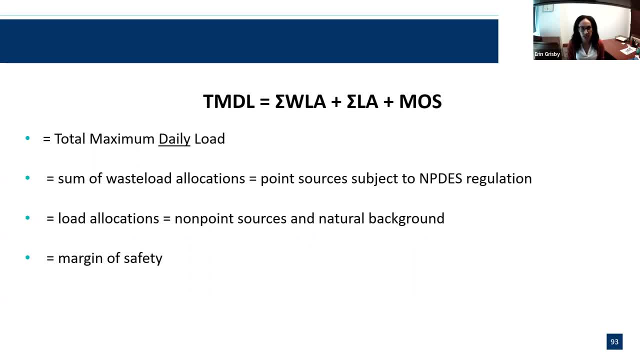 existing point sources subject to NPDES regulation. You add that to the load allocations, which would be all the nonpoint sources and natural background, And then you add a margin of safety So you can take in account for seasonal variations- You should, But the margin of safety itself takes. 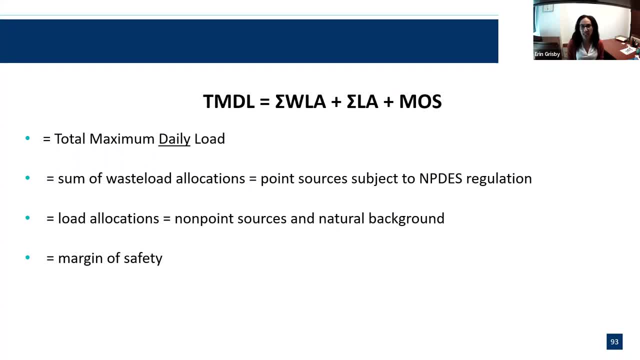 into account any lack of knowledge concerning the relationship between the effluent limitations and the water quality. So sometimes there's a lack of knowledge as to nonpoint source pollution. So there's a margin of safety built into that. I have underlined here daily in the term total maximum daily load. So there's been 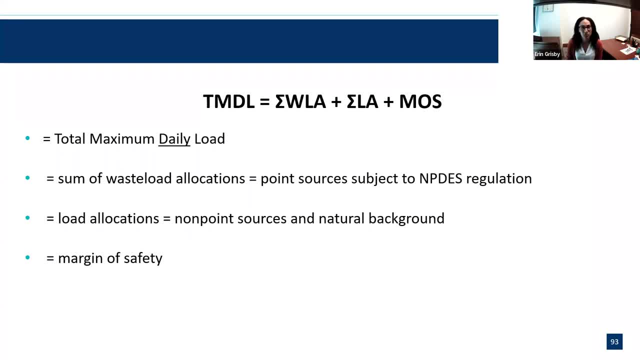 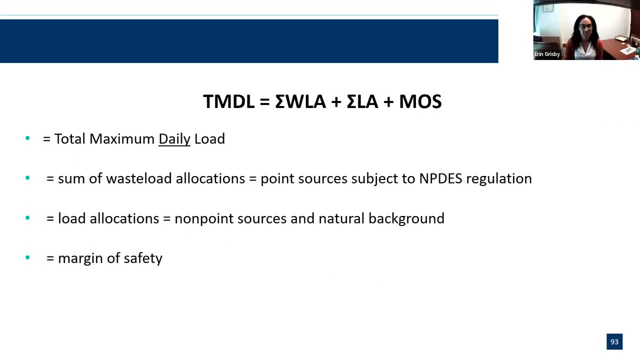 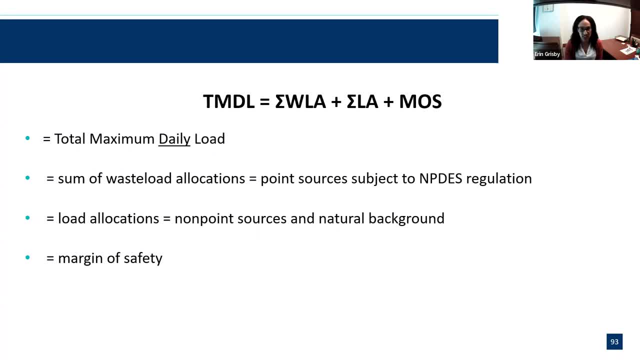 it might not be as transparent as you might initially think And some circuits may have come out a little bit different on that. So that's pretty much all I have for you guys today, And I was not watching to see if there were questions, but I can. 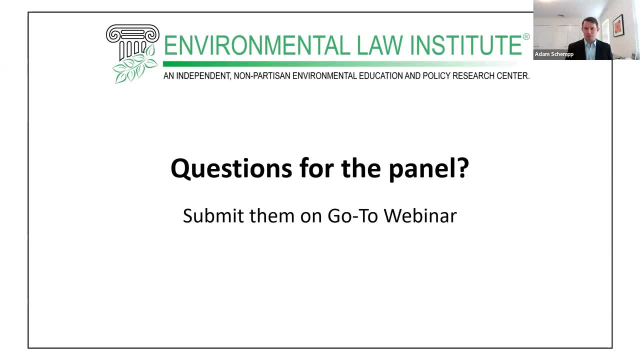 Oh, thank you very much, Erin. Yes, we've had a lot of questions rolling in And with our 20 minutes remaining, we will try to get to as many of them as we possibly can. I'll actually start with Chandler, if you want to explain the availability of the recording for this. 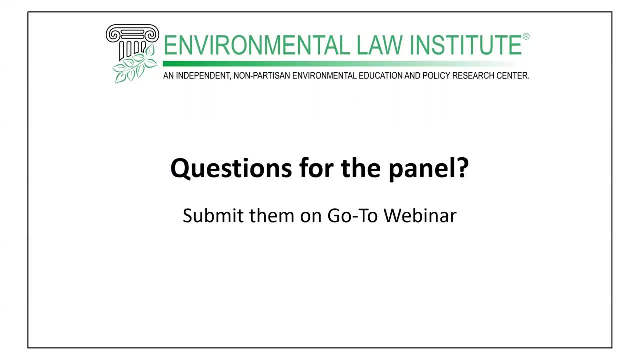 Yes, So the recording will be available online at ELI's website on this event page. So if you're registered, you will have access. I would ask you to fill out the recording and then you can estimate that to be available in about two business days. So check back early next week. 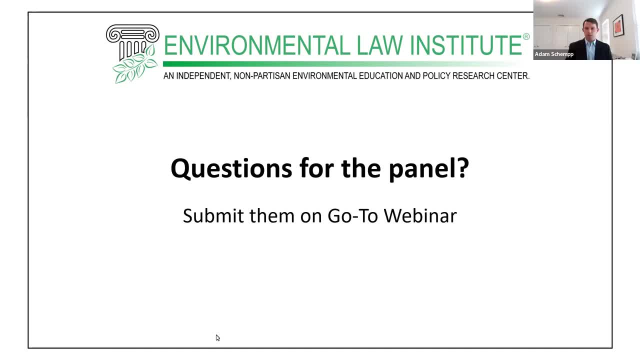 if you're interested in watching the recording, Great, Thank you. So I've actually asked one of my colleagues, Becky Kisslinger, who is the head of ELI's wetlands program, to also join us, because I feel like there are some questions here that she might be able to help with, And I will start with. 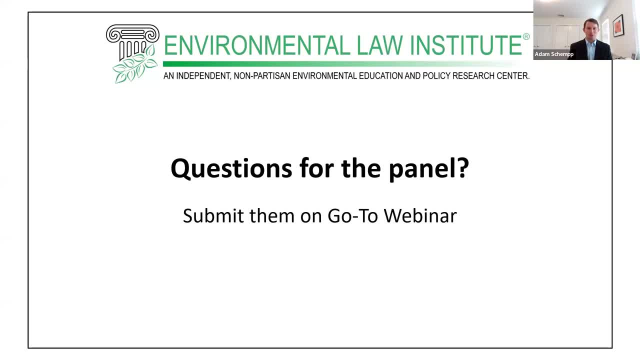 one specifically, And certainly the panel is very welcome to jump in on this as well. But the question is: can you elaborate on what you're talking about? Can you elaborate on what you're talking about? Can you talk a bit about the wetland banking and how that may be done with? 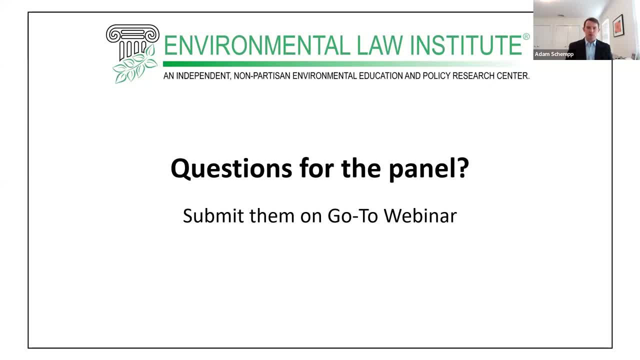 salt marsh areas, for instance. And Becky, are you able to speak? I'm here, Can you hear me? Perfect, Yes, Great, Okay, It's asking me. Well, okay, I'll just go ahead, Thank you, I'm sorry, I. 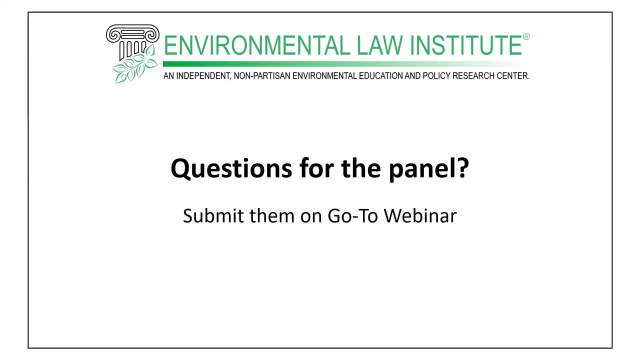 joined a little late. Thank you, Adam, for inviting me. It's a great question And I'm not seeing the presentations. I'm just going to start a little bit at the beginning, but try to go quickly. So wetland mitigation banking is one of the ways that a permittee can satisfy their 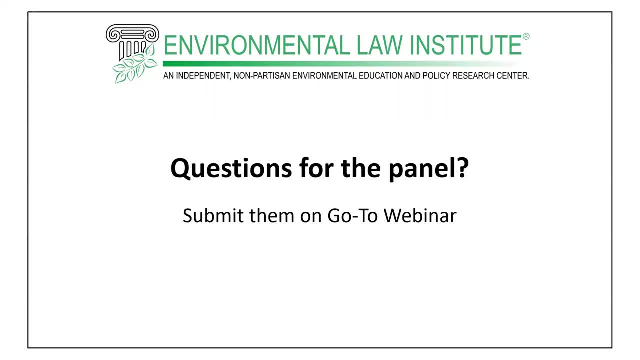 compensatory mitigation requirements under their Section 404 or their state permit for impacts to wetlands and waters. So for a mitigation bank, the banker will enter an agreement with the Army Corps of Engineers and the interagency review team. That agreement is called their banking. 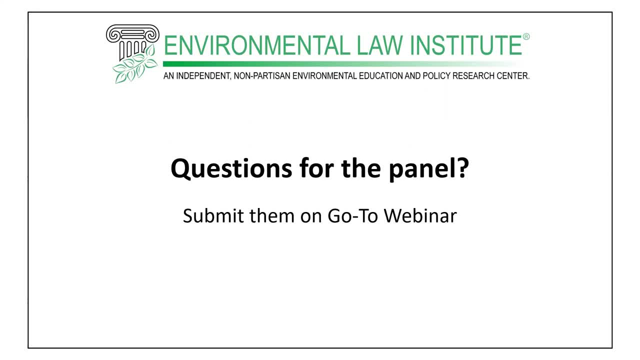 instrument And that lays out their plan for restoring, enhancing and sometimes preserving a wetland, That for which they will then be able to sell credits to permittees for their compensatory mitigation requirements. So once the banker has met the laid out requirements in their 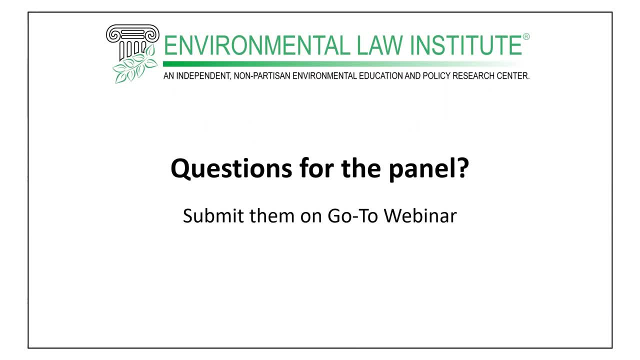 instrument. they are allowed to sell those credits to permittees And those credits are based on the kinds of resources that they are restoring. So that could be a stream, non-tidal wetland, a salt marsh wetland, and then the functional lift that they're providing through the restoration. 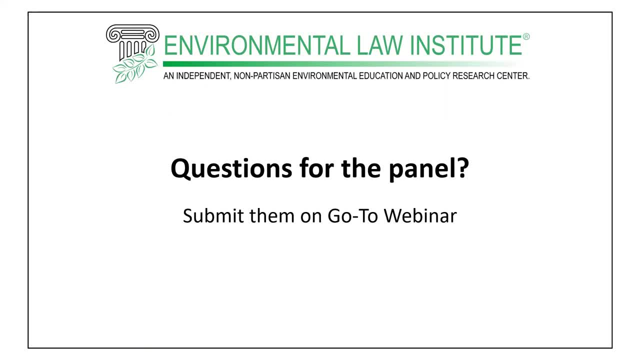 So those credits can be, and so your question was specifically about salt marsh. So they can. a banker could restore a site, a salt marsh site, and provide salt marsh restoration credits on the market for impacts to other salt marsh wetland areas. 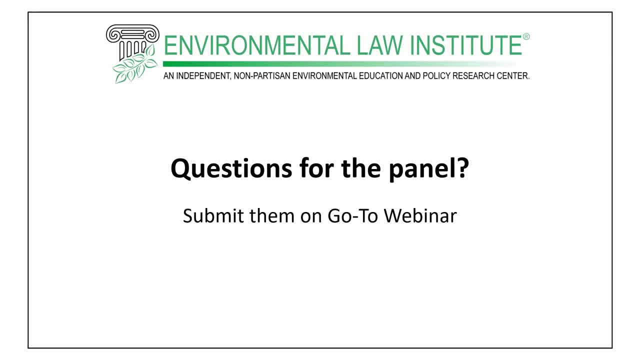 I did a quick after Adam wrote me. I did a quick look at the US Army Corps' Ribbit site which catalogs all the different banking sites and what kinds of credits they have, And there were a number of salt marsh mitigation benefits And I think that's a good way to start. 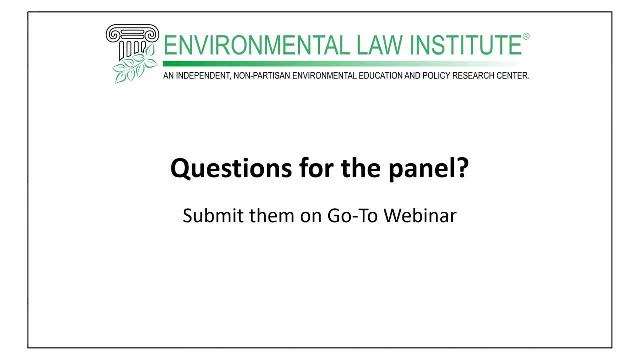 Thanks. So they do. there are. they are out there and there may be more than I was able to pull up, but those would be opportunities for, you know, a restoration area that would be funded through the sale of compensatory mitigation requirements to offset impacts to those sites. 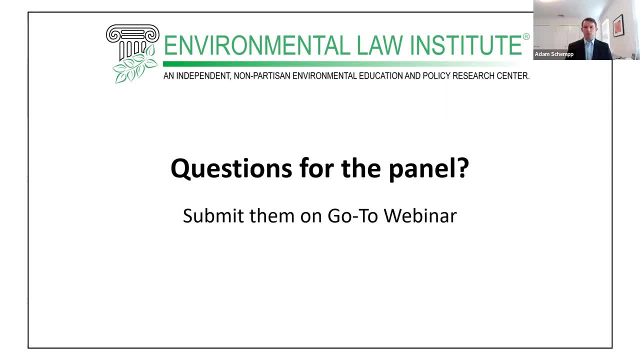 Adam, do you want me to expand on anything, or does that sound? I'm actually wondering if you can. if you're able to send me the Ribbit's URL, I'll put that in the chat. Awesome, Does anybody on the panel want to expand on that? Any other, any comments in that regard? 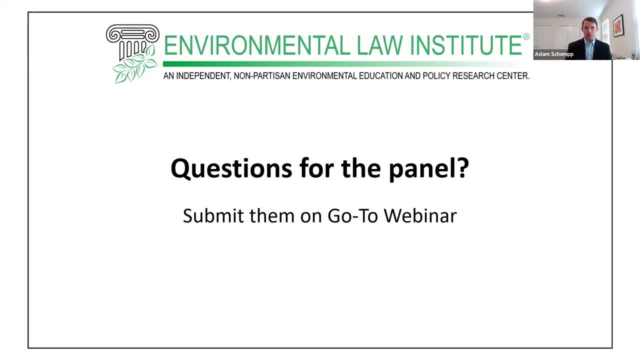 Okay, We'll go to another one that is related, while I've got you, Becky, How effective are these? wetland banking and also the questions about effluent trading programs- how effective have they been- examples and opinions, And so I'll start with wetland banking and then we'll 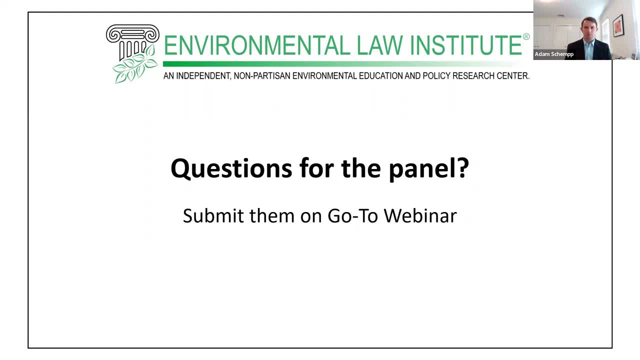 move on to effluent trading. Sure, That's a complex question. So I think historically there was some concerns about the ecological success of compensatory mitigation in general and mitigation banks specifically, And then, in 2008,, the Army Corps of Engineers and EPA. 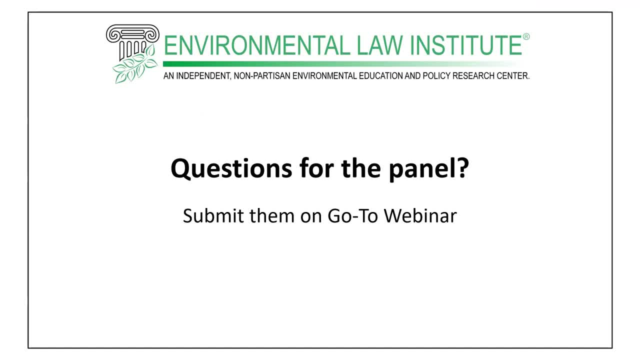 finalized regulations to try to improve the administration and implementation of all forms of compensatory mitigation, And so that required that there were financial assurances to ensure that the compensatory mitigation projects were actually occurred and met their performance standards. They have requirements for monitoring and long-term management, and 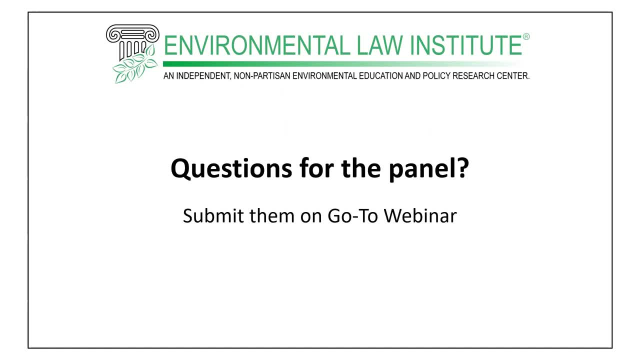 adaptive management and that was meant to really improve the practice. There haven't been a lot of good, comprehensive nationwide studies since those rules were finalized more than 10 years ago, coming on 15 years ago, But I think that practice has certainly improved and there's 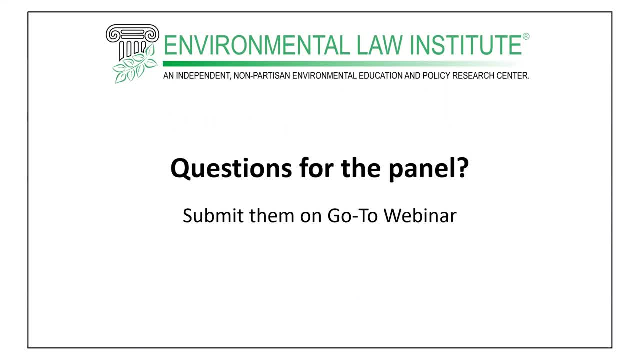 more studies showing that at least administration of mitigation banks and in the fee programs are following the requirements and the regulations. But with regard to the ecological success, I think that more study is needed to show how those sites are faring on the landscape, And the restoration of these kinds of systems is very complex and 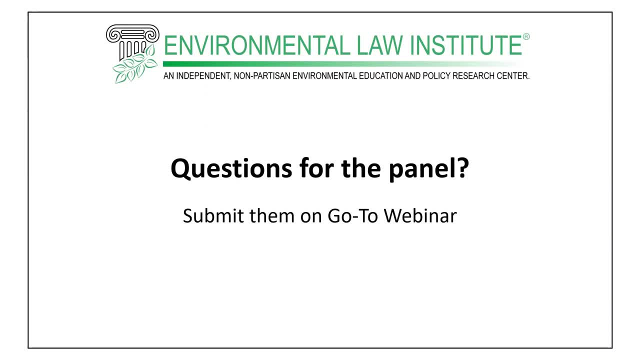 takes a long time to get to where you can see actually how they're going to function over time. So we're just getting to a point where I think those studies would be extremely valuable. Thank you, And thank you for being with us, Becky. 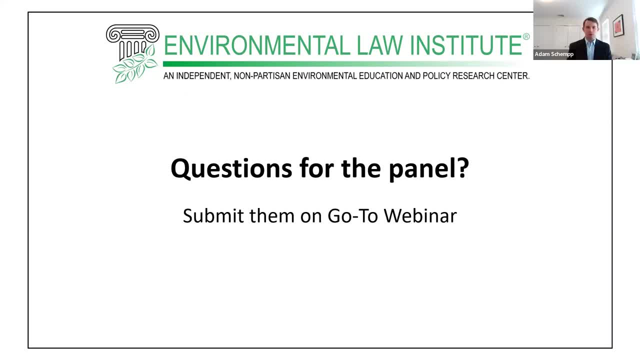 Sure, Looking to the panel with regard to effluent trading programs, whether Aaron or anybody else has a question, please feel free to ask. Would anybody like to comment on how effective they have been? I actually don't know how effective they have been, but I do know that there have been. 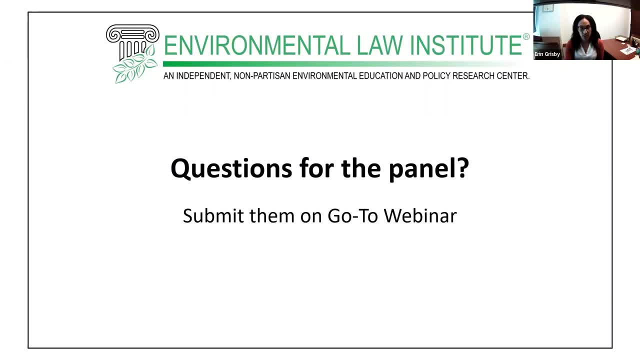 I think, government evaluations and as well as private evaluations that can likely be found online to find out a little bit more. The EPA is still, I guess, supporting those. They have issued some resources, guidance documents and some other things, So I think that's a good point. 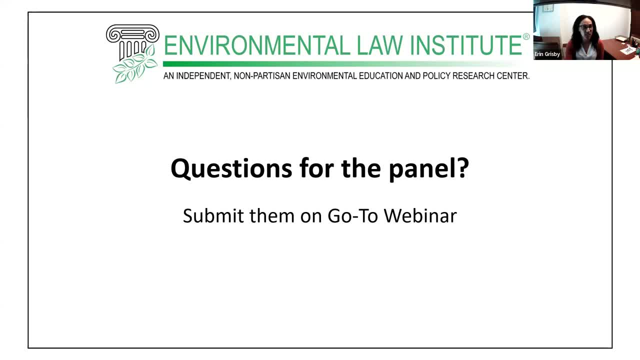 And I know that the EPA, or the EPA that has written on the research finance documents, frequently ask questions and things of that nature. So in my mind there's still a tool that at least the agency thinks is useful. I could piggyback on that And I'll say this is not my area of expertise, But I could just 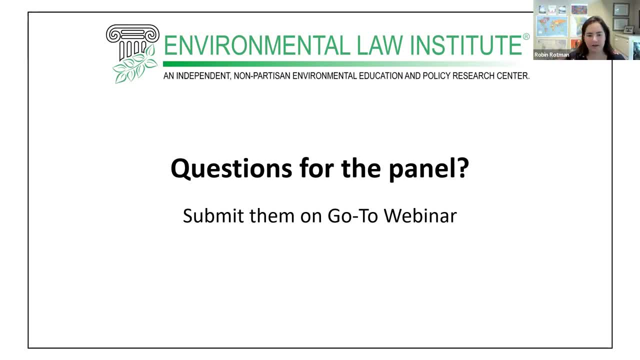 make a couple general points, which is so. the Clean Water Act, as Aaron said, allows for water quality trading. We also see this, for example, on the stuff that we have on the channel, and they have some lot of information regarding what we're doing And they don't. 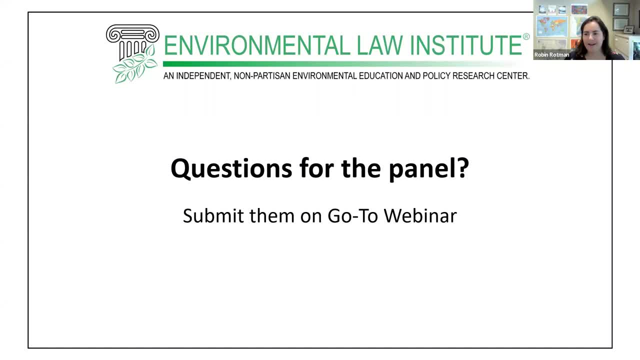 always have it in the table. But you know, I think they have to be doing it right And I think that's really important. And I think it's really important for the agency to hit the example under the Clean Air Act. And I think two issues that are challenging under the Clean Water Act is: one is the fungibility. 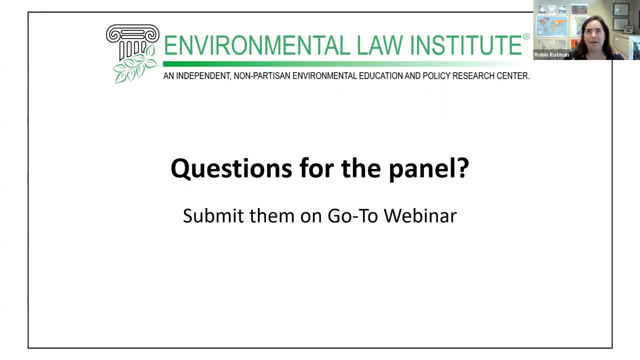 of discharges. So a certain amount of pollutants discharged in one location does not have the same effect on the environment as it being discharged in a different location. So there needs to be a sort of scaling in order to preserve watershed quality. that is technically difficult to achieve. 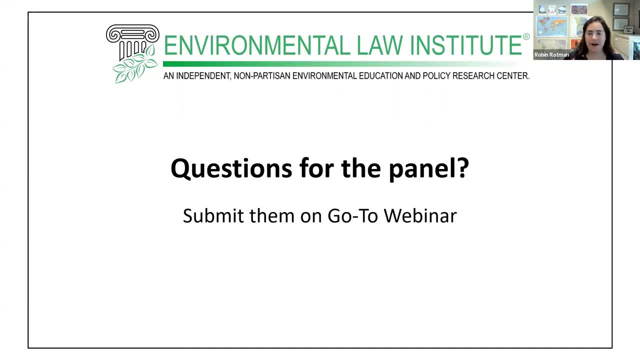 Another point that is relevant not just in the Clean Water Act, but we could also see this in some areas of the Clean Air Act, which is an environmental justice focus, which is that, if you allow trading, there could be the concentration of pollution hotspots. 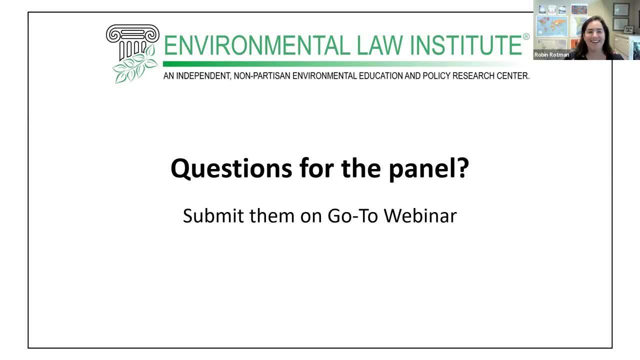 And perhaps if we think about like carbon emissions or carbon trading or greenhouse gases, you know, there it sort of doesn't matter where the carbon is emitted, because it's sort of the same thing, It's not having a negative impact right in that immediate vicinity of emission. but 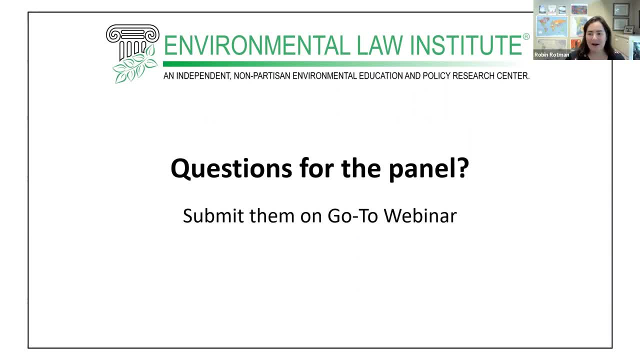 it's having a global impact on climate change, But for water or other forms of air pollution, that is degrading environmental quality in the immediate vicinity of the discharge, And so even if you could work something out that was mathematically correct and kind of- 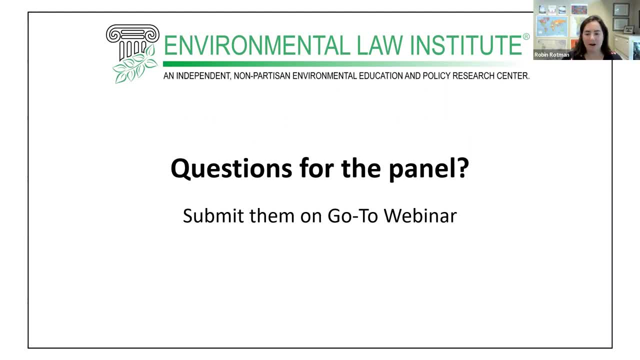 leading to overall maintenance or improvement of water quality. that doesn't mean that, with all of the things that we've been talking about, we're not going to be able to do that, And so I think it's important to think about how we're going to be able to do that, and 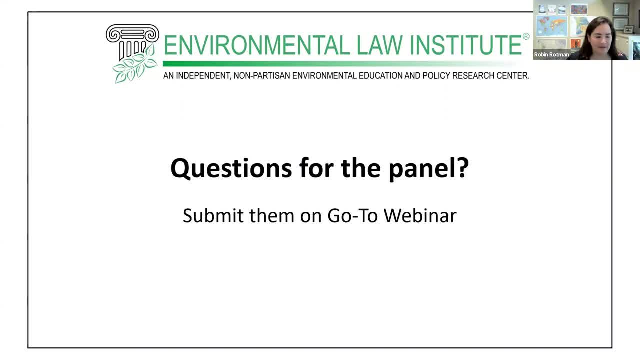 how we're going to be able to do that within each location in the watershed or each population living in the watershed wouldn't necessarily benefit from a water quality trading. And, Neil, this is also not my area of expertise, but I will say, since the question I was asking, 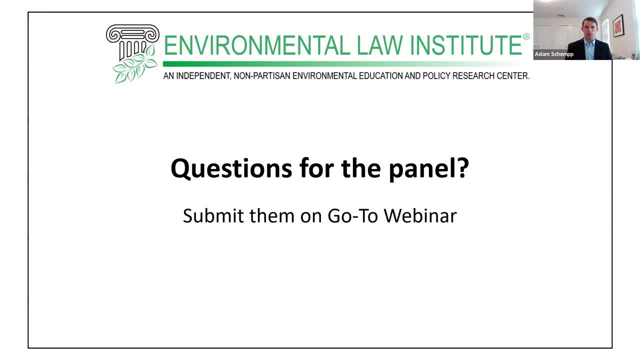 for examples. I feel like most of the examples to date have concerned temperature impairments and that particularly looking at Oregon. OK, trying to get to some of the other questions, Are forest roads and forestry activities only covered by NEPA? They appear to be excluded from the Clean Water Act. 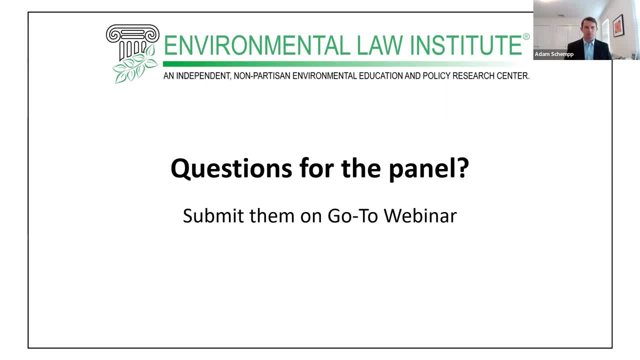 Any answer to that? Well, the Clean Water Act is dealing with discharges of pollution to navigable waters. If we think about the 404 permitting, there are some exemptions for forestry activities, But I guess beyond that I don't fully understand the question. 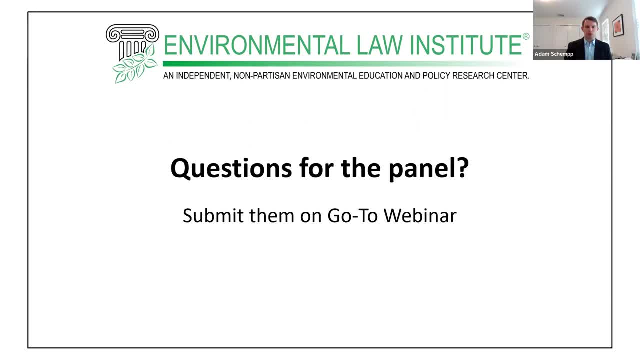 I think it's asking what exemptions there are to forestry activities under the Clean Water Act. Well and so those are mostly related, though, not to road construction within national forest lands, but ancillary, to various silviculture activities. Some debris could end up in a waterway. 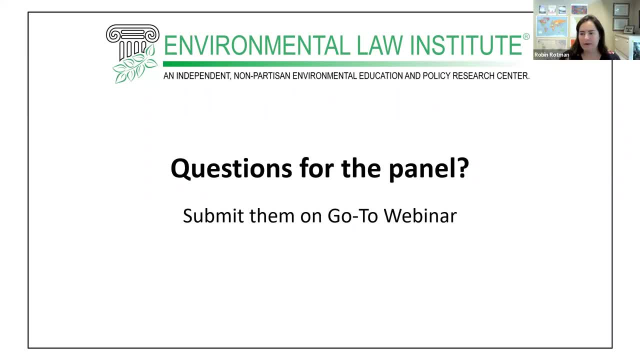 And if that is at a diminished level, then that's not a good thing. But if it is at a diminished or like up to a minimal amount that does not require a permit from the Army Corps of Engineers, I'm not sure if I'm responding to the question. 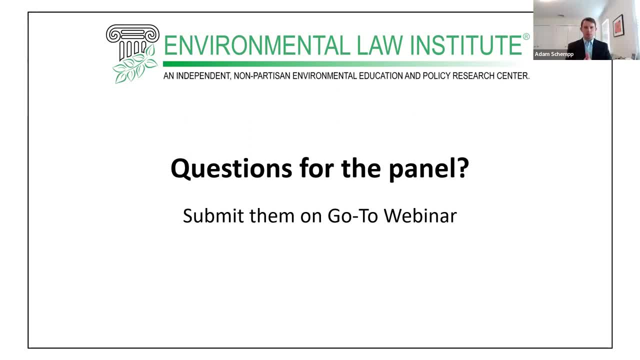 I think that helps. Any other comments on that one? OK, Assuming NEPA applies to the EPA-established effluent limits- the EPA-established effluent limits, how does the economically achievable criteria balance with the other criteria of of NEPA, which also includes economic feasibility? 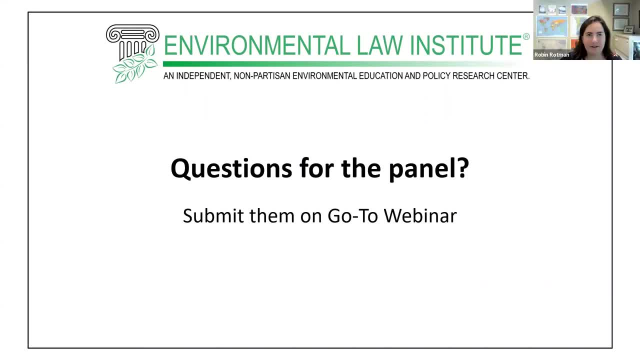 Well, I feel like I'm talking a lot. I'm gonna say this and then I'll be quiet. Okay, so NEPA applies to major federal actions that could impact the environment. However, there are some exclusions under NEPA, and one exclusion is for activities that the EPA conducts. 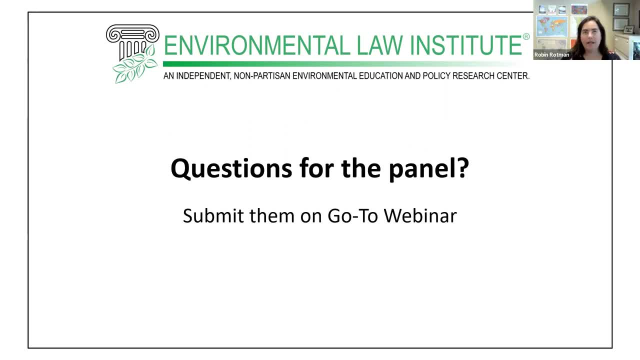 under different environmental statutes, And so the EPA's setting of effluent limitations under the Clean Water Act is not an activity that is subject to NEPA review, because the idea is well, it's already happening under the Clean Water Act, the Clean Water Act and the Administrative Procedure Act. 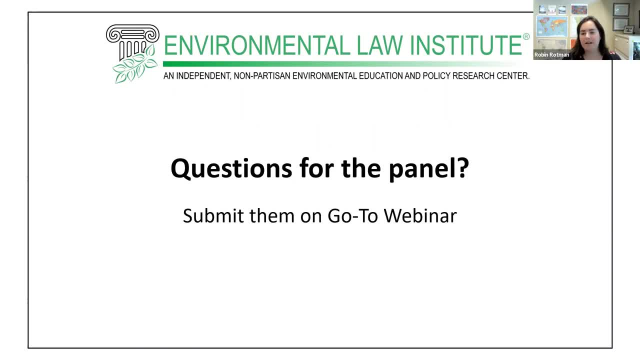 allow for the public to provide comments on that proceeding, And so it's outside the scope of NEPA entirely. Any other comments on that Anyone? I was curious about this, So I was looking it up in between, And one thing I came across was that the Clean Water Act. 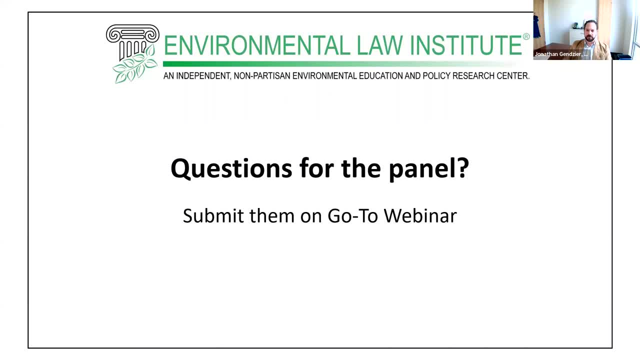 sets out that NEPA only applies to, I think, EPA-issued NPDES permits for new sources. So fairly narrow there. Excellent. Thank you for the on-the-spot research And actually, Jonathan, while I've got you going back to the question, that I had been mistyped- 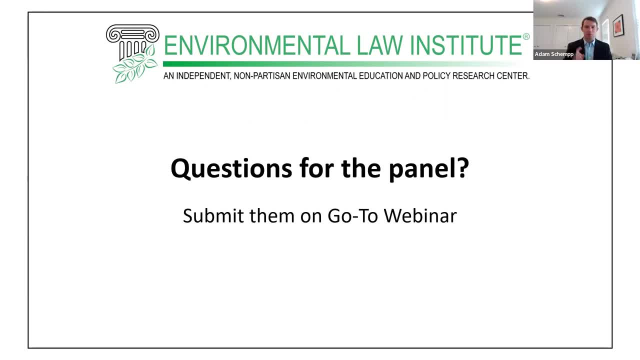 does the proposed Clean Water Act regulation include discussions on playa wetlands, particularly those found in the arid Southwest? I think this goes back to WOTUS rule. So yes, it does. I think it's important to remember that under the Navigable Waters Protection Rule. 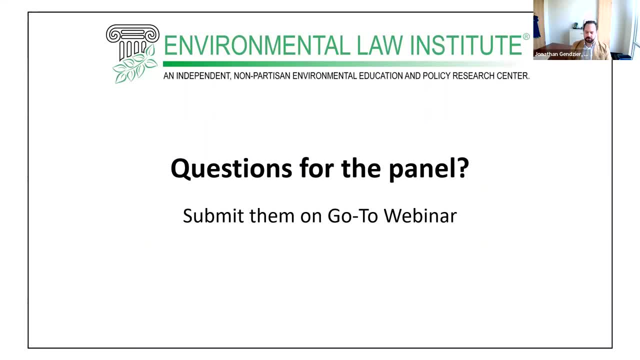 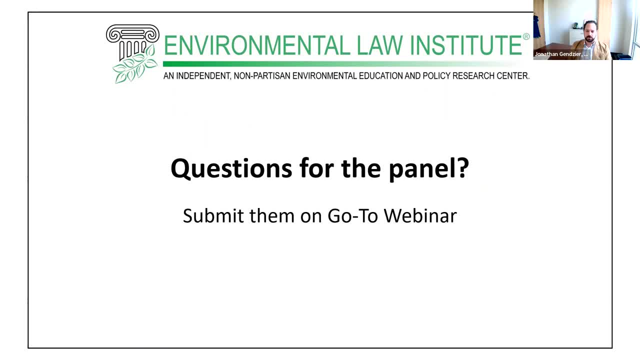 would lose protections, And I think you know there are similar losses for wetlands in the arid West as well. I took a look back at the actual proposal that EPA came out with, And so it includes- it specifies playa lakes as an example of waters. 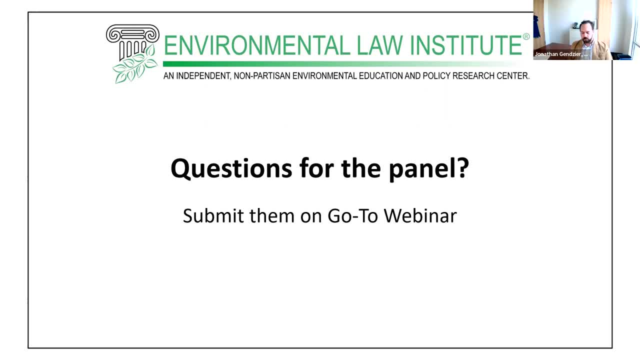 And there's kind of two ways they could come into jurisdiction. One is where the use or degradation or destruction could affect interstate or foreign commerce, And the other is where there is a permanent water body, a continuous surface connection to another jurisdictional water. 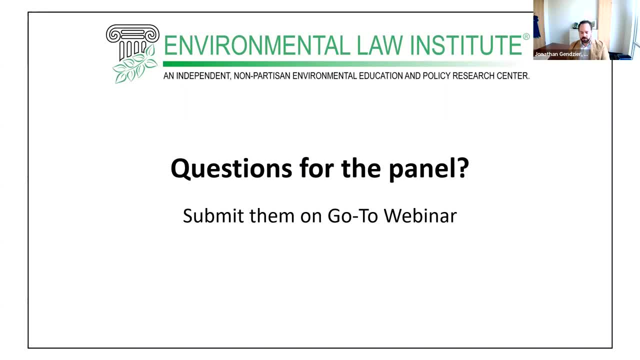 or where alone or in combination with similarly situated waters, they have a significant effect on the integrity of jurisdictional waters. And also, just turning back to that earlier question about similarly situated, I don't think Kennedy gets in the details of what that means. 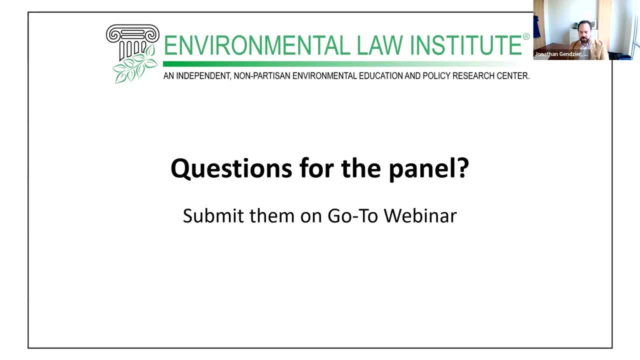 The Post-Riponis Agency guidance from EPA sets out one example where they say: all wetlands that are adjacent to the same tributary are considered to be similarly situated and they point to the integral ecological relationship between a tributary and its adjacent wetlands. 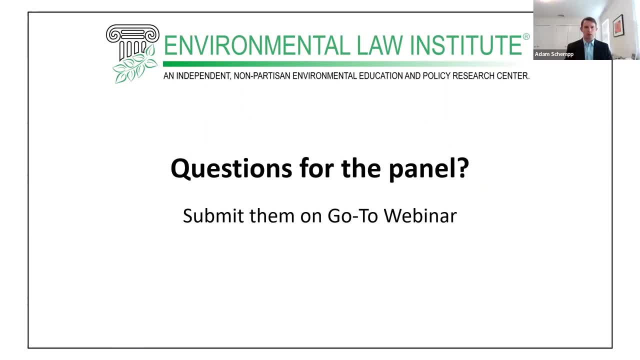 Excellent, Thank you. Any other comments on that one? So I had a bevy of citizen suit questions come through. One of them was: can a state agency action preempt or prohibit? – no, this is the one I wanted to ask. Here we go. 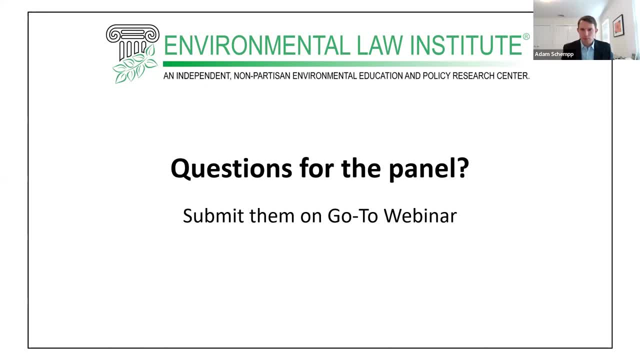 All right, Can a state intervene in a citizen suit at all? That's the first one I wanted to ask. Okay, And what happens to pending citizen suits when that happens? Yes, I mean that – and I welcome the other panelists to jump in, but I think this is known as overfiling. 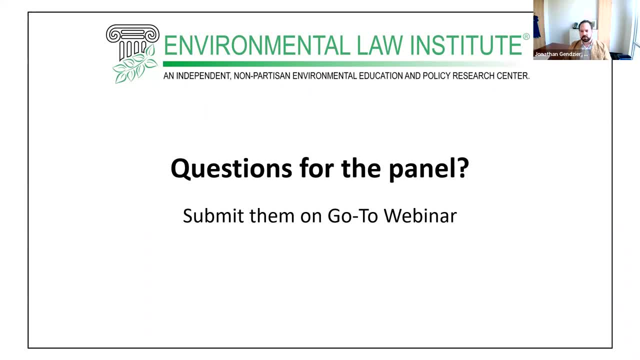 and so you have to send a notice of intent to sue 60 days before actually filing suit in a citizen enforcement, so that gives the state the opportunity to, quote-unquote, overfile or file their own enforcement suit. You know, I think, alternatively, the state could attempt to intervene in an ongoing and 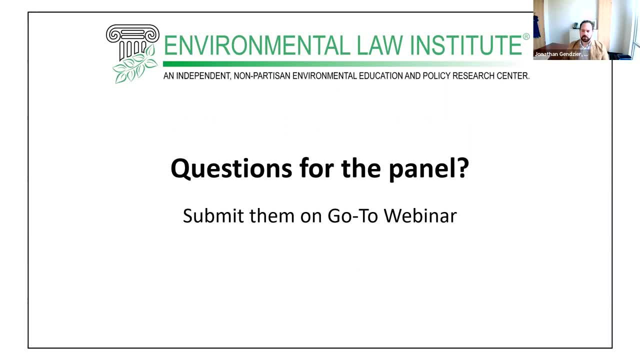 active citizen enforcement suit after the complaint had been filed. The question asked if, when a state agency is a named defendant in the citizen suit, how can the agency intervene. So I mean I think there would already be a participant in the suit by being a named. 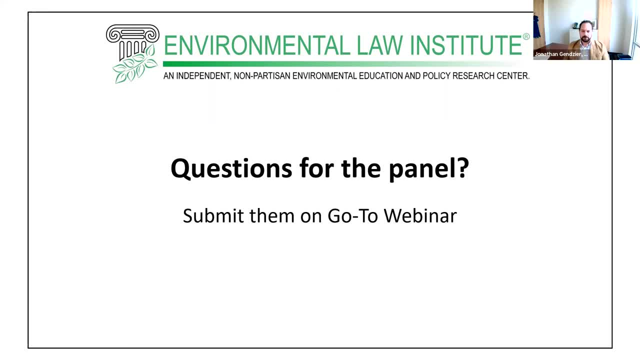 defendant: Yeah, Any other comments on that one? No, Okay, Thank you All right. Going back to one of our earlier questions – and I appreciate, Raymond, your addition in here and I just want to flag it for everybody – there's a note that Section 404 requires. 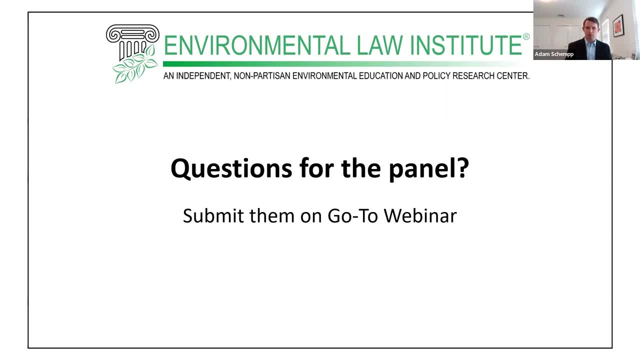 the Corps of Engineers to comply with NEPA before issuing permits, while Section 402,, which is administered just by EPA, does not. 402, definitely some states have designated authority under 402, but most do, Anyway. so I wanted to get – let's see. 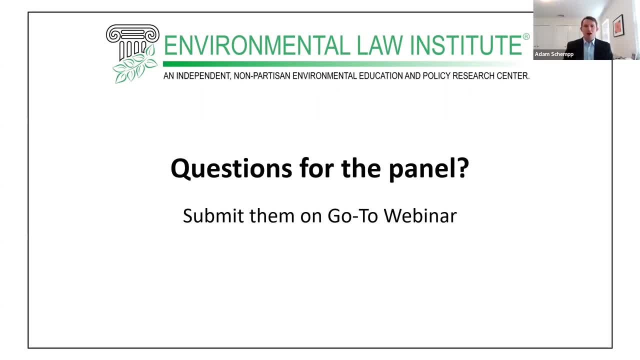 You got it Okay. We've got about four minutes left. Is there any desire to work with FEMA's NPHIP program, N-F-I-P, to ensure that floodplain development does not result in increased TMDLs, especially adjacent to impaired waters? 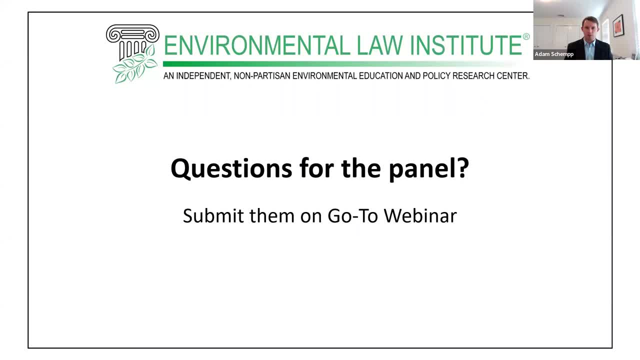 Understanding this should be done at the state level, but is there an effort at the federal level to assist in the coordination, as water quality and floodplain development are not always in the same state offices? Robin, I'm particularly looking at you, but anybody can answer. 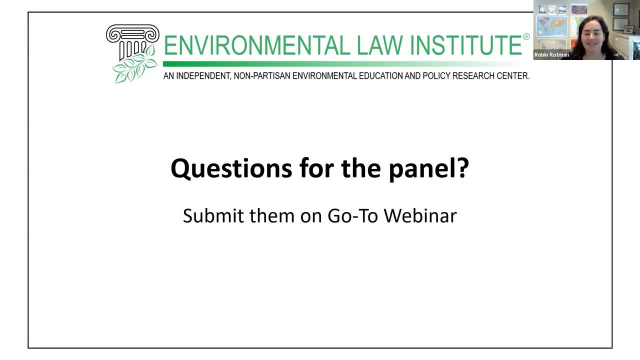 Well, I think – I don't know if I have anything useful to say other than this is a very insightful comment. So the NPHIP is the National Flood Insurance Program, primarily relating to nationally subsidized flood insurance for development occurring in floodplains. 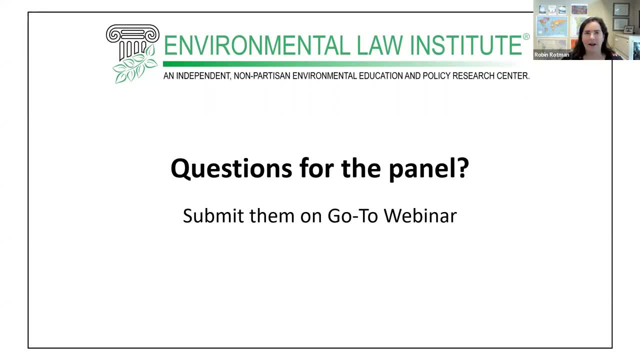 And we could have a long conversation about whether it actually encourages development in floodplains or not. But I am not aware of an activity that is linking the NPHIP and TMDLs. but I think this is a brilliant idea. Maybe can I punt to Erin. 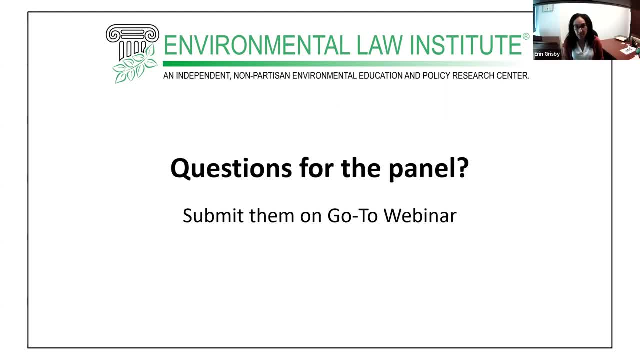 Yeah, I'd have to say I'm not fully aware, but I do know there is a lot of coordination with FEMA and EPA. We even deploy with FEMA as part of our – we can do deployment details with FEMA and even colleagues have gone to work with FEMA at the time for years. 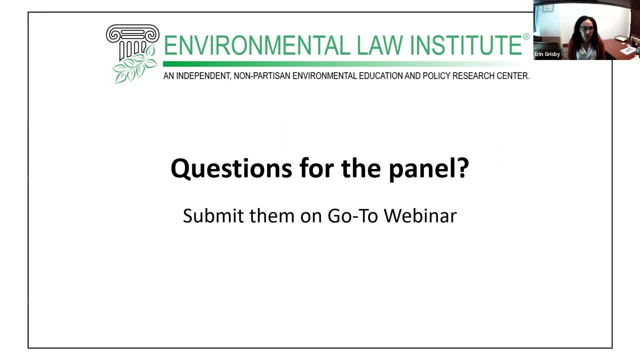 So there is coordination. I don't know specifically on this point, but I would – I'm trying to – yeah, I guess that's all I really have to say about it. It's definitely not my area of expertise, but there may be something there. 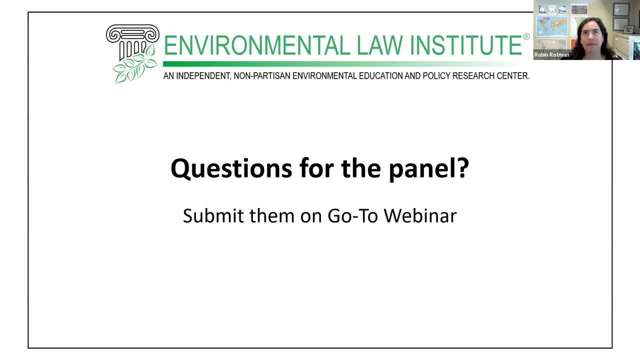 We could make a broad point, which is that – we're often talking about the conversion of agricultural land into urban development, and it is not a foregone conclusion that that transition is bad news from the standpoint of, say, nutrient loading, which could be covered by a TMDL. 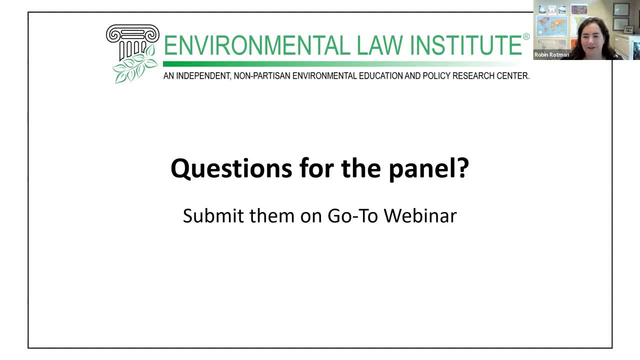 We could talk more generally about urban sprawl or where we should encourage growth, but in fact urban development may really – really be a problem And that can result in a reduction of nutrient loading and support the TMDL objectives. And I'll also add – it's funny, this comment comes up, this question comes up, but ELI is.